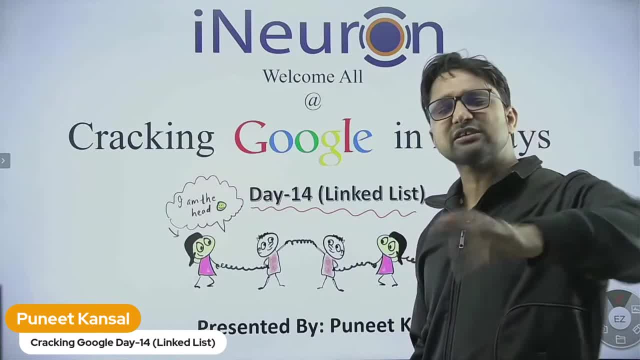 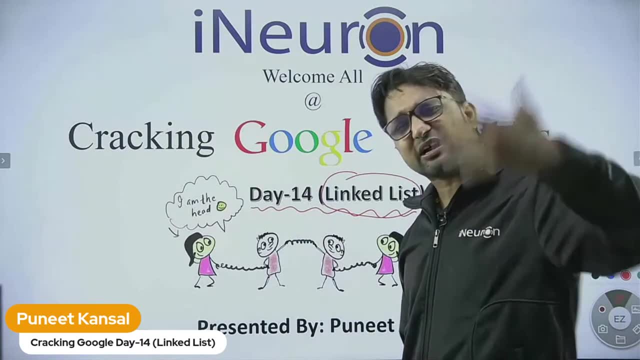 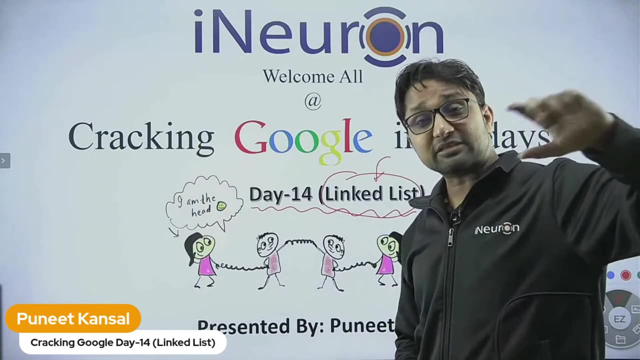 series. but don't need to worry. if this is your first class, don't need to worry, Just attend this class. There is no prerequisite for this class. you just come attend this class and understand the linked list And we will solve a Google problem. Understand that and you can go just simply. 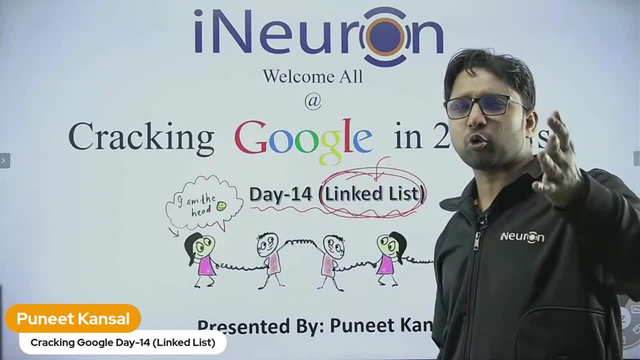 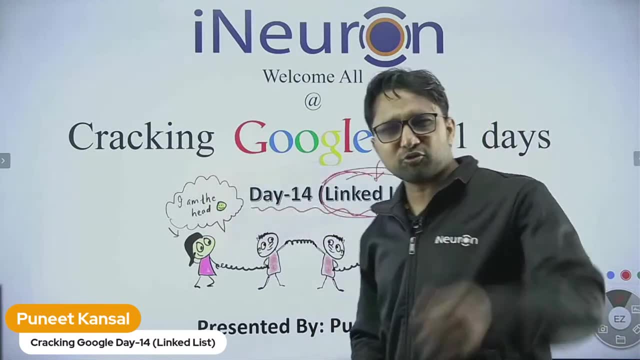 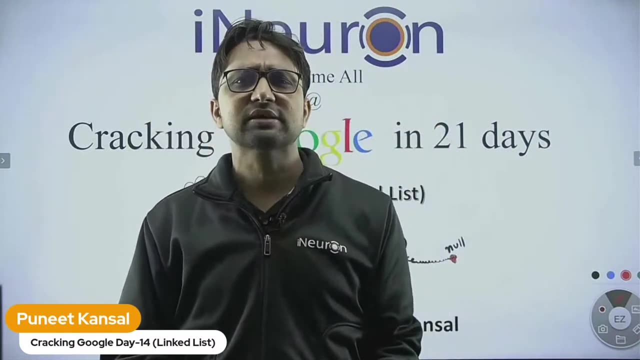 enjoy this lecture independently, don't need to know anything. And if you want to check the previous lectures, then go to the description. go to the description. There is the link is given for this complete course. you can register for this course And if you will complete the course you will also get certificate. This course is free. 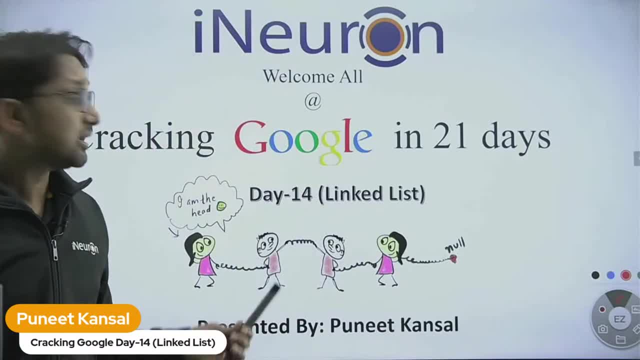 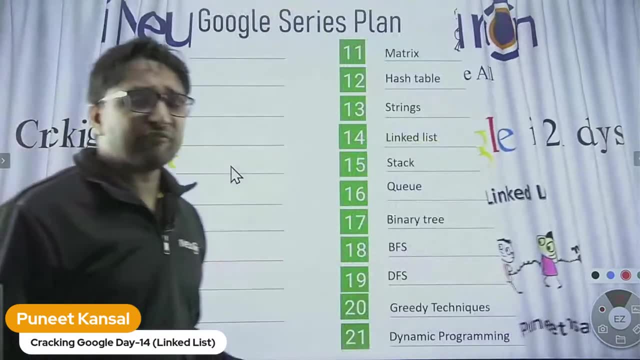 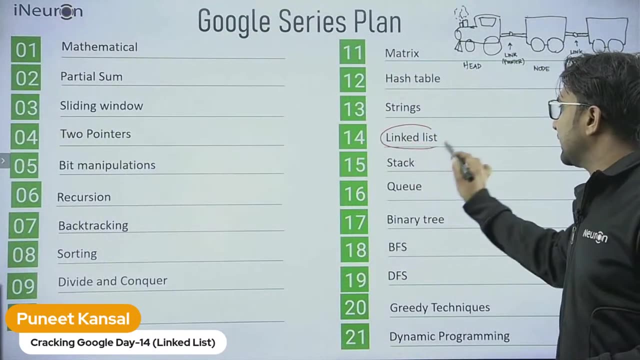 of course- And we are, believe me, this is in this course- we are covering the Google problems, which are which are really interesting problems. So definitely that will help you to improve. And let me tell you, today we are covering the link list, which is the 14th day, and we 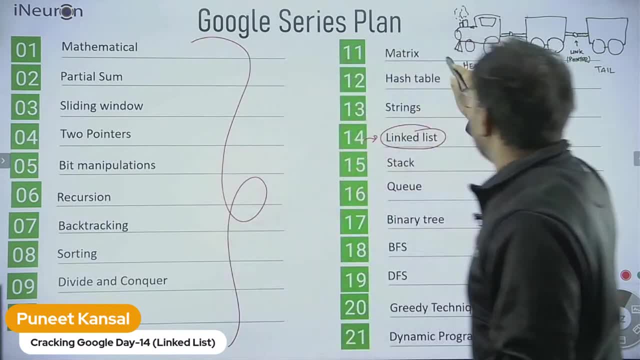 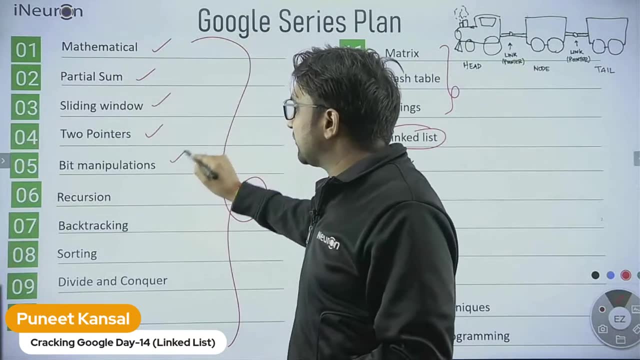 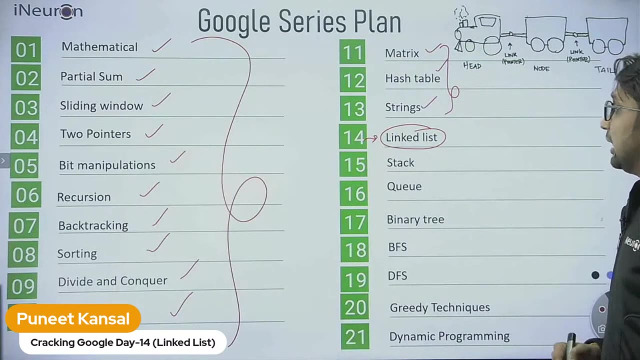 have already covered all these topics By today. we have already covered all these topics. taking google problems, we have already covered. mathematical problem, partial sum, sliding window, two pointer bit manipulation, recursion, backtracking, sorting, divide and concourse, binary search, matrix, hash table string- already we have covered. you can go to the description and you can check out all. 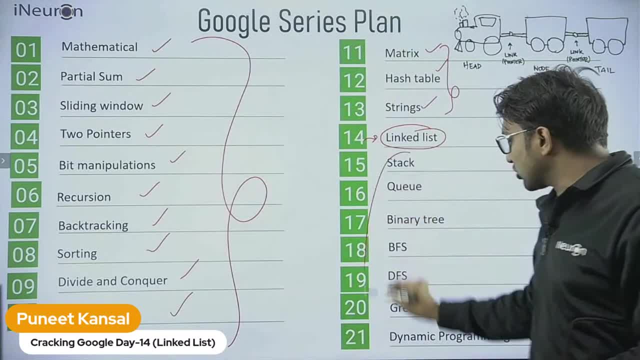 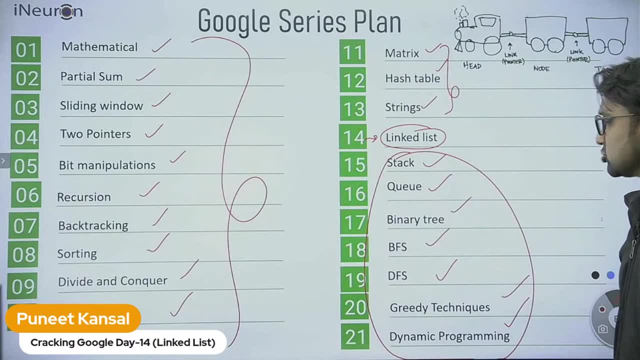 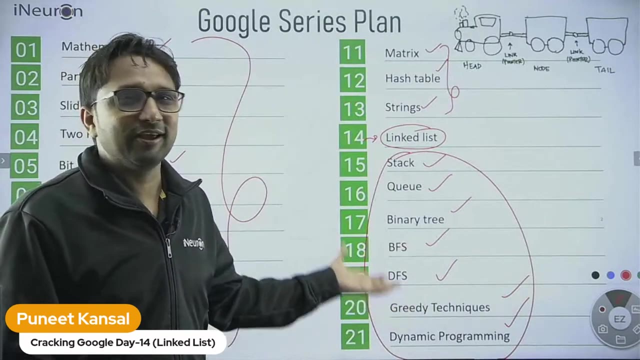 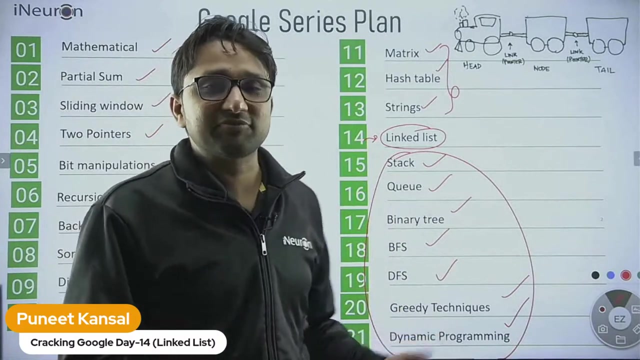 these previous videos. after this we will also cover other important topic like stack queue, binary tree, bfs, dfs, grid technique, dynamic programming. so you can see over here we are covering all the most important topic in dsa. there is nothing left. actually, we are covering all the most important topics in dsa and we are solving google problems. so definitely this series will. 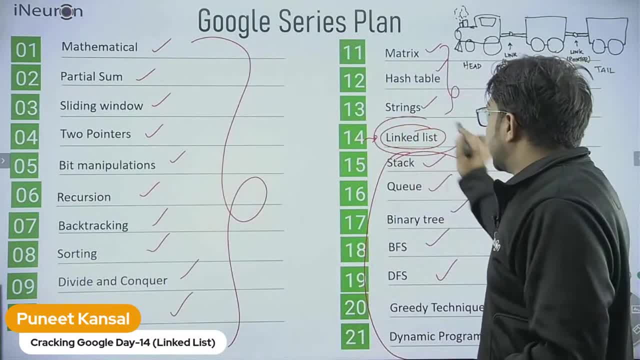 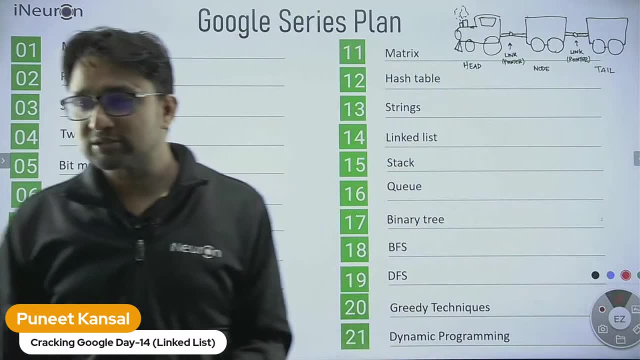 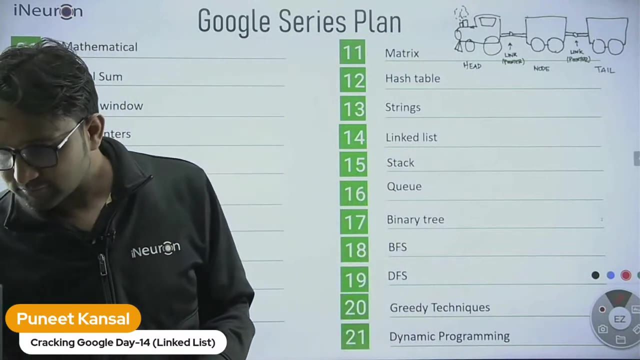 help you. let's start with today's session. that is linked list. so let's discuss, let's solve a problem related to linked list. before moving on, you can write in the chat box if i'm properly audio or not and everything is properly visible, so that we can move on. please write in the chat box. 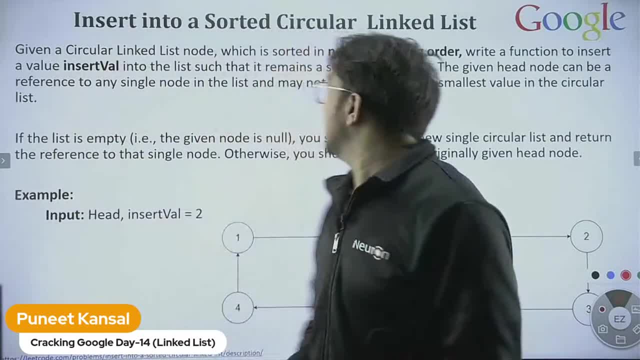 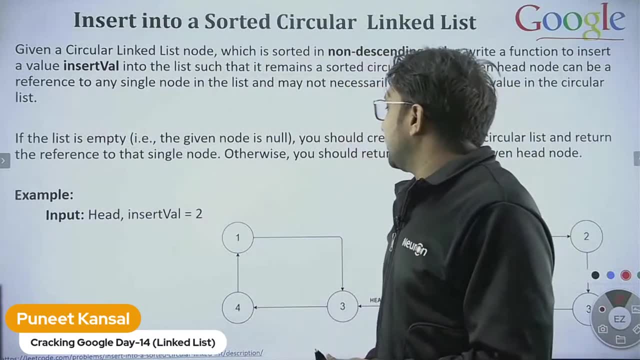 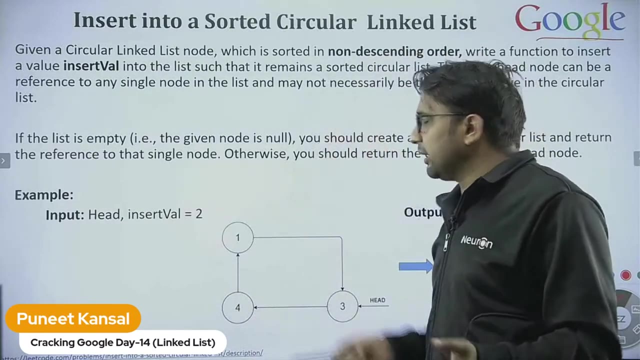 otherwise. uh, here is the problem for today. this is a google problem. today problem is little easier. you will find out little easier. uh, let's see, uh a problem. if you don't know even about linked list, don't need to worry. just check out this problem and just take it as a apt question. okay, take it as. 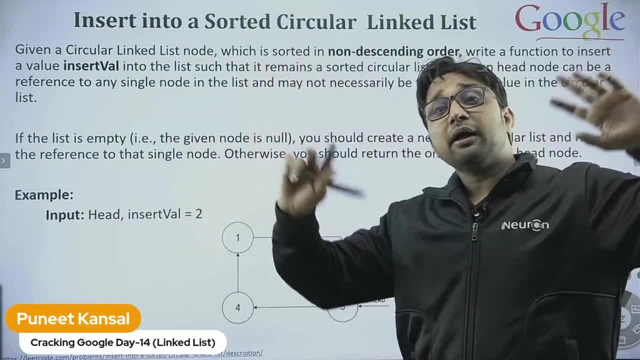 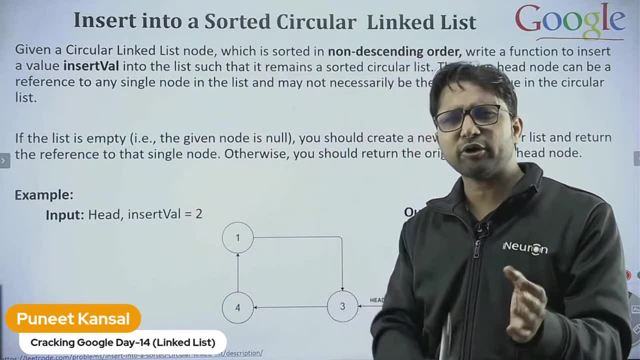 a apt question. try to think about the logic and that's it. that is the most important part, if you are coming up with the best logic or not. that is most important part. after that, okay, you need to master one particular language. you need to master one particular language and 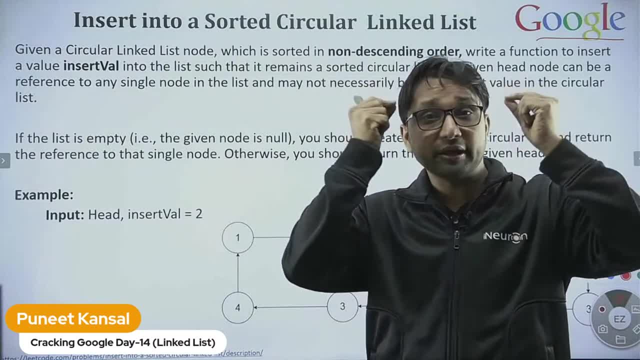 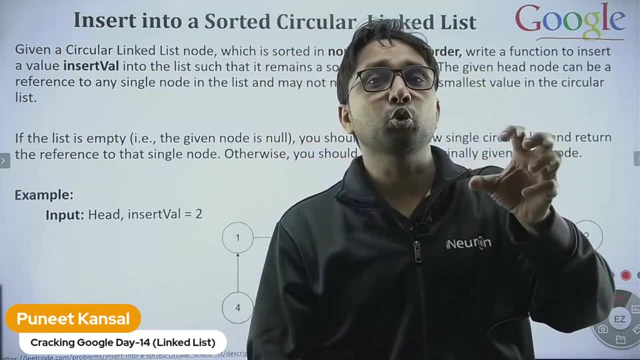 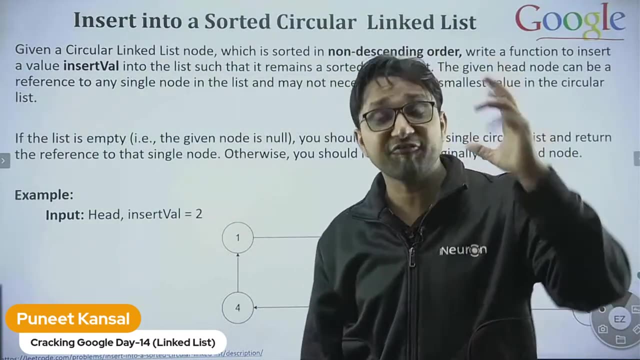 you must be able to convert your thoughts, your logic, in the form of code. so there is there is only two steps in dsa. one is you should be able to think about the logic. you should be able to think about the logic, efficient logic, i have to say efficient logic. this is the most important part. 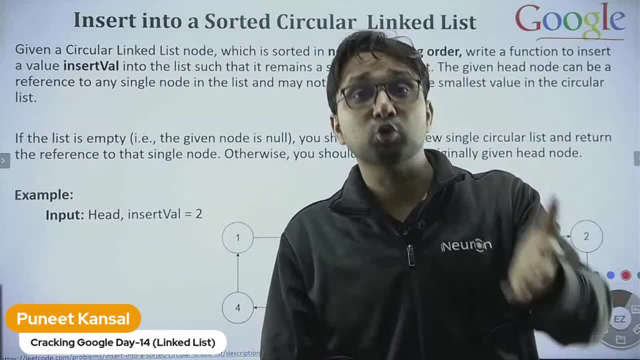 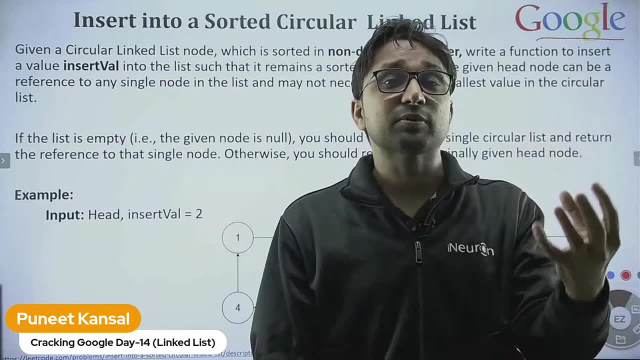 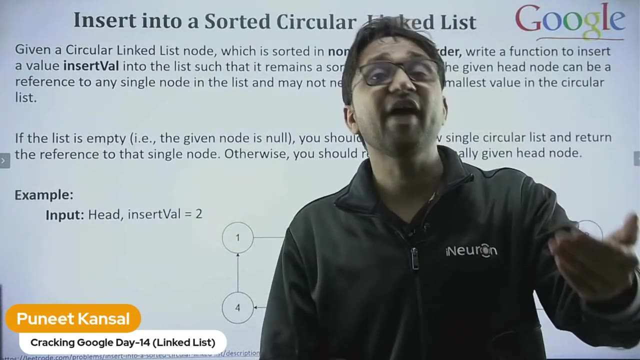 which take actually six months to some people take two years, depending upon how much time you are giving to dsa. so this thing takes six months to two year to develop the logic. okay, so there's somebody is giving you the problem and you are coming up with the efficient solution. so this thing comes. 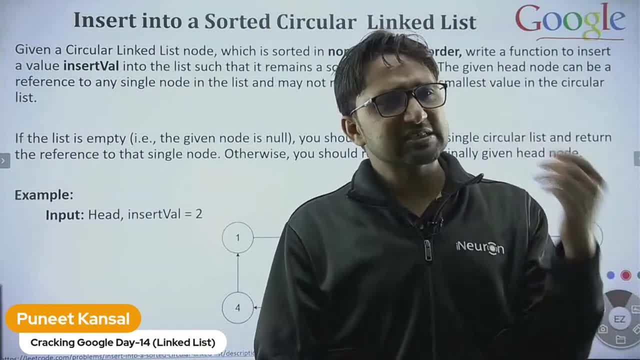 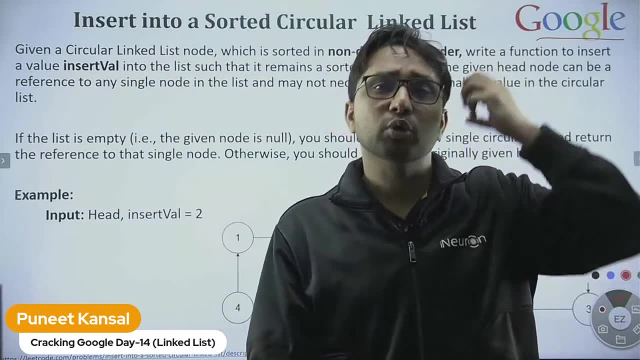 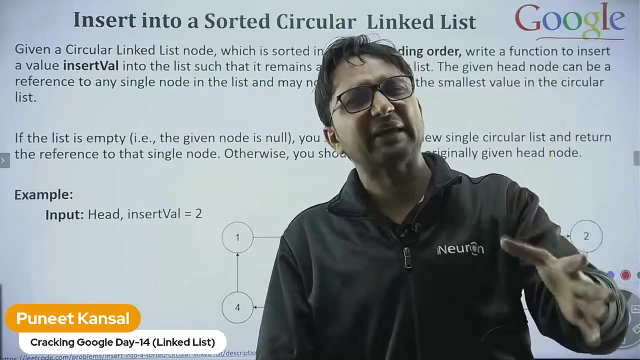 out after lots and lots of practice. this takes six months to two year. and second part is that once you are coming up with the logic, you need to write in it in the form of a code in any language, either c plus plus java, python, whatever javascript, whatever language. so after solving, actually 100. 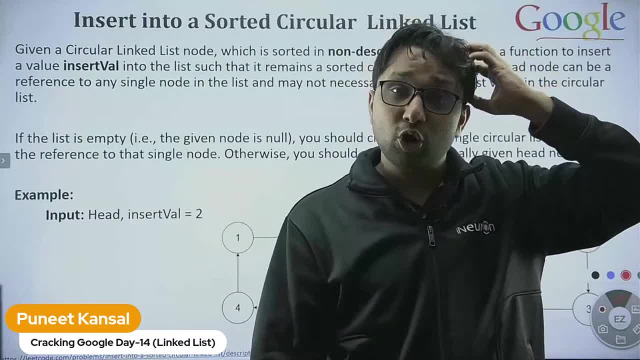 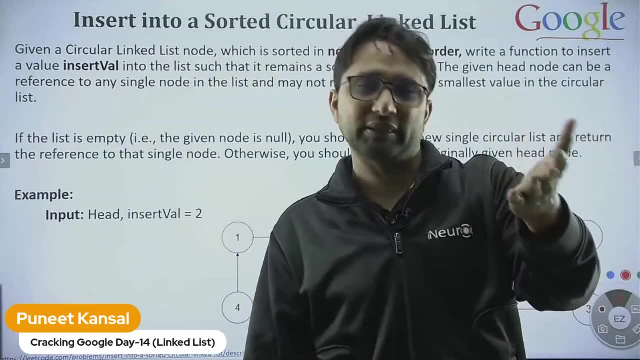 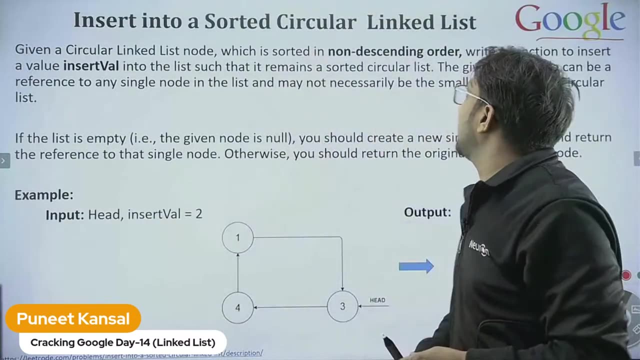 problems. you will find it easy to convert your thoughts in the form of the code. that becomes easy. that is easier part that take max one to two month. but the most time consuming part is logic building. so let's solve one problem related to the google and can you tell me? can you tell me, okay, do. 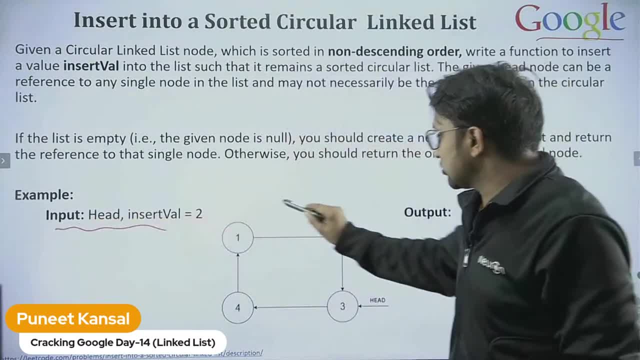 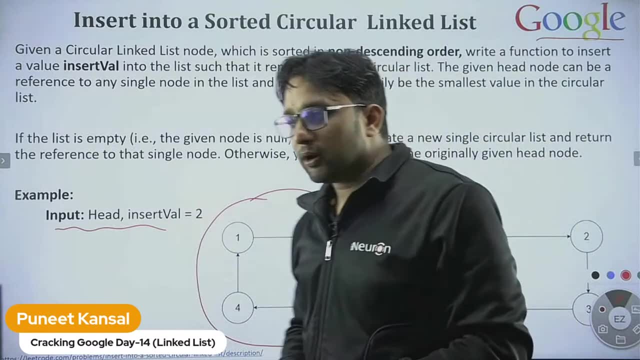 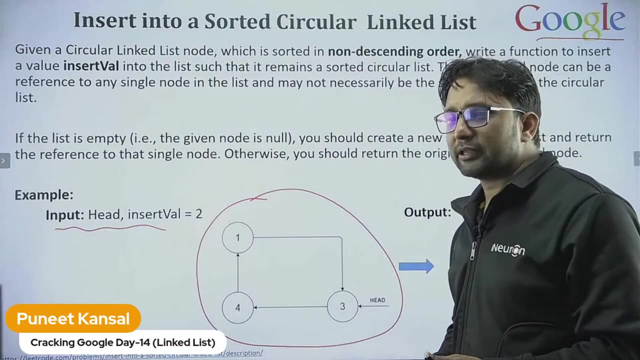 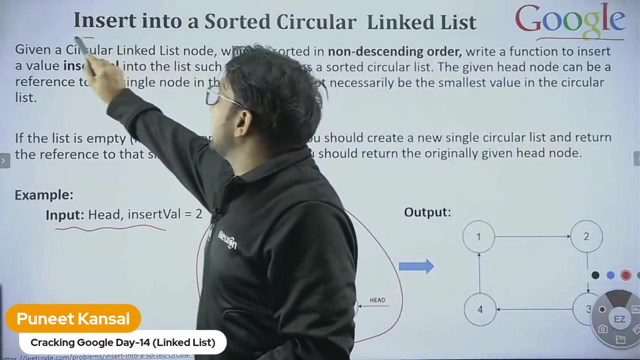 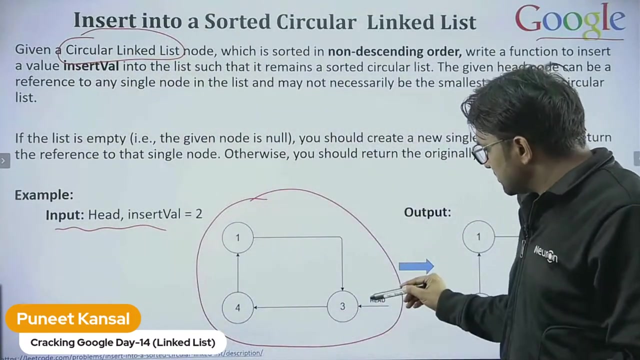 what will be the output for this input? so this is the input given to us and you need to tell me what should be the output. hello, uh, good evening, thomas, so i will check. well, i forgot something at the problem. yes, you touched that. no, so here you are in one of these two, Paulo here. 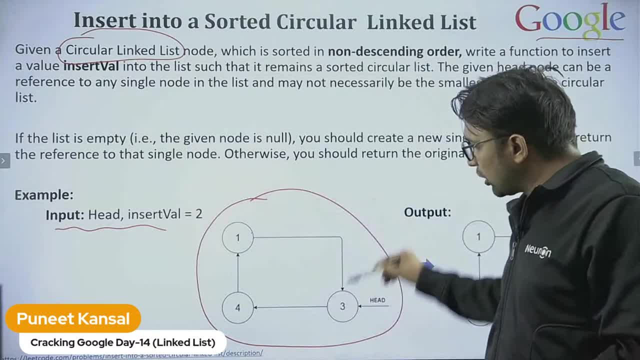 is correct. so here is the code. it's been searching, but it doesn't seem to work. ok, okay, so here is the command: измен equals to ten time solution, but theanno it says block. leave this call on H2 and the If so, to break the string in line with your element. then I cannot. 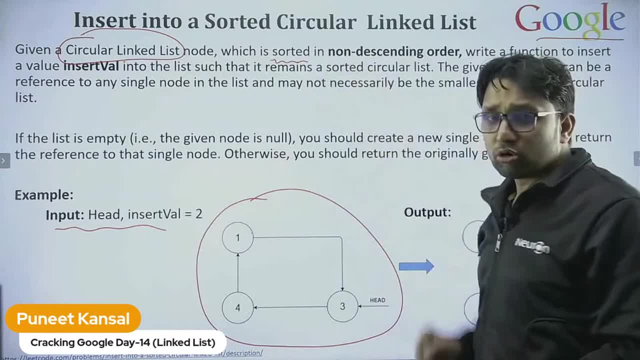 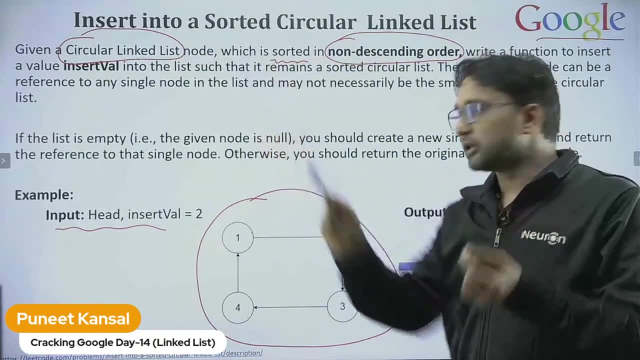 so far as everyone is using Je organise an ink element, it has been working. so could you see that the list is sorted. actually, the list is sorted in non-decreasing order. when non-decreasing order means increasing order, the list is sorted in increasing order. see three, four, like you can say. 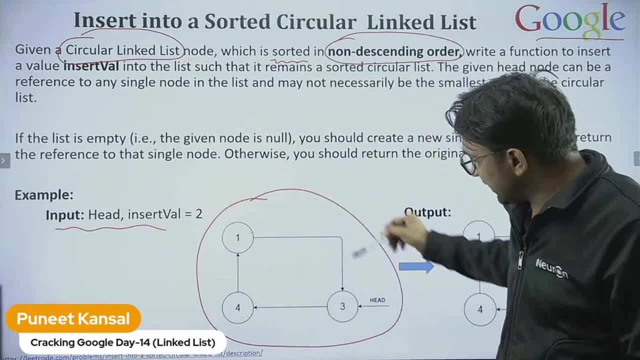 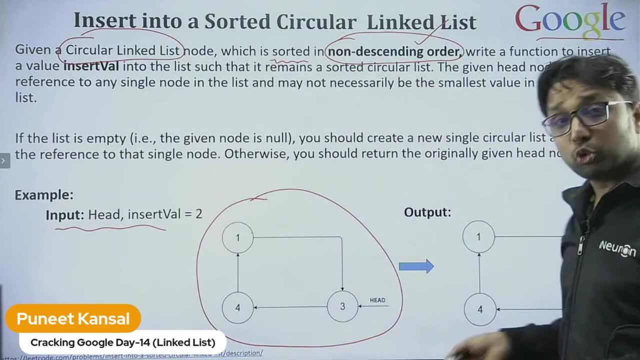 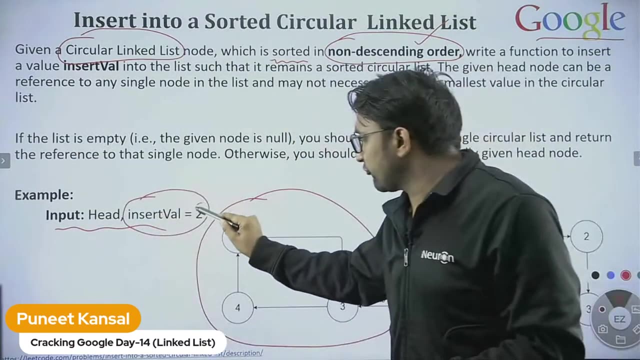 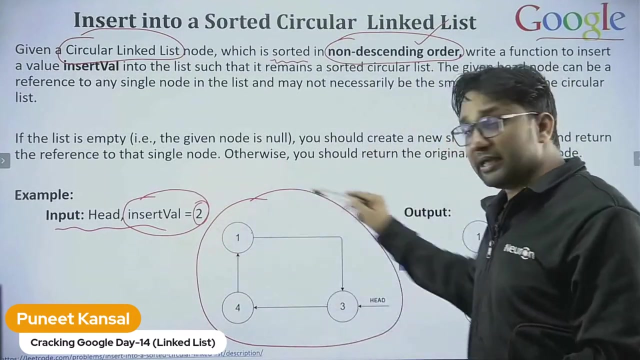 one, three, four. so list is in increasing order. list is in increasing order. okay, fine, what you need to do in this is you, they provide us one value. they provide us one value here. they for this input. they provide us value two. you need to insert a node in this link list, in this circular link list, such 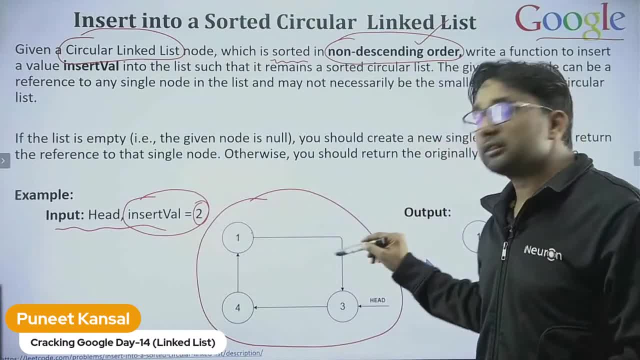 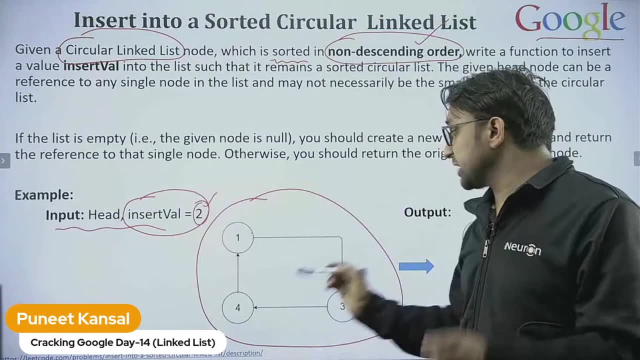 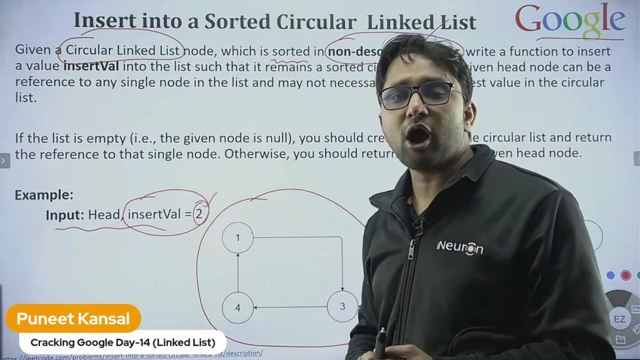 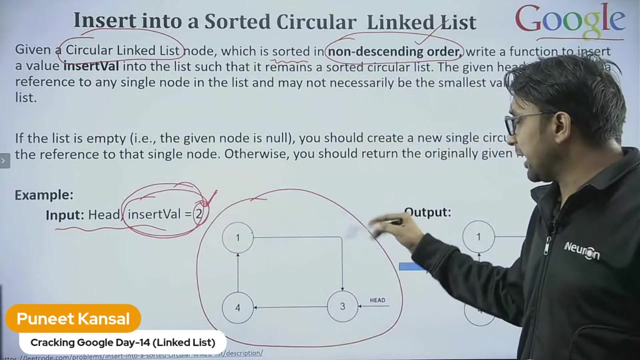 that after inserting the node, still the link list is sorted, even after inserting this node. after inserting the node, still the link list is sorted. so any idea coming to your mind, please share anything coming to your mind- how you will insert this value, this value node here so that we get this output, so that we get this. 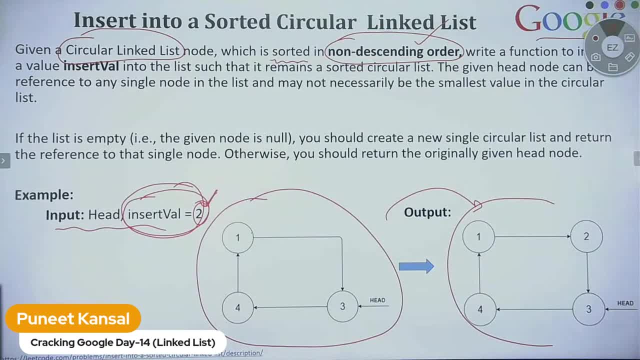 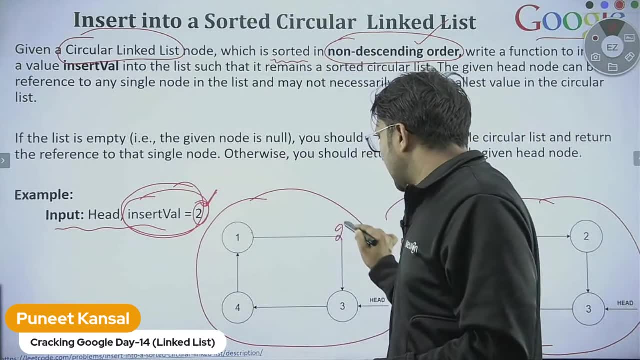 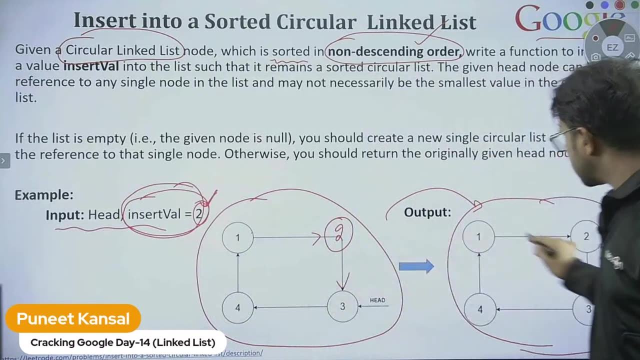 out. this is the output. okay, this is the output for this particular input. so we, if we will insert two, where the two will go, definitely the two will come here only between one and three. the two will come between one and three. now you can see still the. 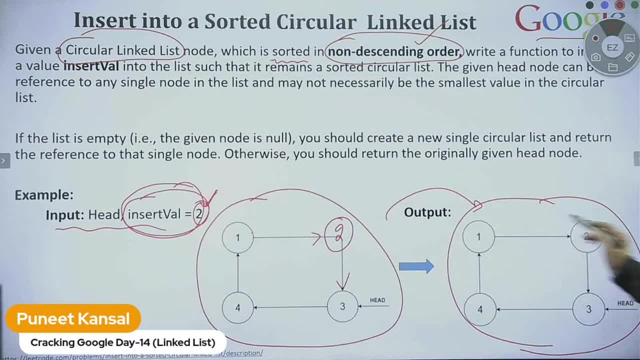 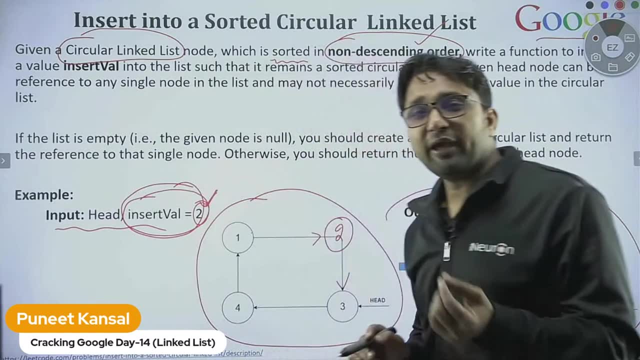 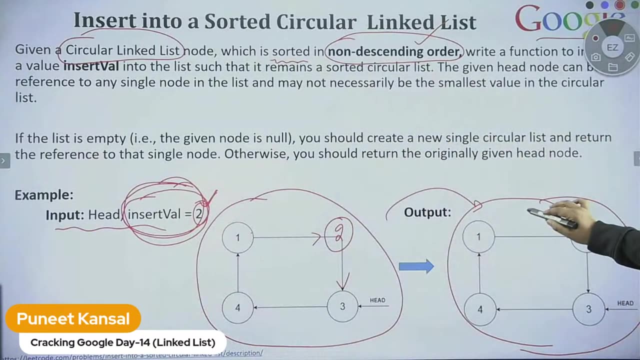 still the link list is sorted only. so one, two, three, four. so that is sorted. only we need to find a place in the circular link list where we can insert the new value as a node, so that even after insertion the link list is sorted only. so that's it very easy actually. uh, how you will. 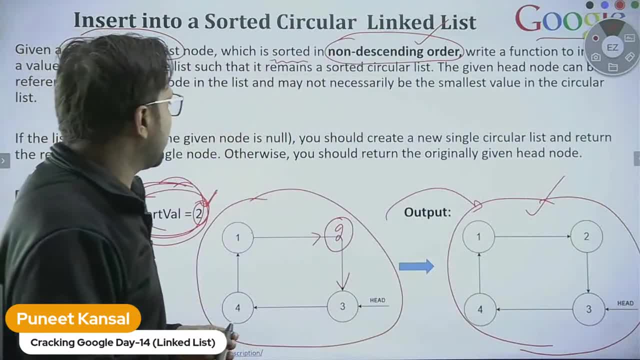 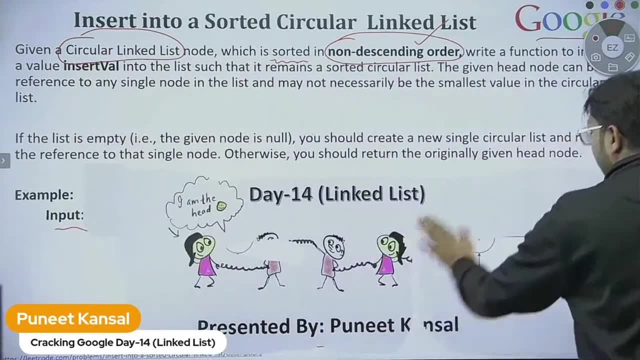 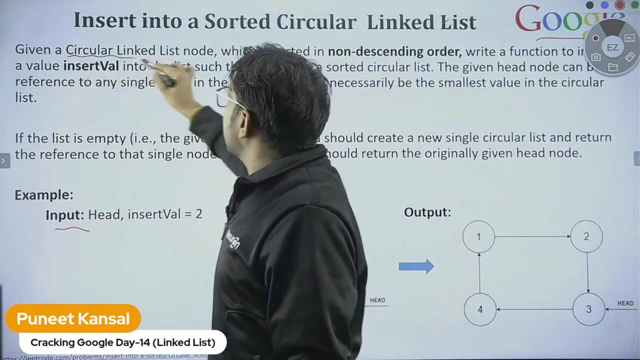 find out this thing. any idea, thomas, if coming to your mind or anyone else you can share with me. otherwise, let me read the problem statement again. let me read the problem statement. let me read the problem statement. given a circular link list. yes, they provide a circular link list. 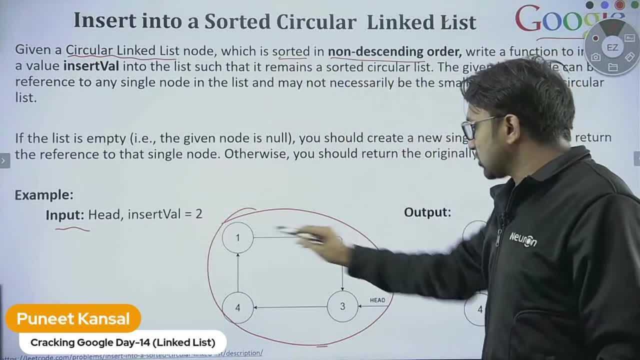 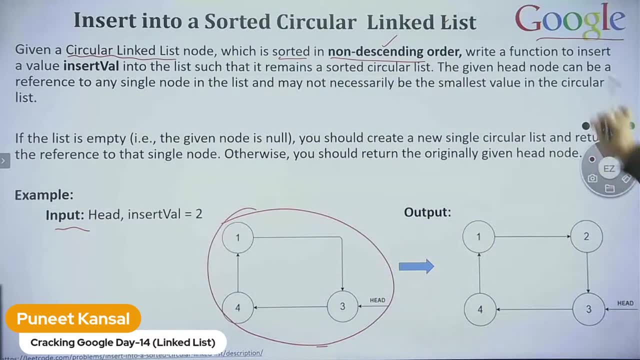 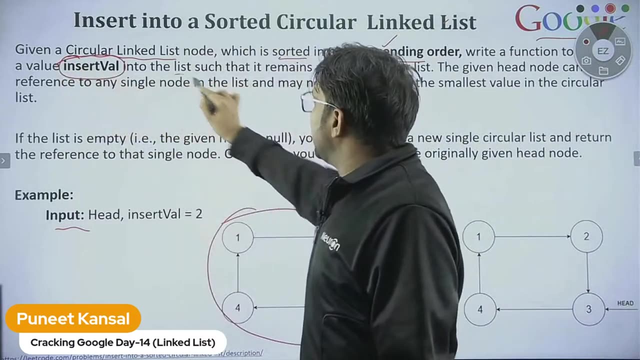 which is sorted in non-decreasing order. yes, that is sorted in increasing order, you can say: or non decreasing order. write a function to insert. write a function to insert a value. we need to insert this value into the list, into this list, such that it remains sorted it. it remains sorted circular. 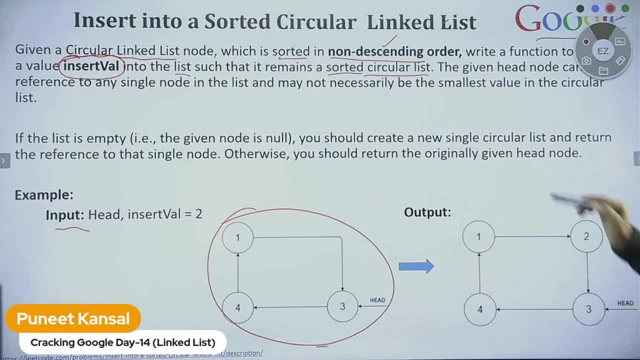 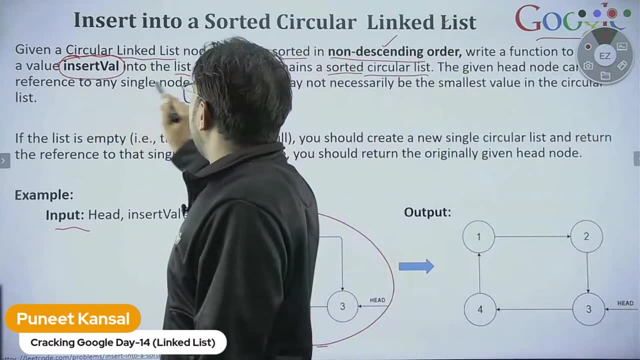 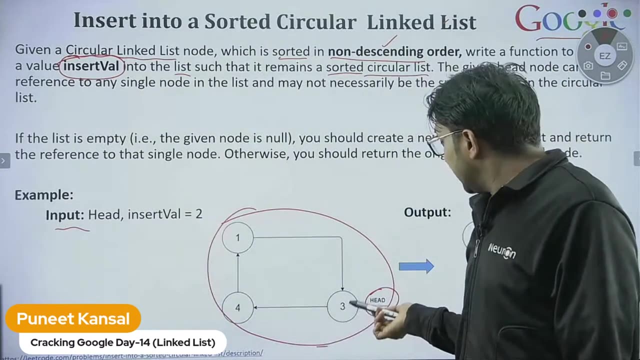 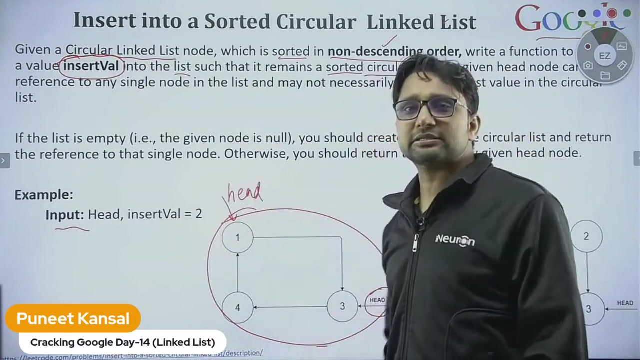 link list. so after insertion, still, this should remain sorted. okay, the given head node can be a reference to any single node. so they are. they are just saying that the head node they provided that can be, that need not be pointing to the minimum element. that need not see. whenever we pass the link list, whenever we provide the link, 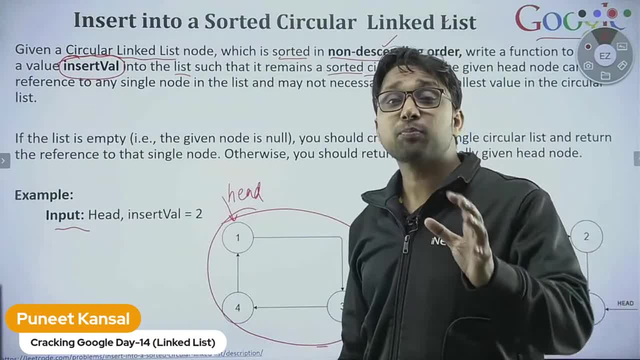 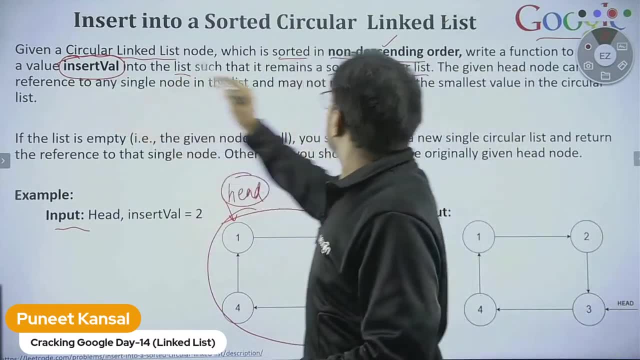 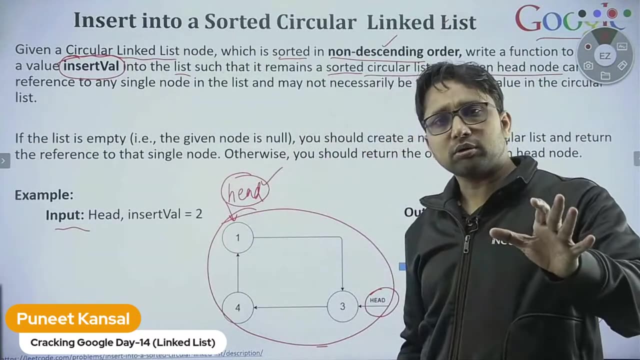 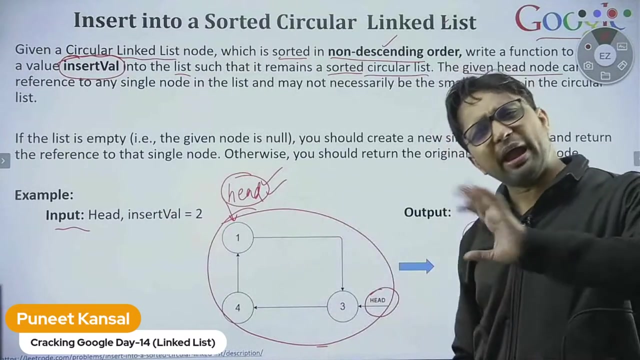 list, then we do not, we just provide the head node, we just pass the head node, that's it. but here in this line, what they are saying is that they are providing the head. the head can point to any node, either 1 or 3 or 4, if there are n nodes. so head can point to any. 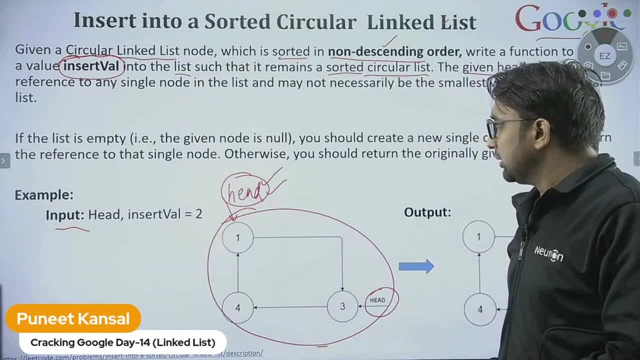 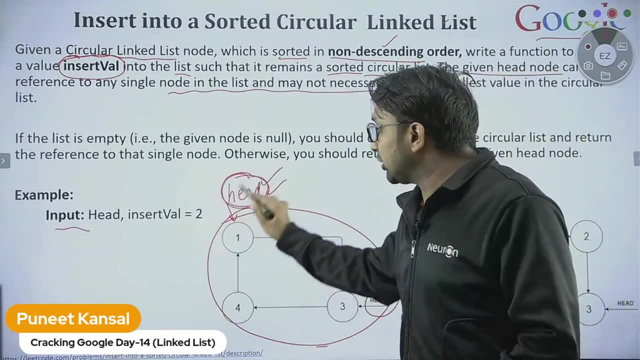 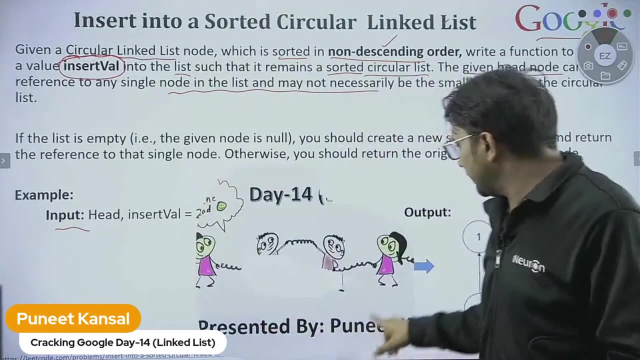 node, any node, head can point to: okay, it's not compulsory. in this line they are saying: is it's not compulsory, that head will point to one only minimum element only. okay, see here. also, here itself, the head is pointing to 3. so let me read the statement, the given: 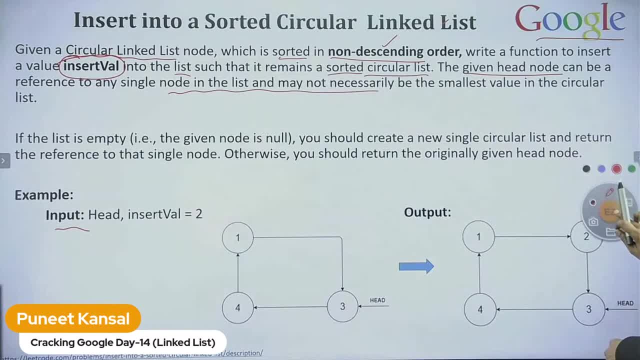 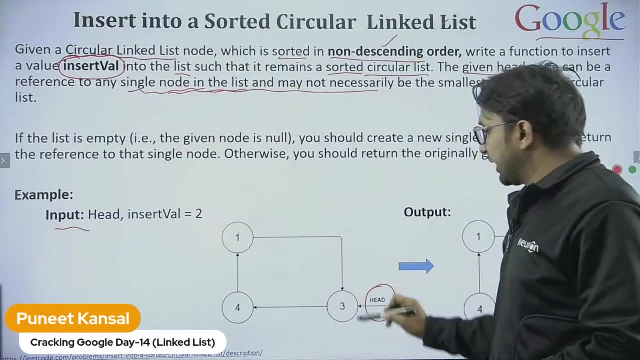 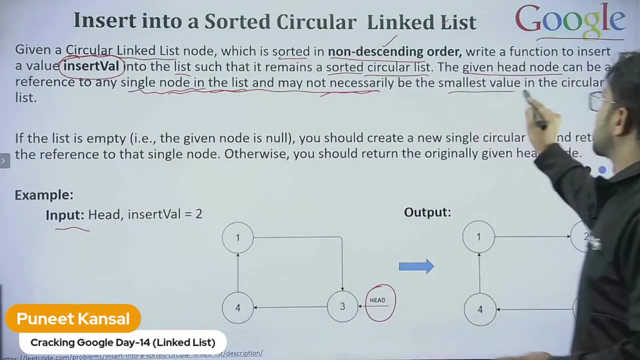 head node can be, can be reference to any any node in the list. so given head node can reference to any given any node in the linked list. so not necessarily to be the smallest value in the circular list, not necessarily head will point out here, so they will provide. 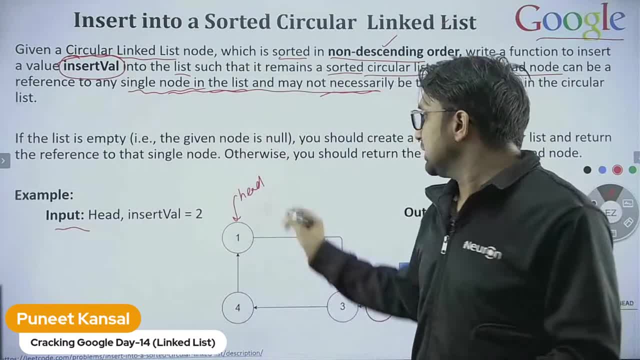 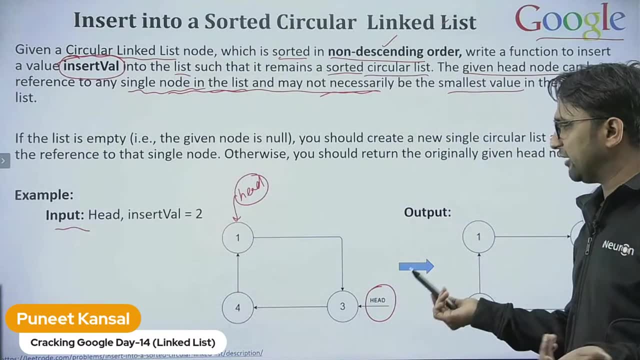 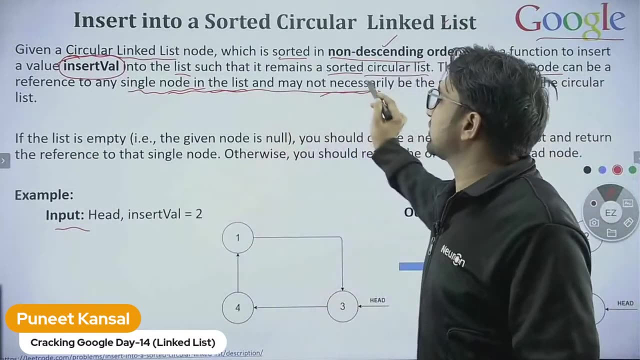 provide us the list. how, how somebody provide the linked list? they simply provide the head of the linked list. so head can point to anywhere, either to 1, 3 or 4. that is not fixed to minimum element. this is what they are saying. fine, if the list is empty. one more thing they are. 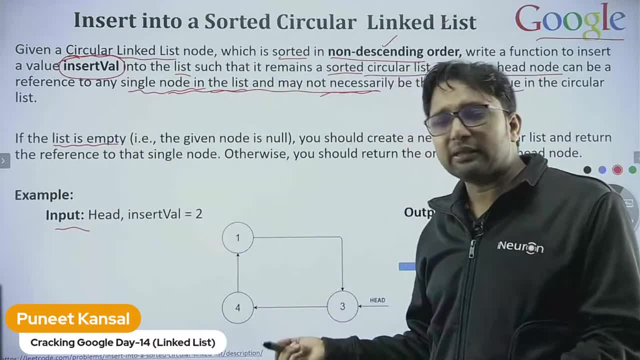 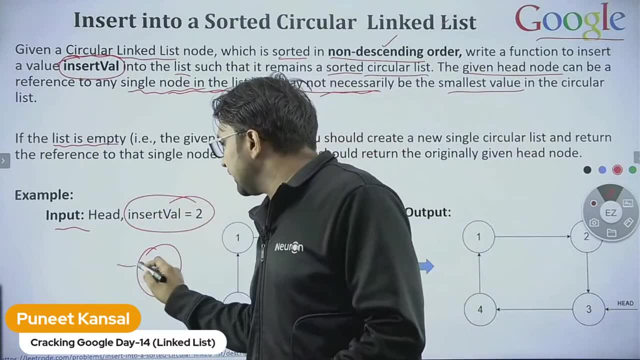 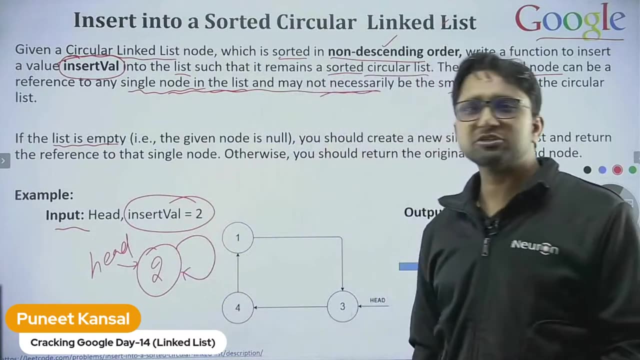 adding. this is the edge case, actually. if the list is empty, then what you will do? if you want to insert this, then you can make a node with this value and make it as a head only list. this should point to itself. this should point to itself. this is what this statement. 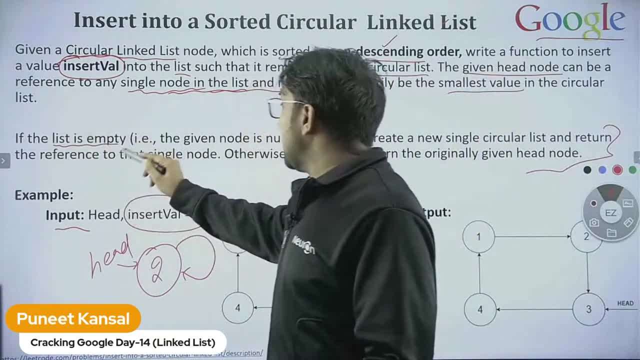 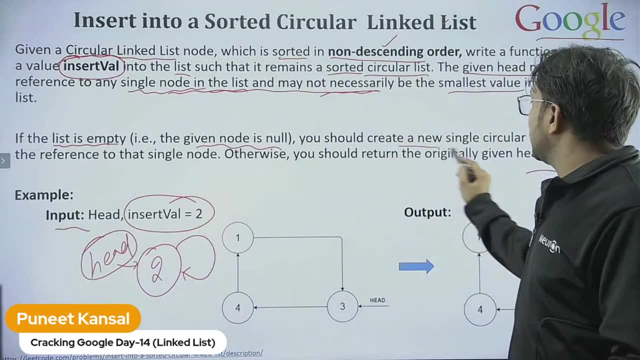 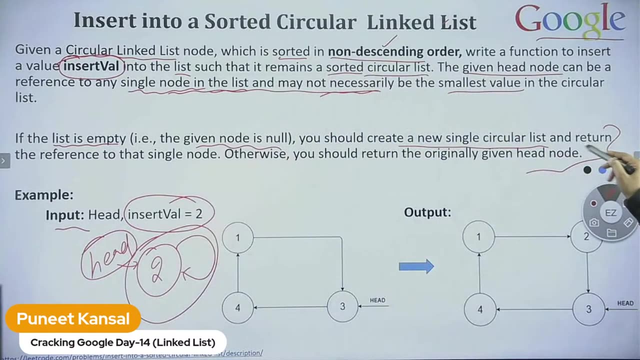 is saying that we read it if the list is empty, that is, the given node is null, if the head is null. if the head is null, you should create a new sindal circular. yes, we created a new single circular list, single node circular list, and written that reference of that node. 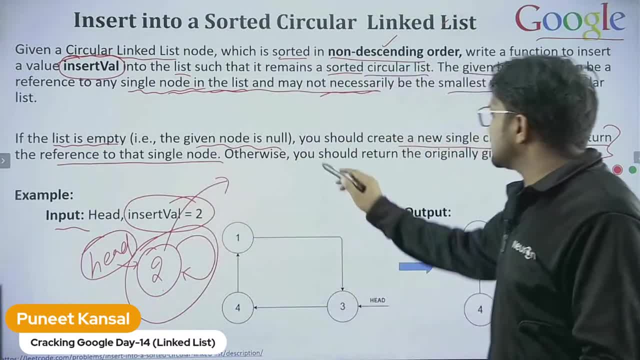 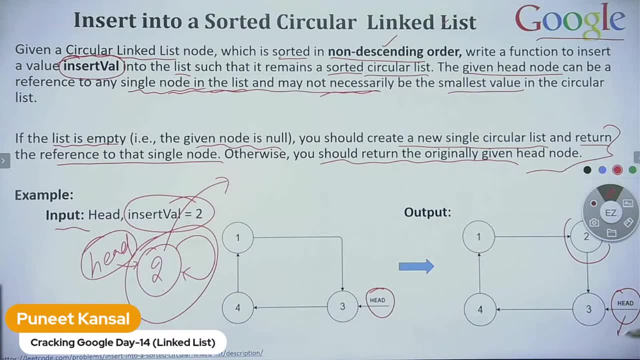 so we will return written this as an output. then we commit another reference to that node, so we will return. return this as an output. Yes, we need to return the head after inserting two. also, we will return the return the head of the after inserting two. we will return the head of the list back. fine, this will be our. 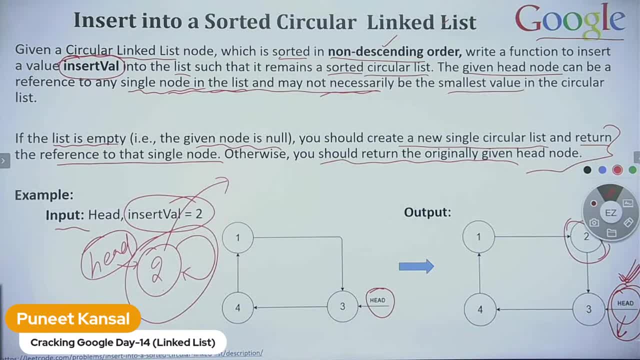 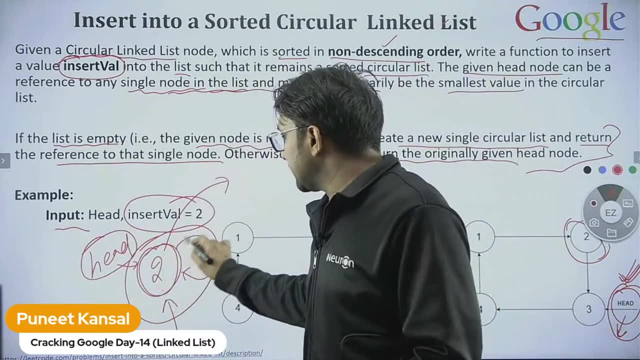 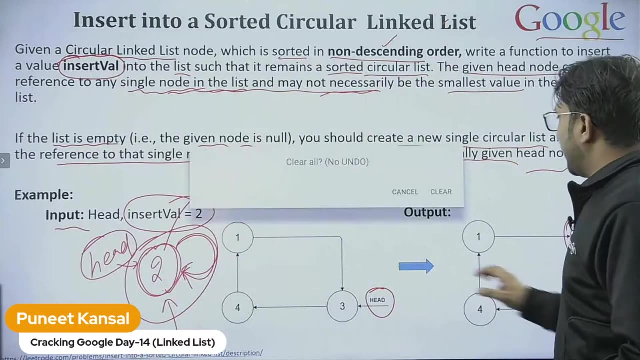 this will be our output. you can say we will returning the head or we are returning this single node. if there is no node at all, we will create the node, make it circular and we will return this. that's it. this is what we need to do. so what is the question? okay, i'm repeating again. 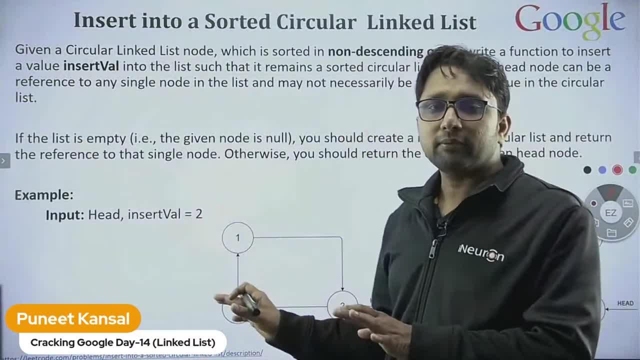 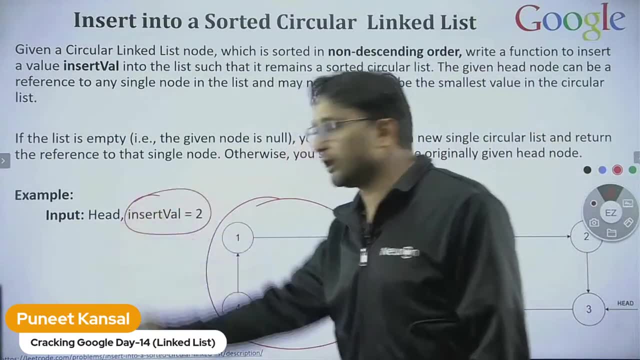 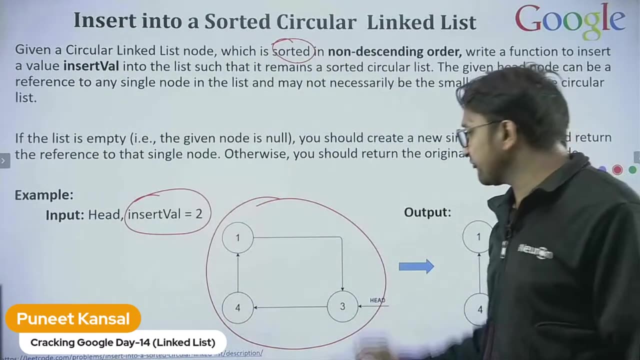 what is the question? i'm repeating again over here, simple: they provide us a circular linked list. we need to insert a node with this value in this circular, sorted, sorted linked list, such that after insertion of the node, such that after insertion of this new node still the list is. 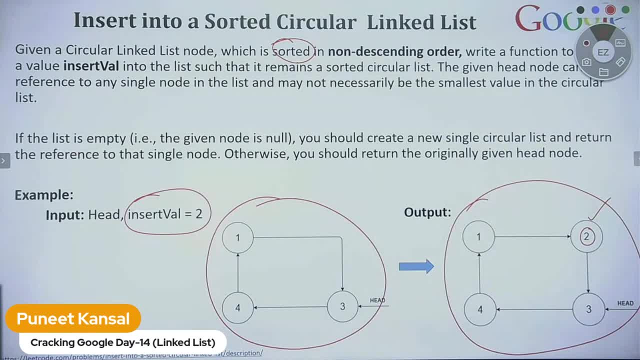 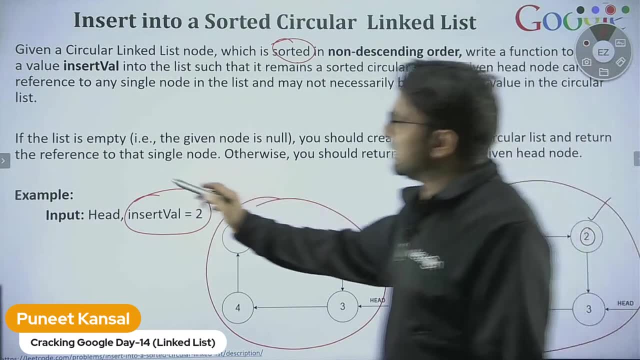 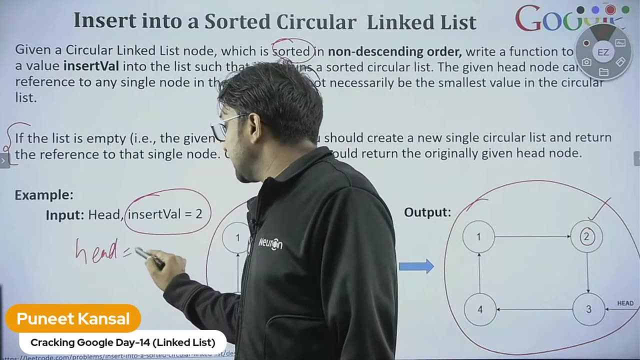 is: see, still, this circular list is sorted only one, two, three, four. yes, that is still sorted. that's it. and in this they are saying that if the list is empty means head is equal to equal to null. then what you need to do, then you need to. 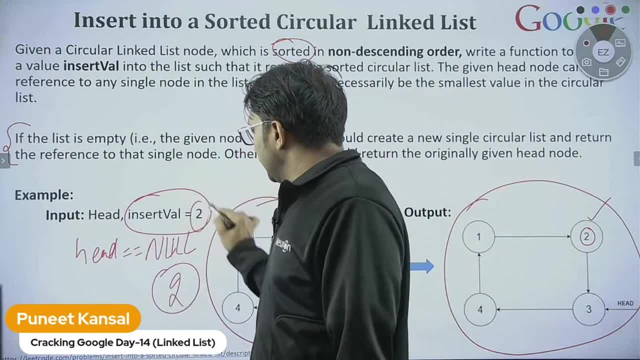 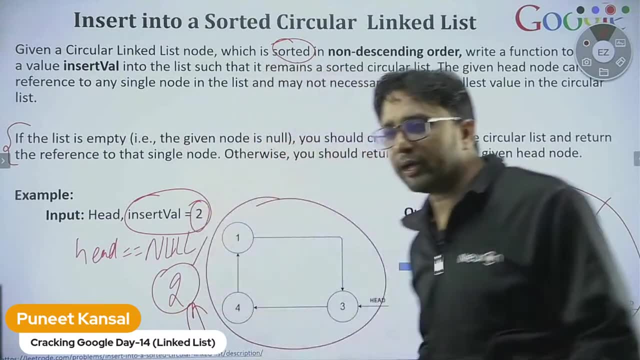 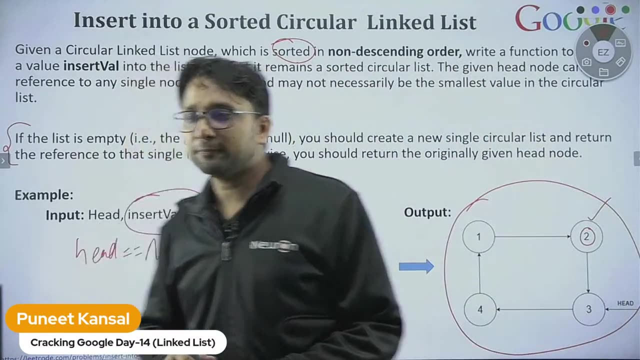 then you need to create a new node with this value and make it to point to itself. that's it, and return this node. that's it, fine, okay, i hope the question is clear. i hope the question is here. hi slc, nice to see you here. so i hope the this question is clear to people. if any doubt in the 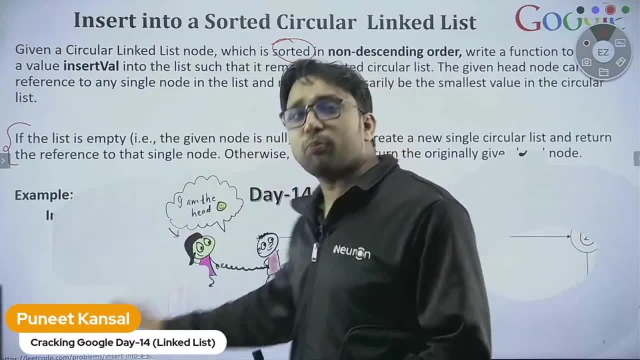 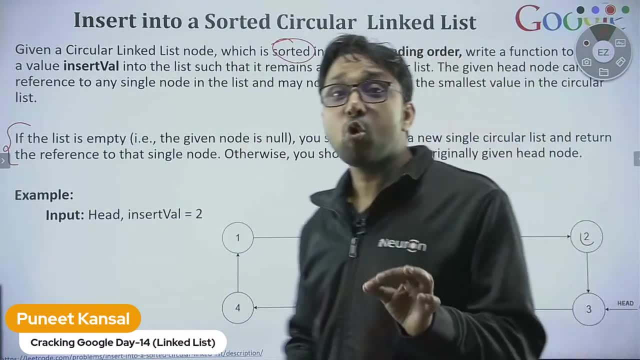 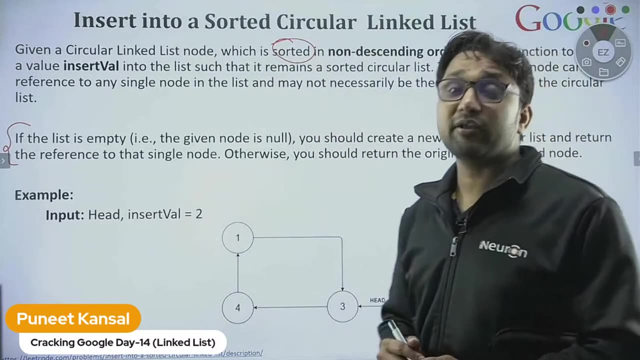 question. please write in the comment section if any doubt, please write in the comment section. please write in the comment section if any doubt is coming related to the question. otherwise, please let me know what should be the logic, how you will approach this problem, please. please reply. this is very important. if you are replying or not, this is very. this is making our session more. 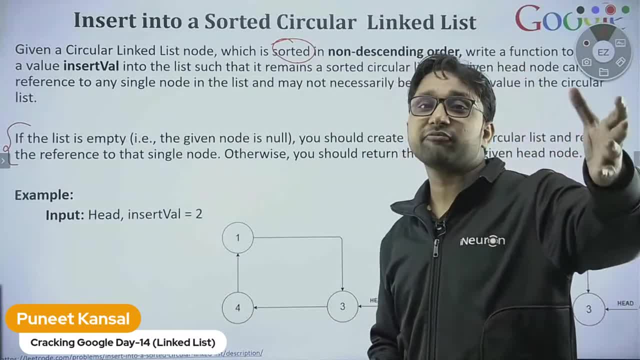 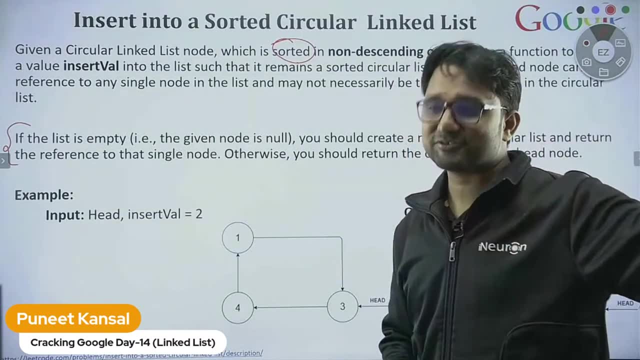 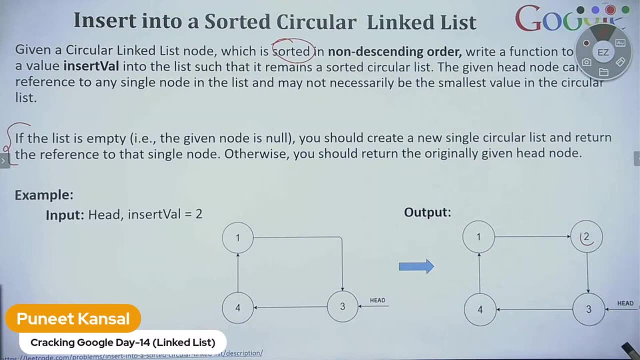 interesting. the more you are replying, the more session will be go interesting and that will benefit many students also, not only you, that will benefit many students also. please reply, please reply what should be the logic, how you will solve this problem. okay, let me go to the 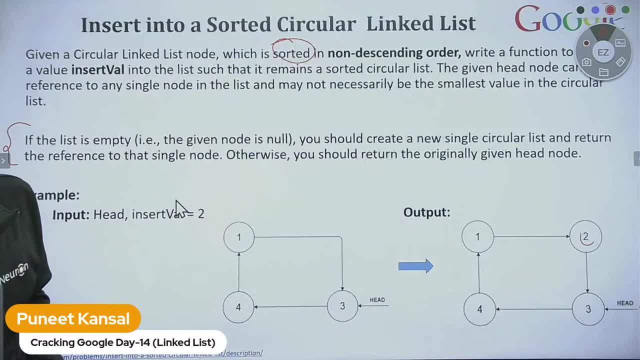 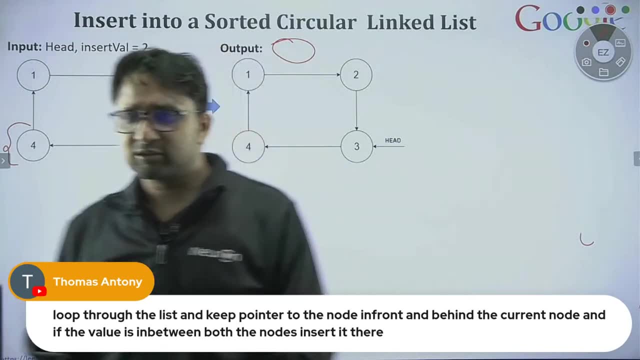 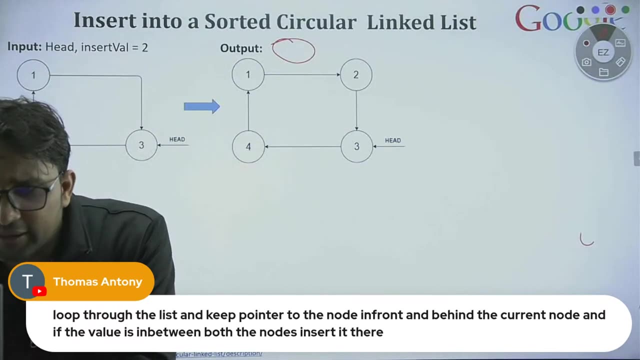 so there is a one logic from thomas. let me share that with everyone. here is the logic shared by the thomas. so what? let me read what thomas is saying. loop through the list and keep the pointer to the node in front and behind the current node and if the value is between the nodes, insert it there. 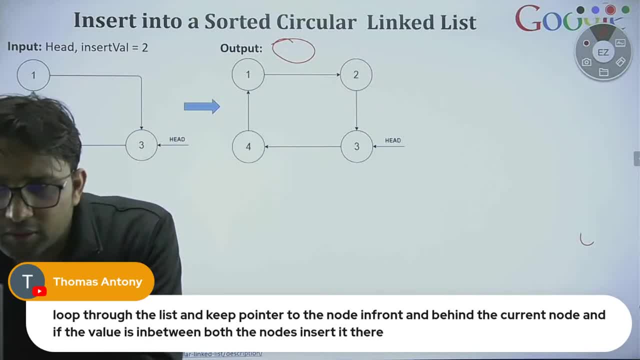 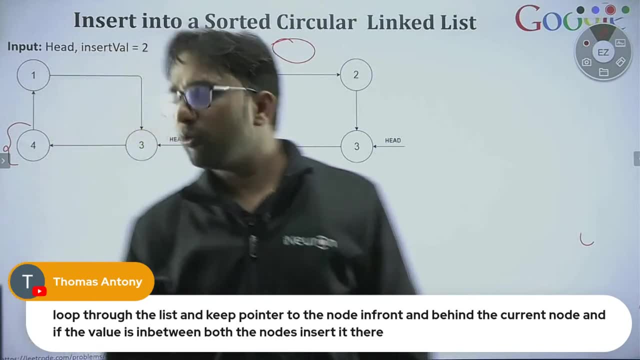 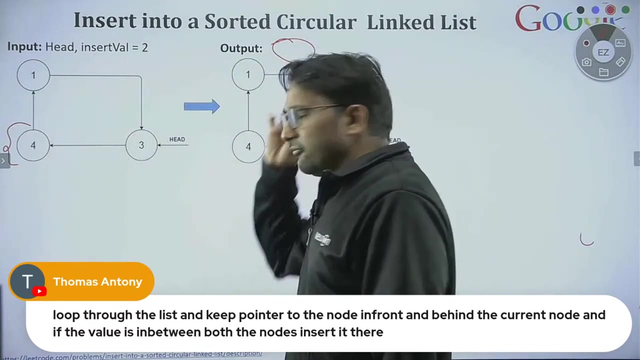 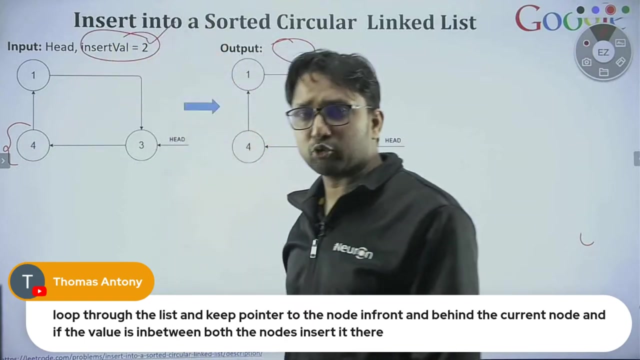 okay, fine, okay, so let me, let me try to implement the same thing what thomas is saying. so, even before that, okay, one last question, you please tell me. first of all, we need to insert this as a node, this value as a node we need to insert. we need to insert two as a new node. we 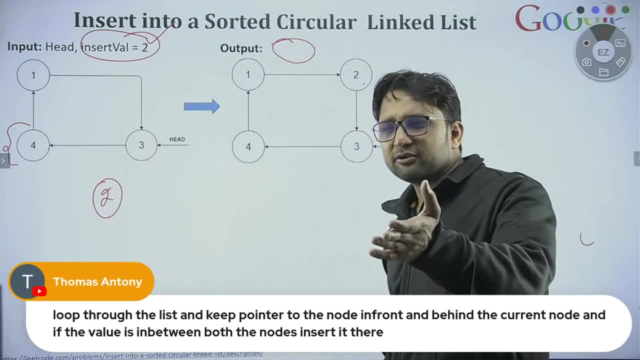 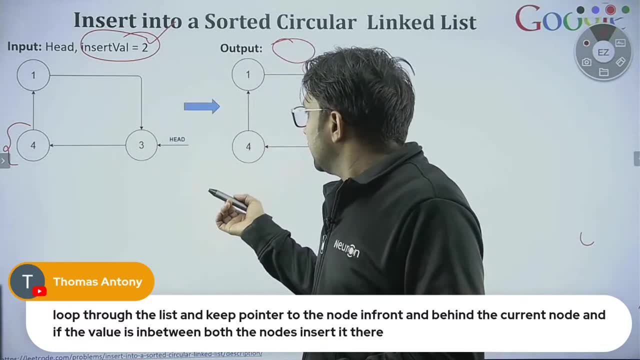 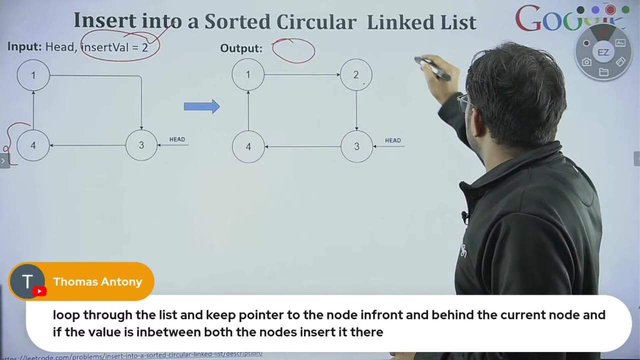 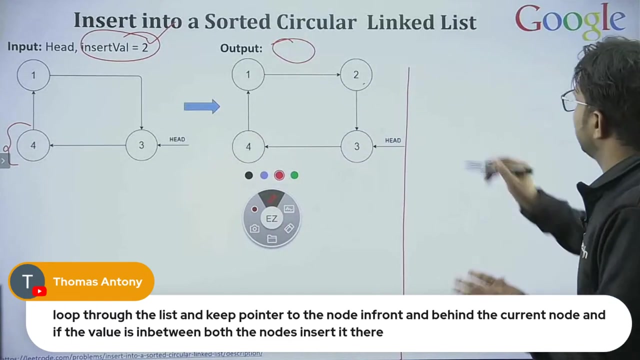 will insert over here. can you give me one condition, two people. can you please give me one condition, although, thomas, you have written that, but okay, maybe you can verify so you have already written. otherwise, still, i'm writing over here. so let me write over here, let me take this over here, and here we have space. fine, so if i want to, 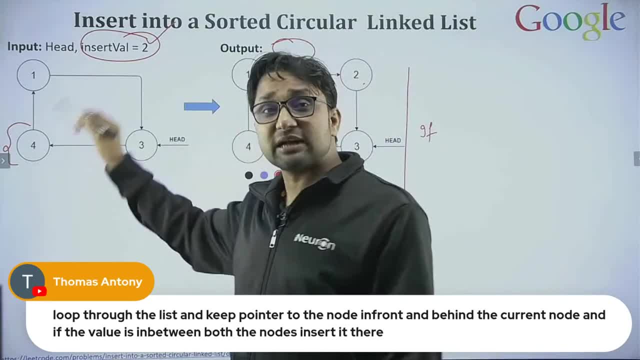 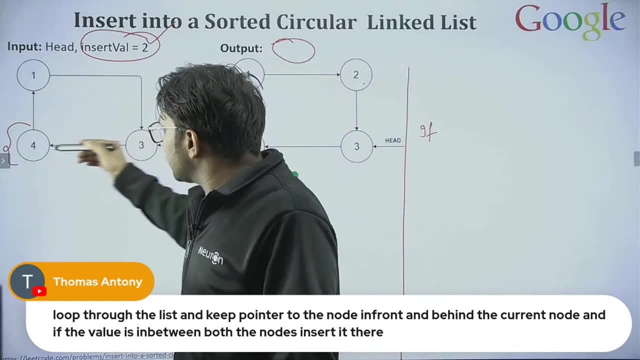 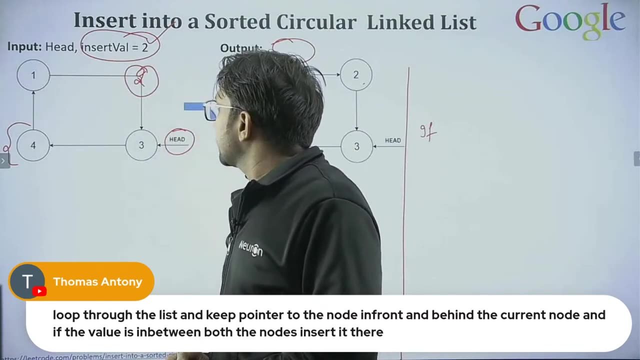 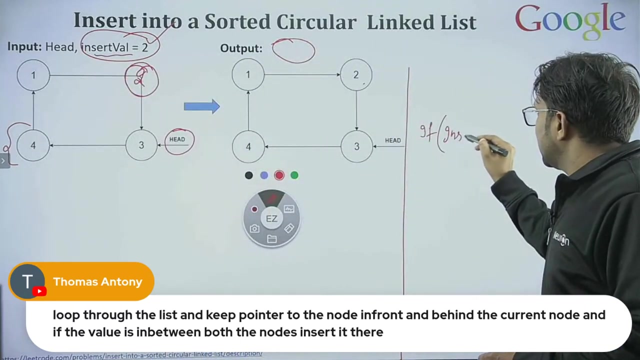 find out. i want to find out where i can insert this node. so you are saying that start from the head, keep moving on, how i will find that. okay, two will be inserted here you are saying that. you are saying that if your inserted value, if the inserted value insert, insert. well, if this value is greater, 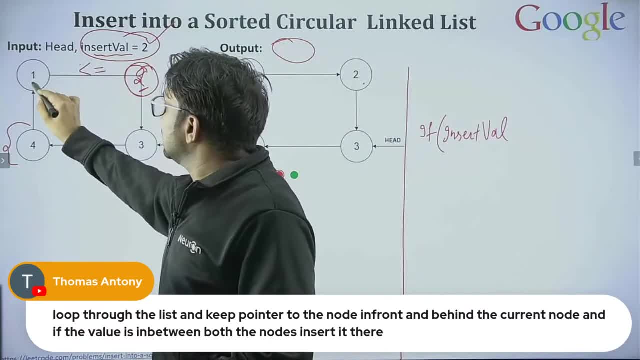 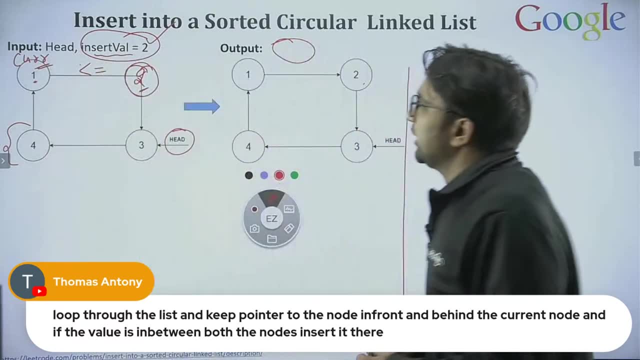 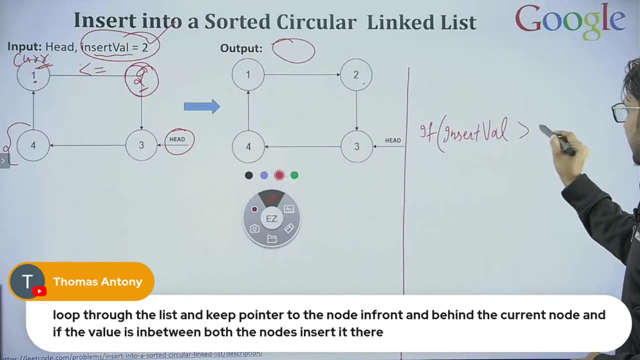 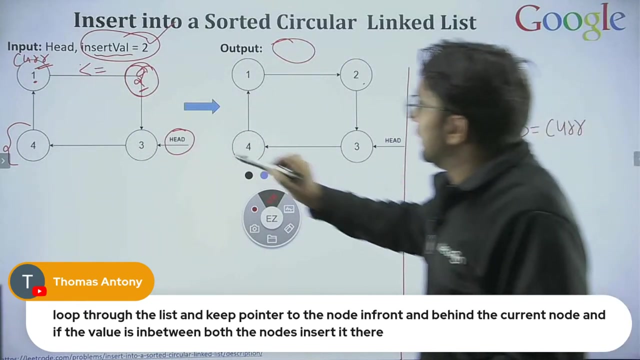 than greater than equal to: okay, let me give it a name: current current value. okay, so let me give it a name present. if that is, uh, let me give the name to this uh node, that is, current node. if this value is greater than equal to current current value, and and this value is. 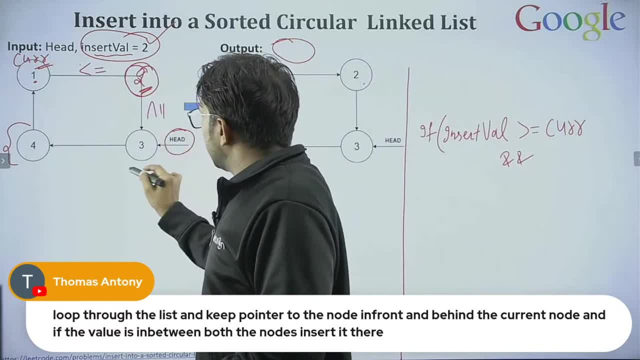 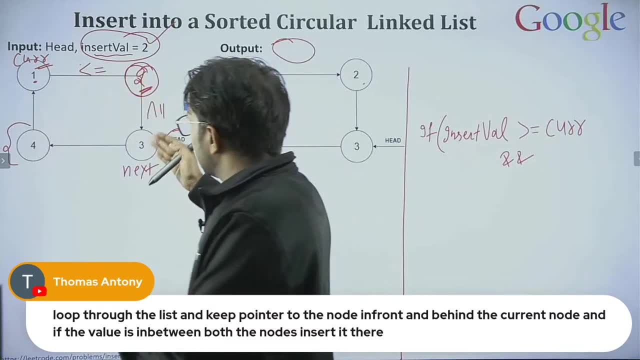 smaller than equal to. okay, let me give give the name to this next node. so you are moving means so you are moving. uh, one point, one point, one point, single point, most wunderbare one. that's what you mean. remember circle reference, right where here hundred percent ofb is斤 respect. 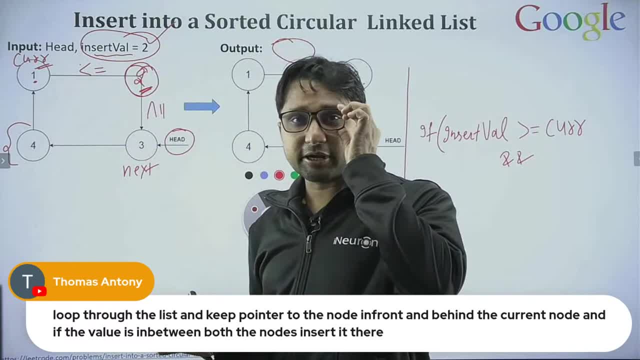 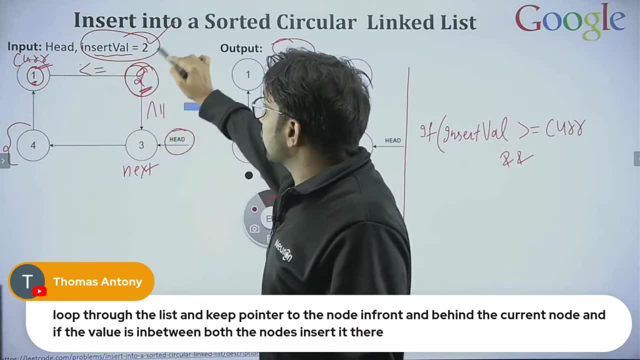 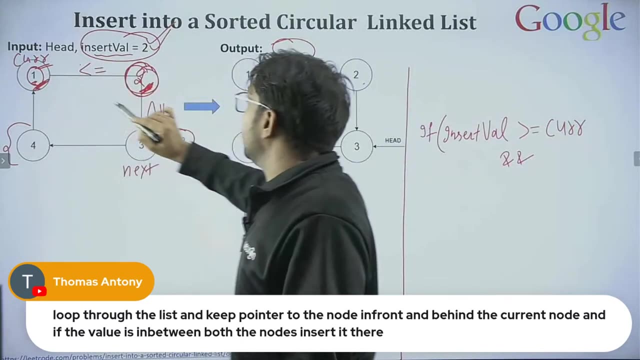 node to another and you are finding a. you are finding a relation that if you find a node whose value is smaller than the smaller than this insert value, but this, well, sorry, sorry, this value is greater than this value, current value, but smaller than the next value. so let me write. 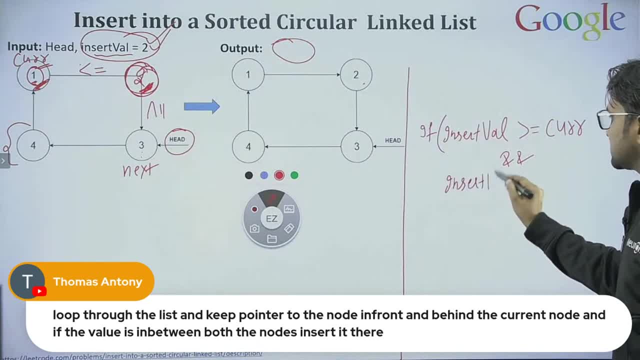 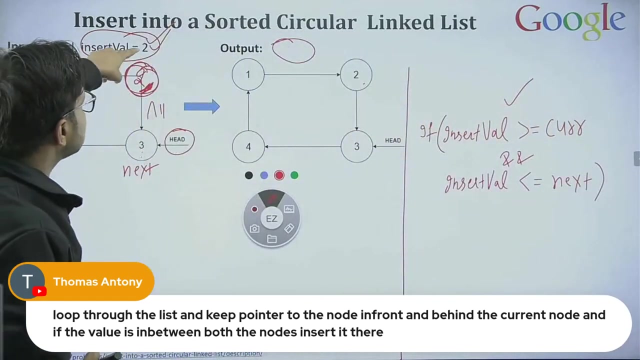 another condition: if insert, insert well- is smaller than equal to smaller than equal to next value, next value, so please verify, is this condition will work, is this condition is will work? to find out the place, to find out the place where we need to insert the two where we insert where. 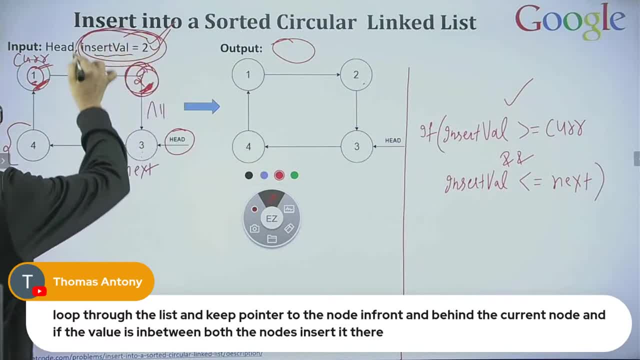 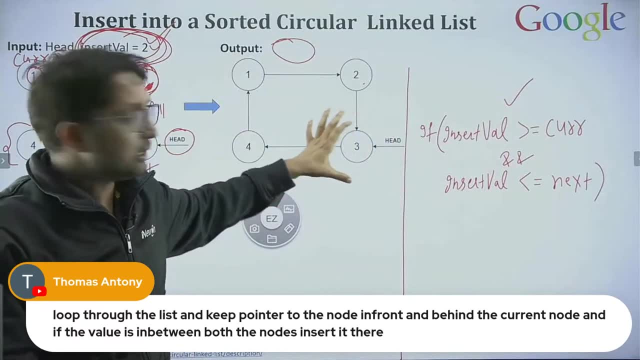 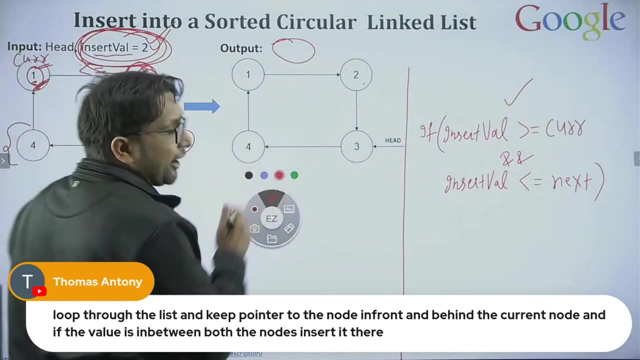 we need to insert the insert a node with this value. is this condition will work or not? please verify yes or no. please write in the chat box, but I'm what my question is. I am representing the question. the question is, I want to find out a place, a place in my linked list, in my 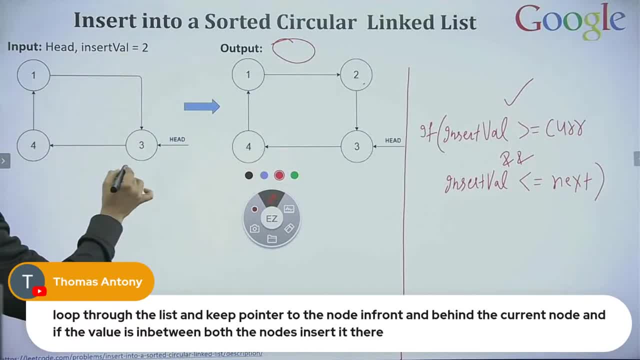 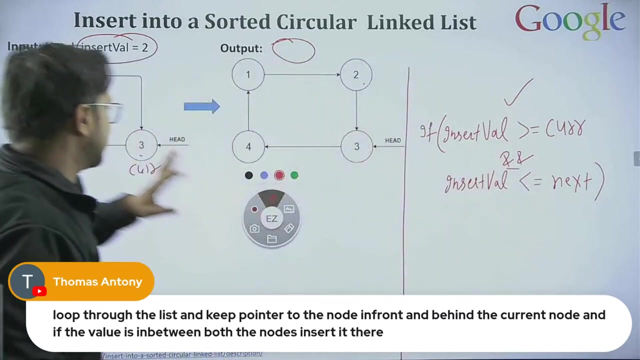 linked list. this is a linked list. okay, currently this is the current and this is the next. so I'm finding my insert value is: that is, that is greater than current. no, that is not greater than current. so this condition is failing because- and is here- if one is failed, then then this condition is failing. 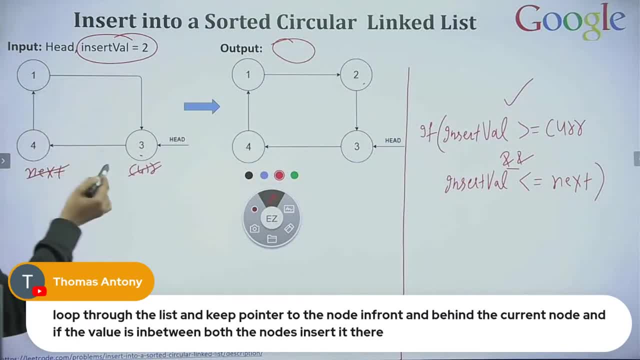 then i will not do anything. i'm just finding the place where i need to insert these two. so what i'm doing? making this as a current and this as a next node, just taking two pointers, which is pointing to- earlier they were pointing from here and here. now, here and here move one step forward. 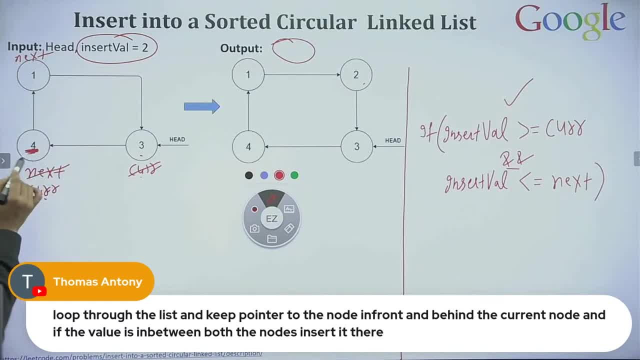 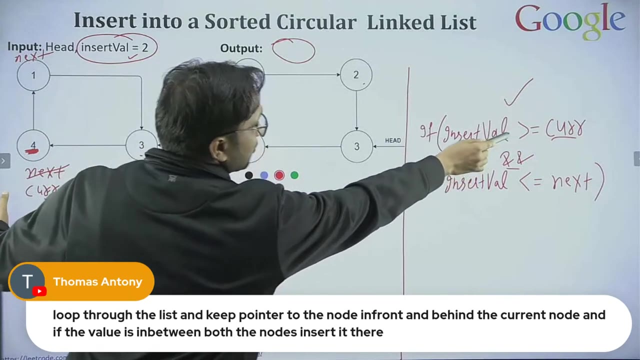 again we are finding: is this value is? is this value is smaller than my insert value? no, two is greater than four, not smaller than four. two, two is smaller than four, not greater than four. so current value is not, is not smaller than the insert value. again, we, what we will do, we will. 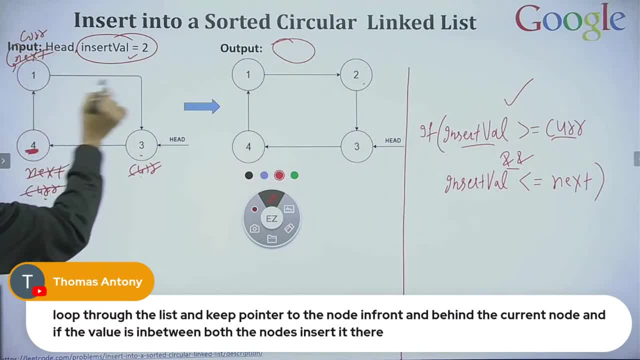 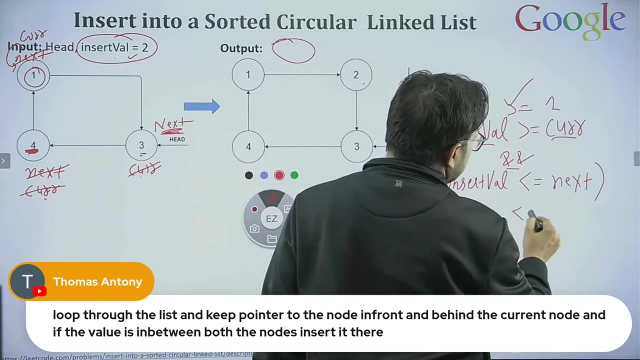 make it as a current, current node and the next node is this one, this as the next node. fine, again we are asking: is this value, is the current value is smaller than two? yes, and is the current value? is the next value is greater than the? is greater than this? let me check. yes, that is greater. 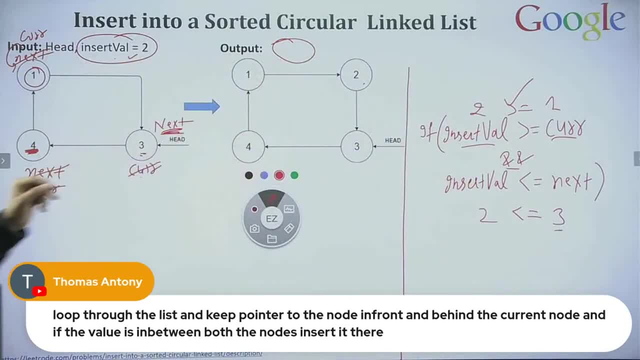 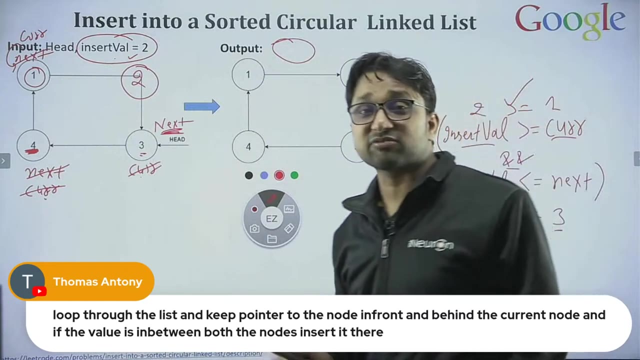 so both conditions are satisfying. so we find a place. we find a place where we need to insert the value. we find a place where we need to insert the value, but you okay, for almost all the cases. this is working for almost all the cases. i'm saying almost. 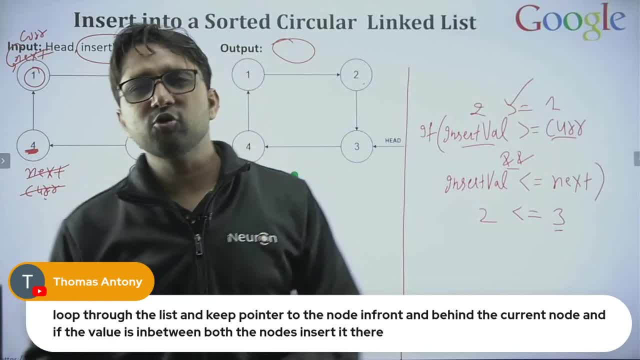 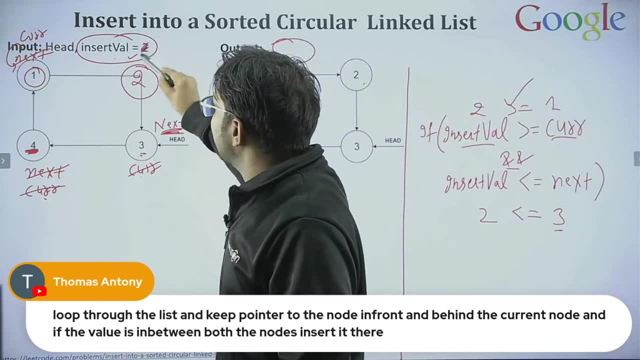 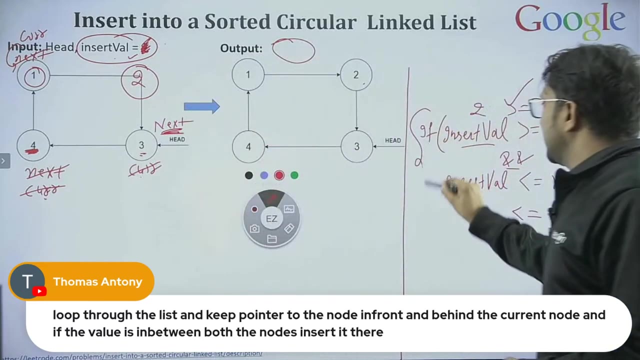 but still that will be failing somewhere. can you identify where this condition will fail? can? can you give me some value? can you give me some value? which i insert, which i insert and this logic will not work, then this logic will not work actually, and this logic will not work actually. 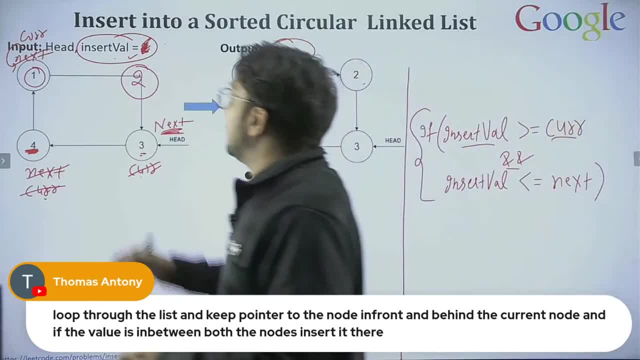 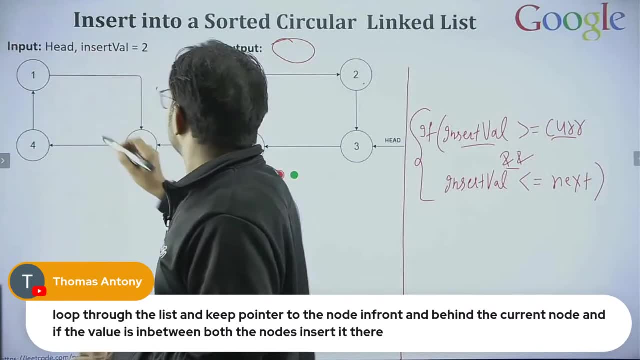 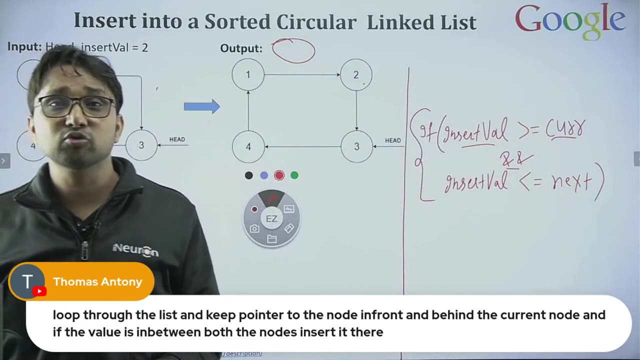 anybody, anybody can give me, can tell me what value should i insert in this link list so that my this logic get failed. what value we should insert? can the node have duplicate values? yes, thomas, nodes can have duplicate values. on decreasing order: what do you mean by non-decreasing? what it's: a non-decreasing value. we encode it into the value for nodes, but with the help of. We know that a chick coin will not be able to recover in the wheatまた, but it will be capable of keeping a loyal quantity of worth cooked sentiment compared to what is happening. we know that a arm is going to be on the plate, what that means, which means that there we have not able to solve, but people gave, along with the Ambata that we created, dziaramuchi or whoever else is using another first generation globalization in the system. 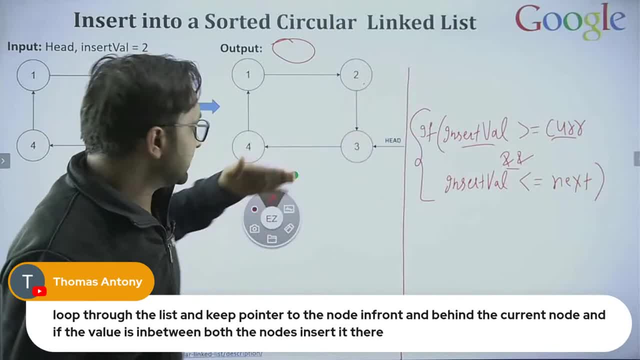 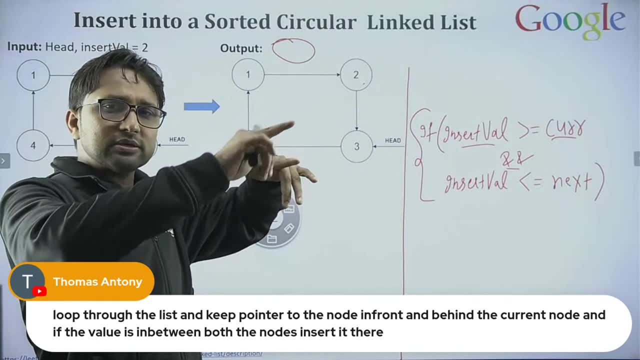 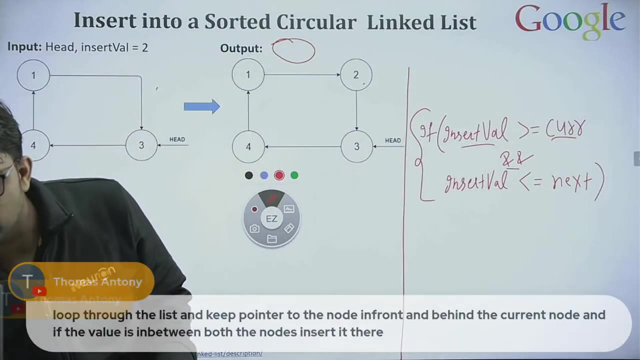 can-do not-vale to this same structure, which is correct for this order. what do you mean by non decreasing? that is, in increasing order and not only increasing. the value can also be same. the value can also be same. so, yes, duplicate values are allowed. so, Thomas, give the answer to this. so let 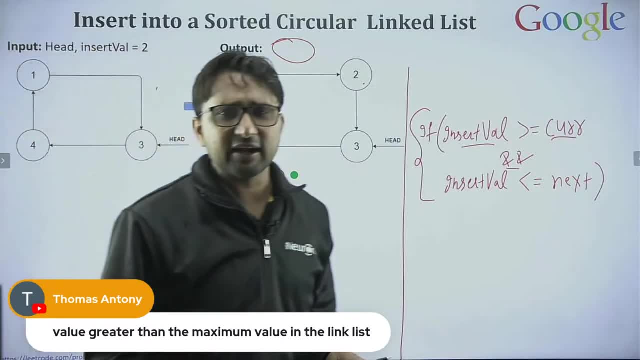 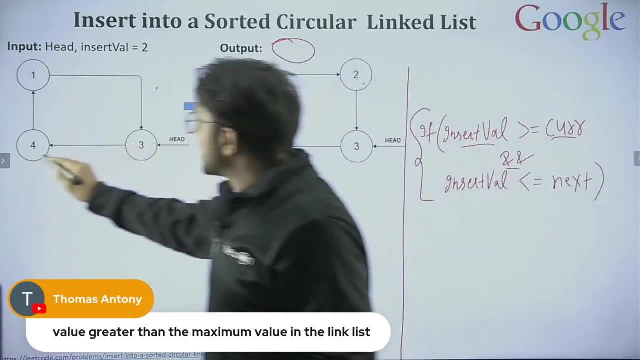 me highlight this thing: Thomas say is saying that take the value greater than the maximum value in the list, then this logic will fail. so let me take maximum values 4. I am taking 5. I'm taking 5. let me check if my condition first of all, if 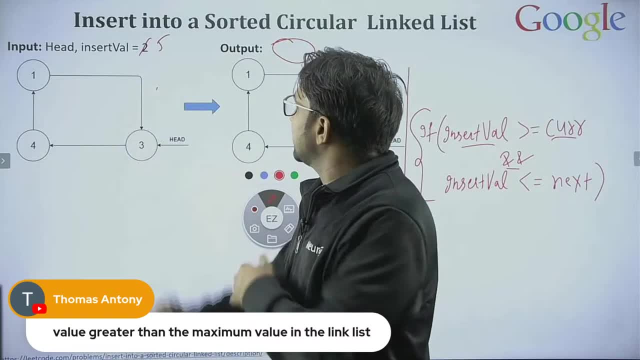 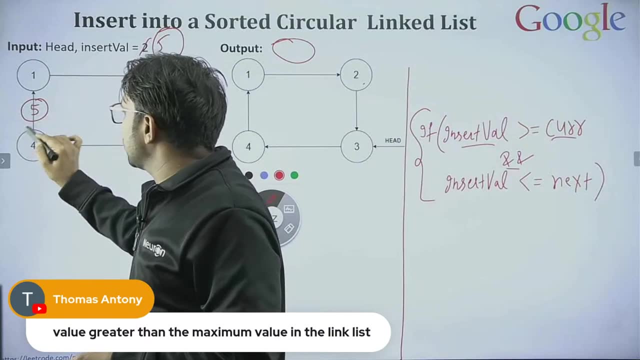 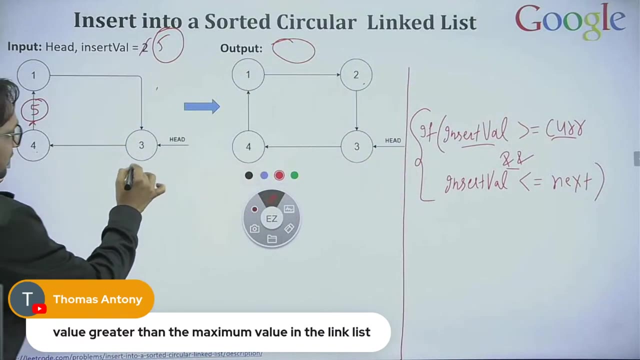 I see over here where the node will be inserted. this node will be inserted. so this node should be inserted after 4 here. this should be inserted after here at this place. so if I start, let me try this logic. this is my current node. this is my next node. I'm checking, I'm checking the. 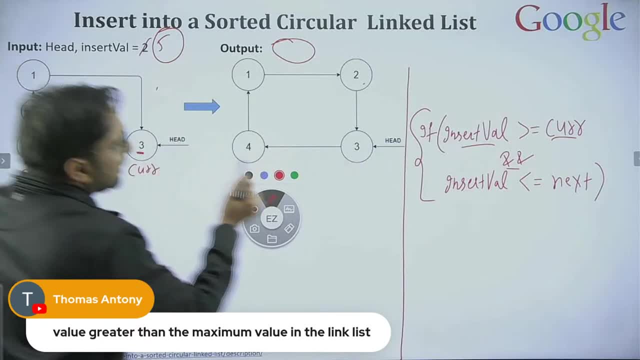 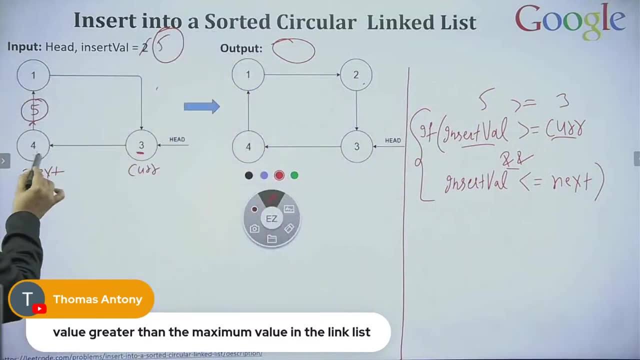 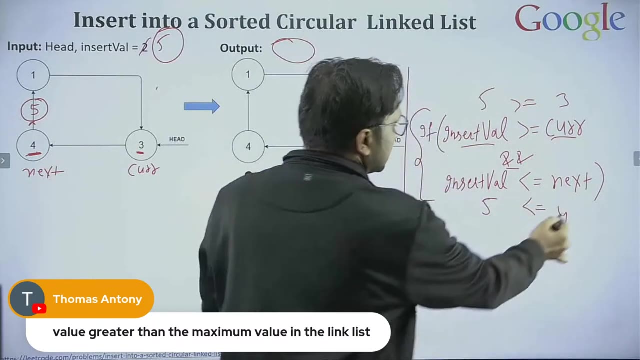 condition. is the condition satisfying? no 3: 3 is not smaller. yeah, that is smaller than 5. this condition is satisfying. sorry, and what about 4? so is the 4? let me write over here: is the 4 greater than equal to 5? no, so this one. 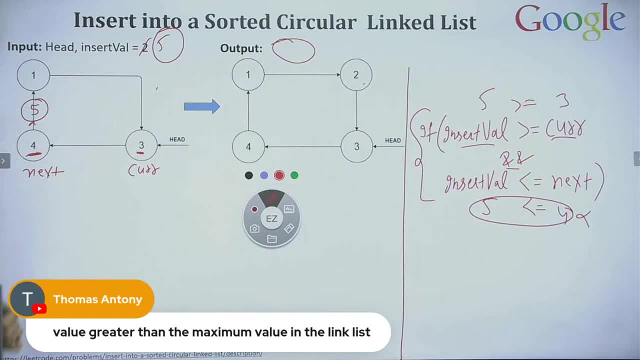 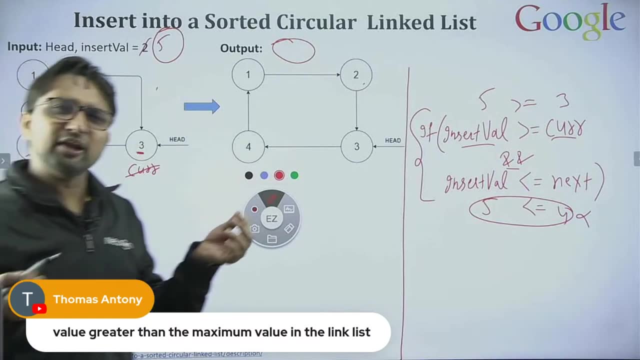 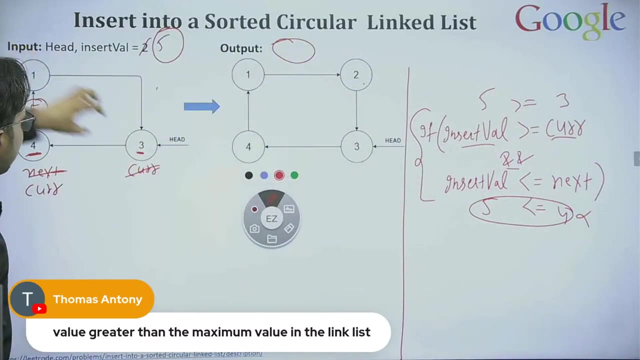 condition is failing. this time because one condition is failing, what we will do? we will increment. this will be our current. we are just checking two nodes. which is satisfying this condition? okay means one value should be smaller, one value should be greater than in between. we will insert: may be equal also. that's. 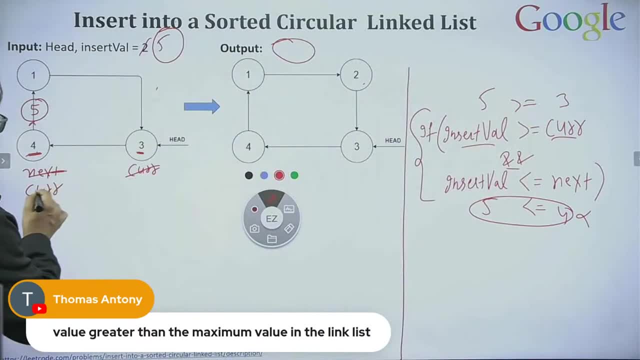 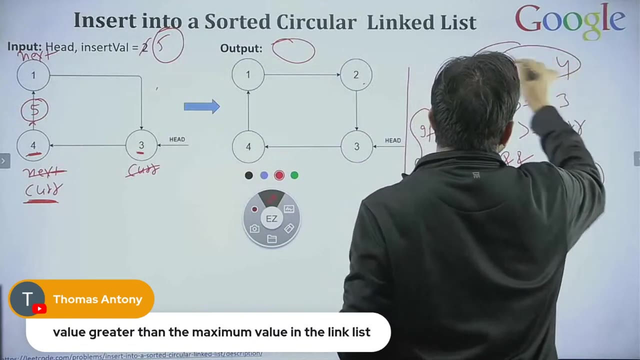 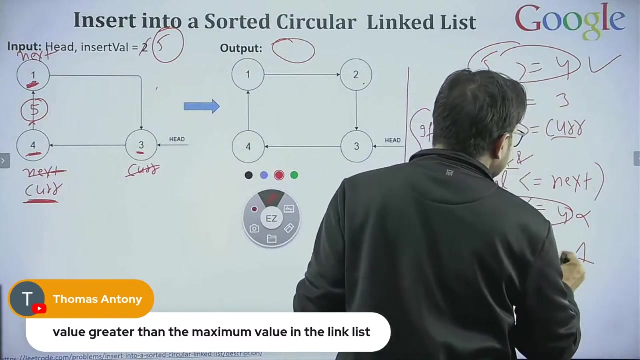 why we write equal also that that is also working. so this is current. this is next. now let me check out if the condition is working or not. so current value is 4: is that is smaller than equal to 5? yes, the condition is satisfying. what here next value is 1. is that is greater than equal to 5? no, that is not greater. 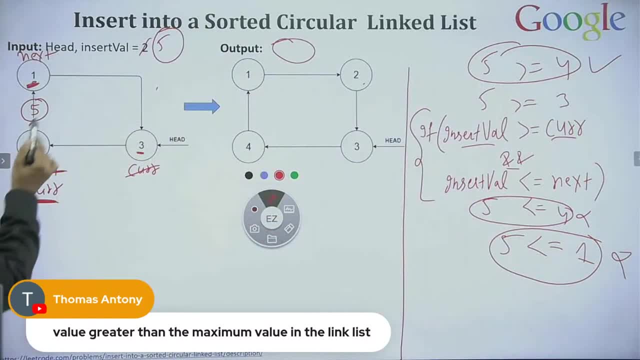 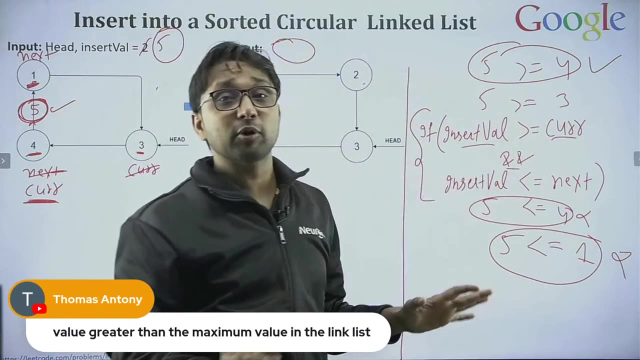 the condition is failing, we will move on, but we need to insert here. but we need to insert here. we cannot move on, we need to insert here. so, for 5, using this, using these statements, we are not able to find out the place where we need to insert the. 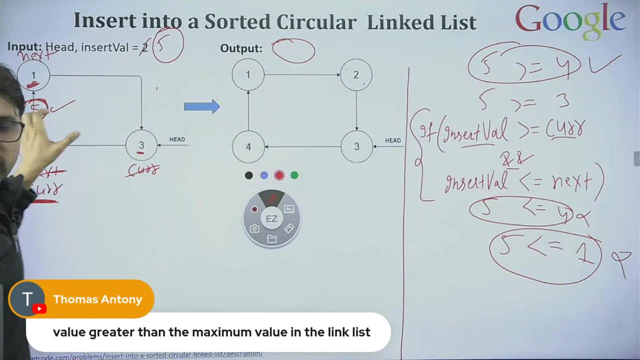 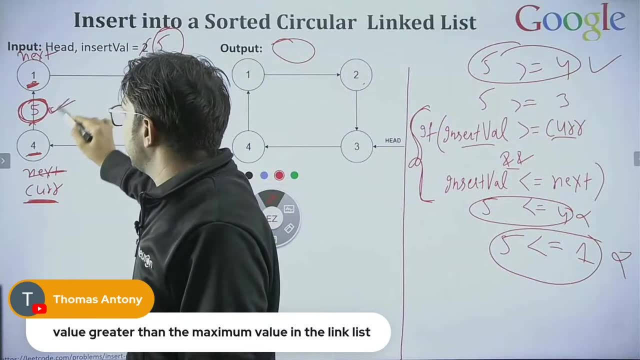 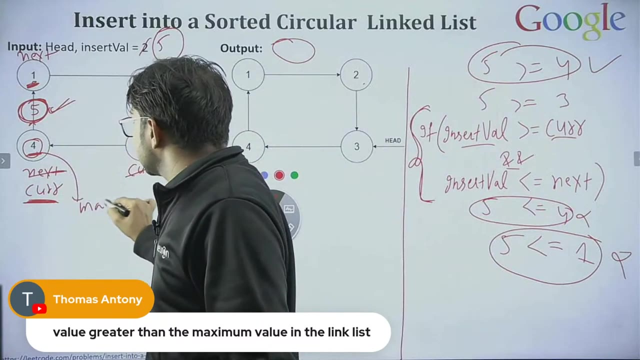 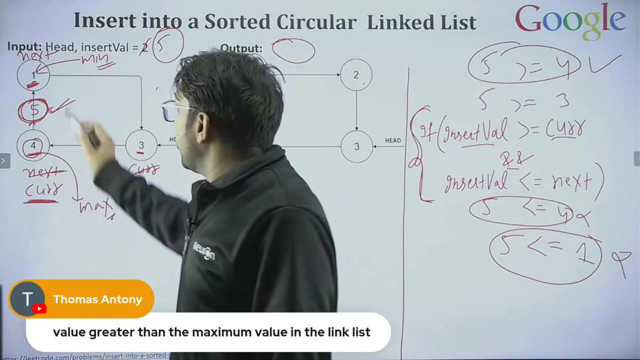 pipe. okay, so this is one exception, actually this one exception. otherwise this condition will work everywhere, except this place. only what this place is, this is the place between the highest value, maximum value and minimum value. this is the place between maximum and minimum value. so, except this place everywhere. 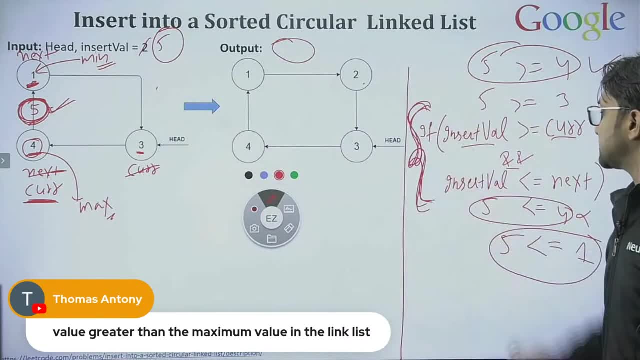 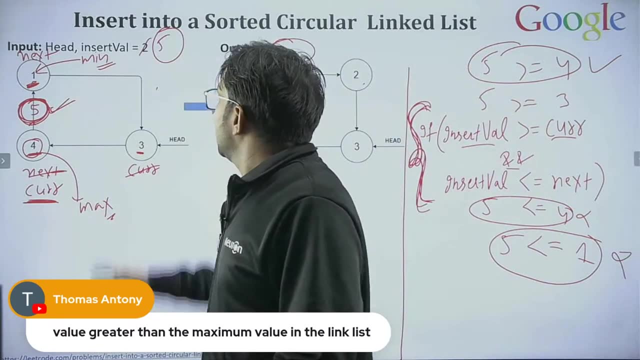 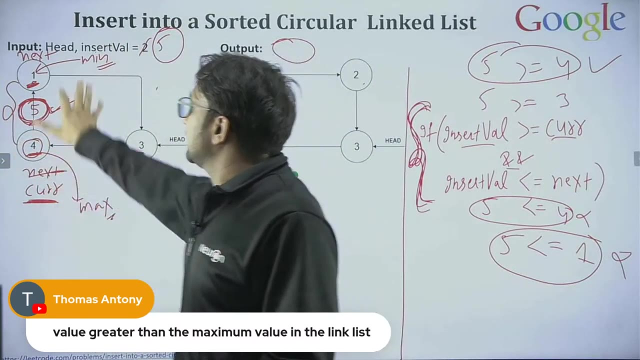 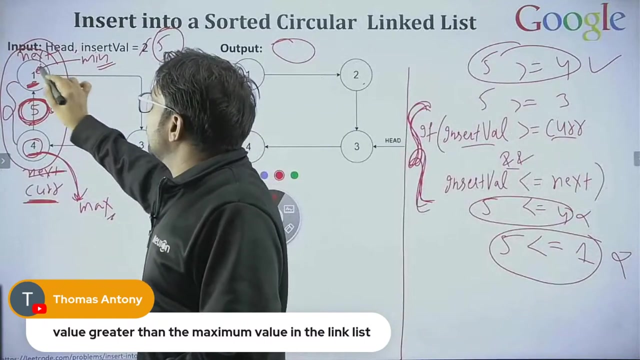 this condition will work perfectly. you can, you can, you can notice this thing everywhere. this condition will work. so now the question is how you will handle this condition, how you will handle this condition, how you will identify this condition where you have a max value and you have a min value. you have a max value and you have a main value. any doubt, please ask. 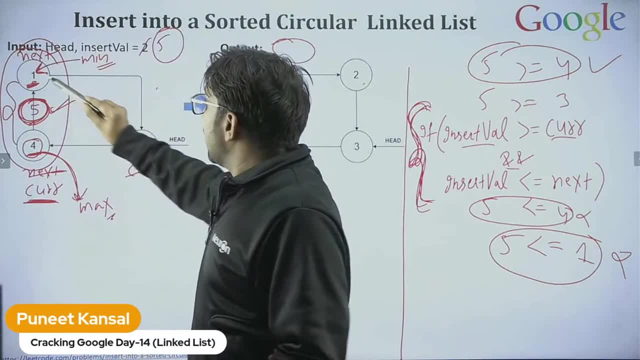 any doubt, please ask. otherwise let me know in the comments section. so so that's it, guys. very much, i hope it was useful and thank you very much for watching today and i will see you in the next place. bye, bye me. know what condition I have to write so that I can identify that? okay, this is the maximum value. 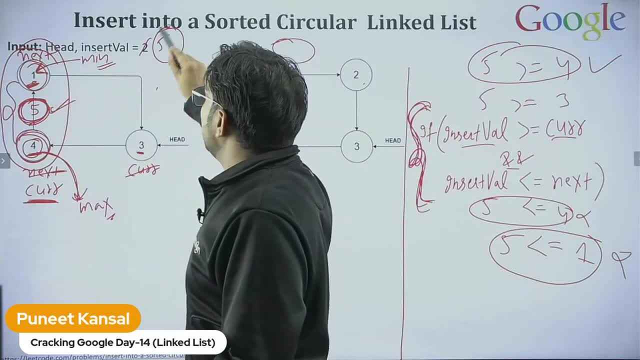 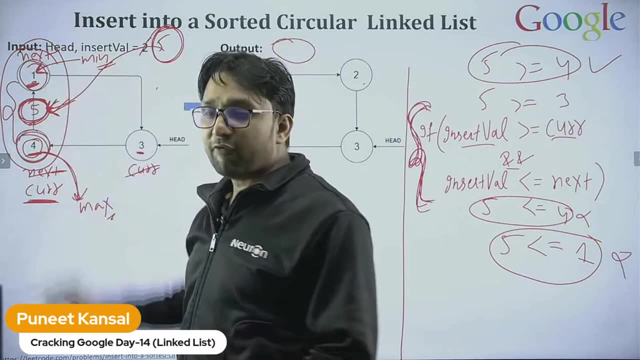 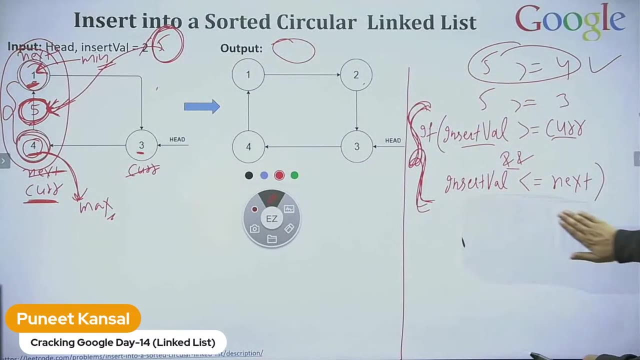 in the linked list and this is the minimum value and the value which we need to insert. that should be inserted over here. that should be inserted for finding this thing, what condition I have to write? what condition I have to write? any idea from you people's side, any idea? please think and reply. 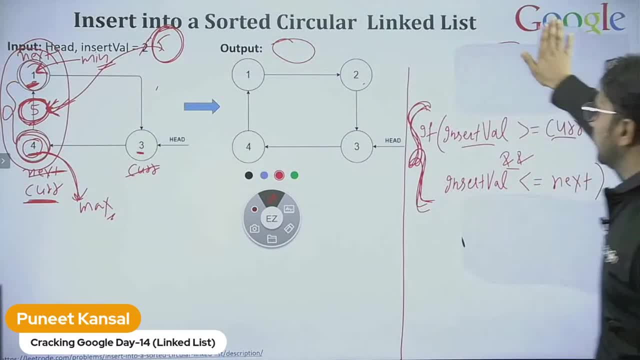 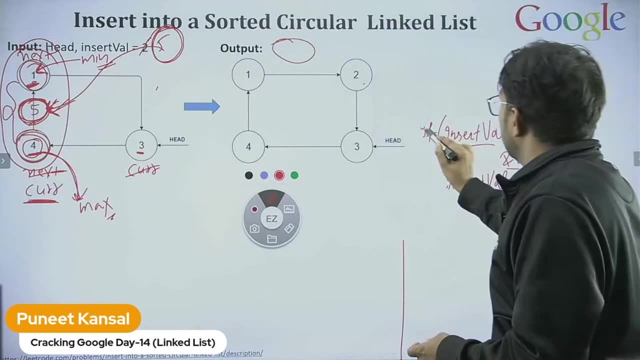 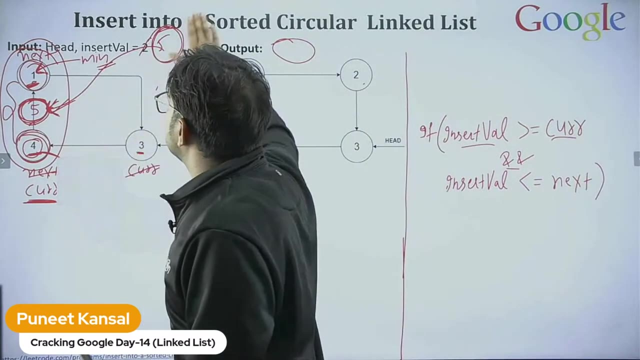 that is important. if you are thinking or not, that is the only way to master the DSA. that is the only way, if you are thinking or not. there is no other way. if somebody is saying that I will teach you directly, I will give you the DSA directly, they are lying, believe me. they are lying. there is no. 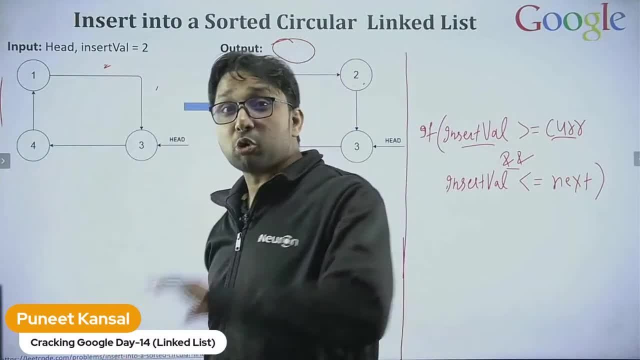 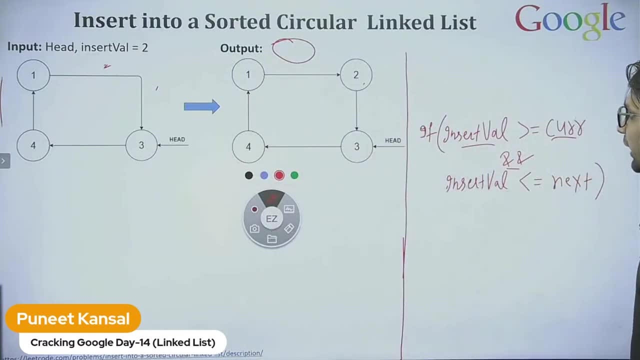 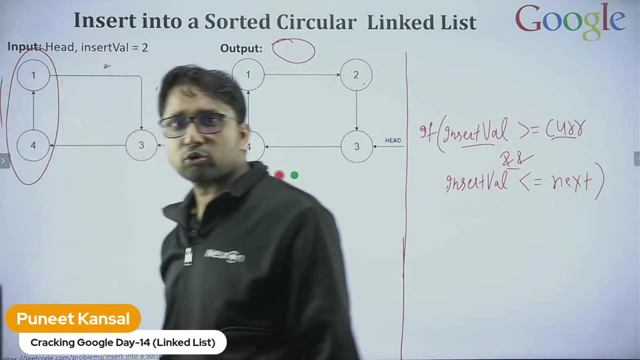 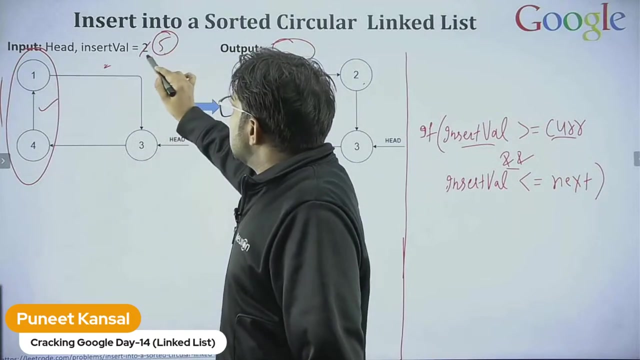 shortcut. there is no shortcut to math. there is no shortcut to learn the math, it's a math only. so please think and reply what condition I have to write so that I can find out this place. I can find out this place if some value is there which will be inserted in between these two. otherwise, otherwise, except this position. 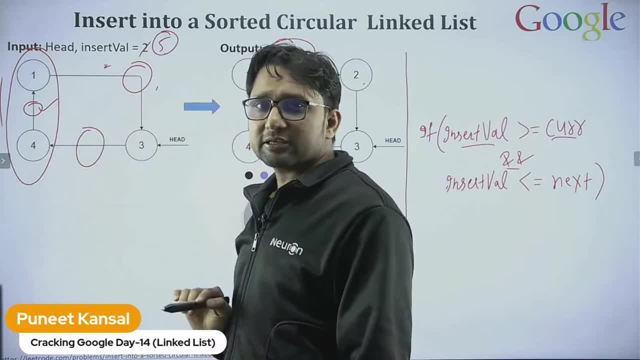 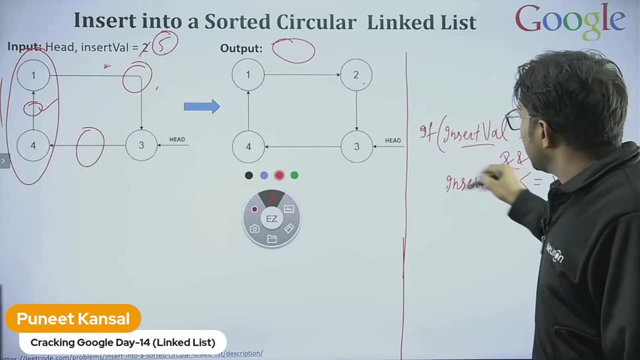 everywhere, wherever you insert in the linked list, wherever you insert, this condition will work very fine. so, okay, you can. maybe you can say that you can. otherwise, you can please check the link list and you can check the link list and you can check the link list and you can check the link list. 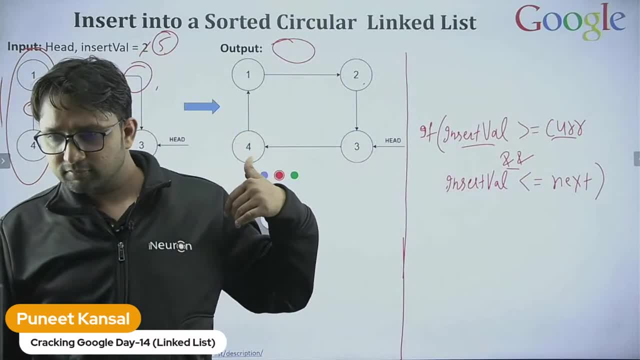 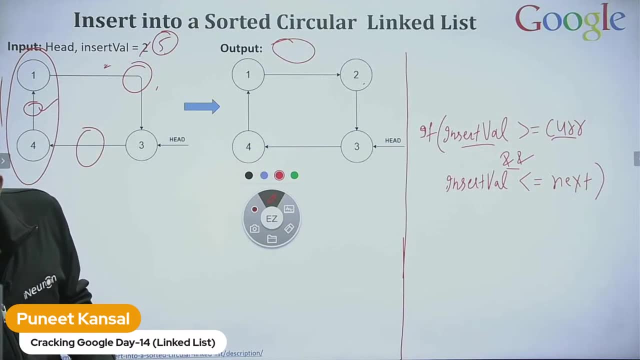 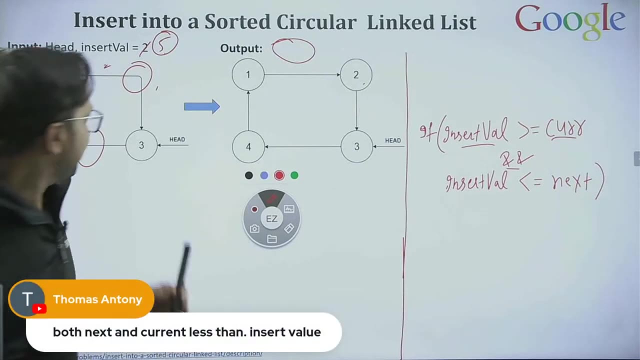 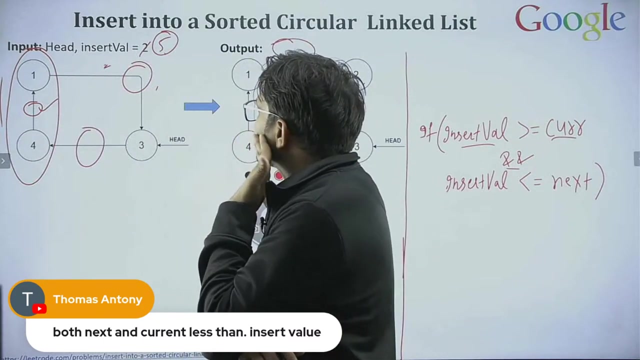 out this what I'm telling you. so there is a one reply from the Thomas. let me take that first. both next and current less than insert value. so Thomas is saying: okay, if both are smaller, let me try to fail Thomas, this condition. maybe I can. maybe I can try. you're saying that if both are, both are less. 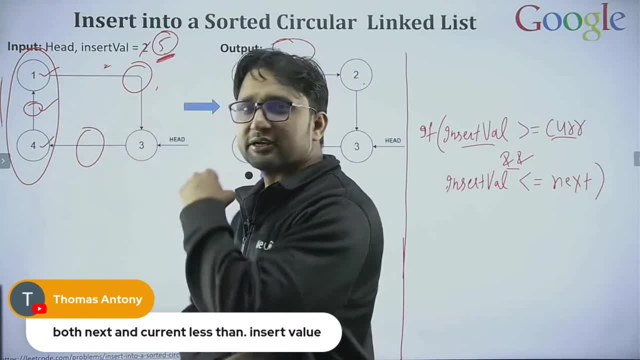 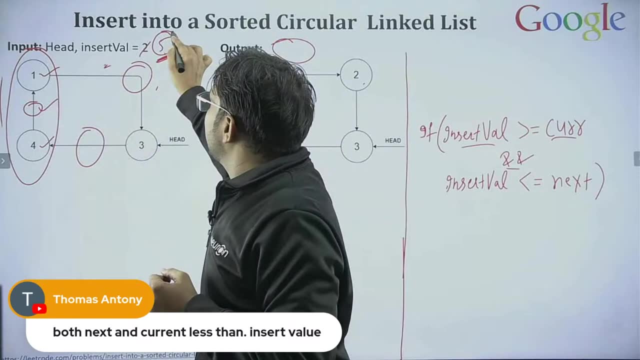 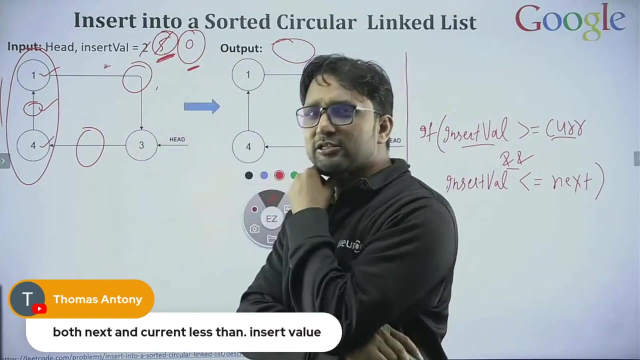 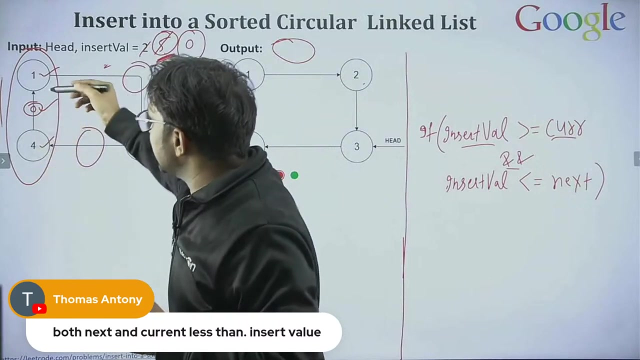 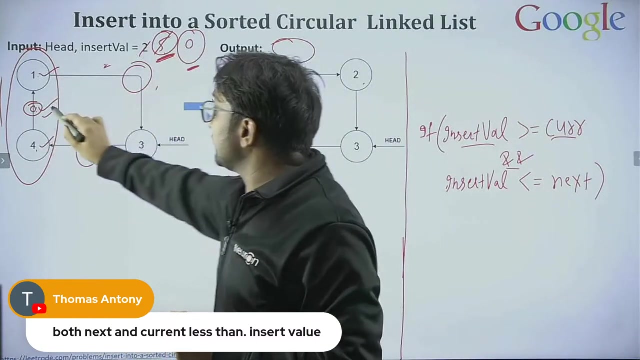 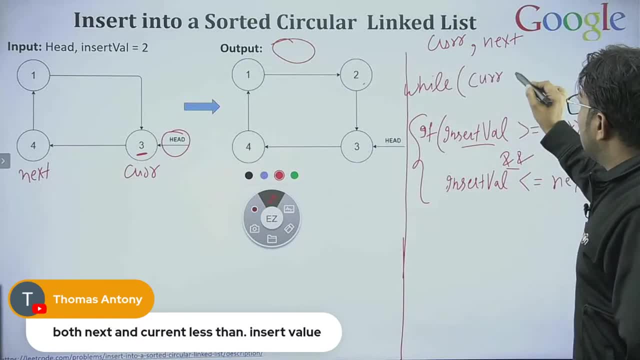 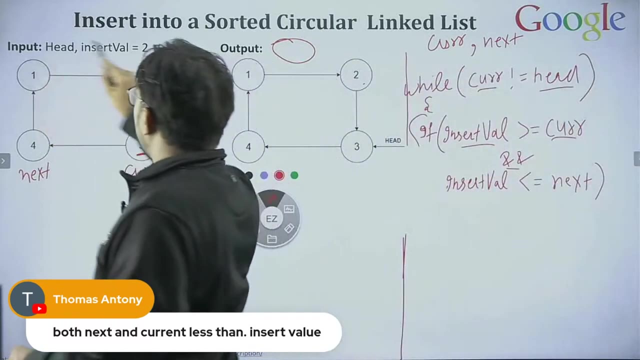 I'm checking. okay, if my current, until my current is not equal to head, I'm. I'm checking this condition again and again. I'm checking this condition again and again. until my current will not become, I'm coming back to the head again, I'm coming back to the head. I will keep. 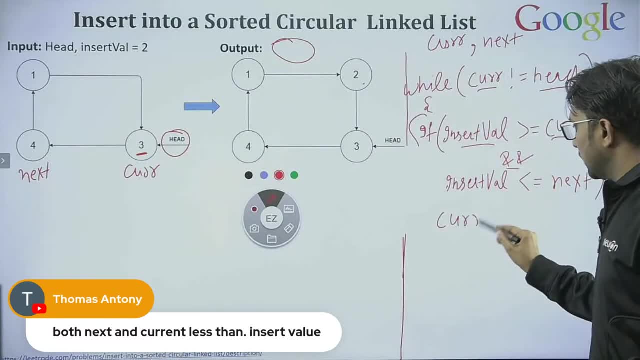 checking this condition, let me update my current also. current will be become the next if this condition is not satisfying. if this condition is not satisfying, then we will update our current. current will be the next element, current will point to the next and what will be the next? 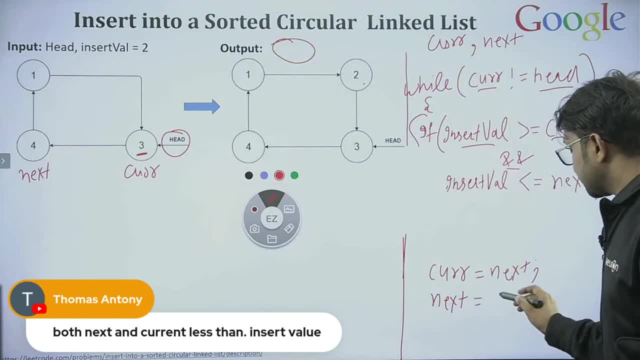 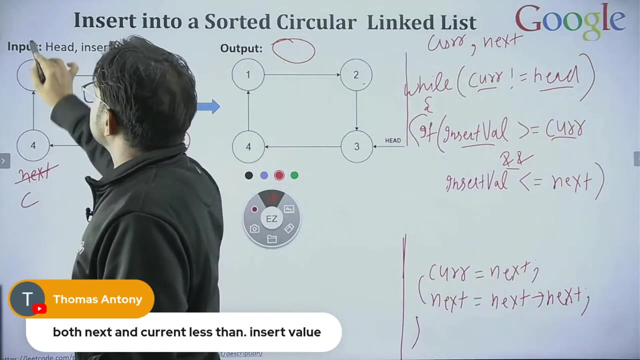 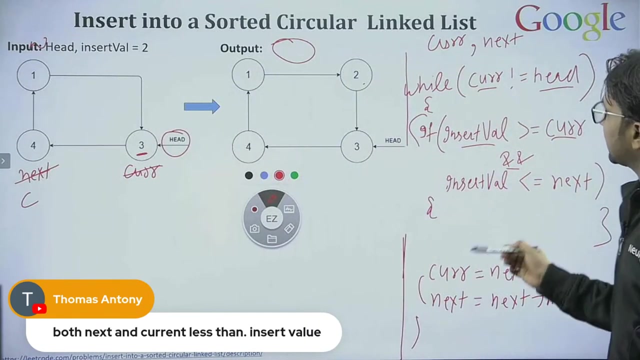 next will be, next will be next of next, next of next. fine, so we need to. we- I'm updating these two- means: next of next, then current will become this and next will become this. keep doing this thing until unless this condition is not satisfying. if this condition is satisfied, then we can insert our. let's suppose 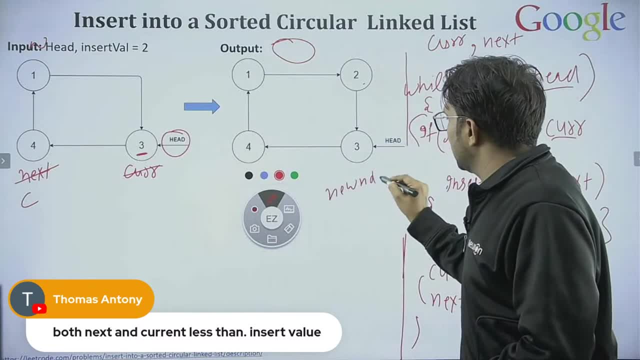 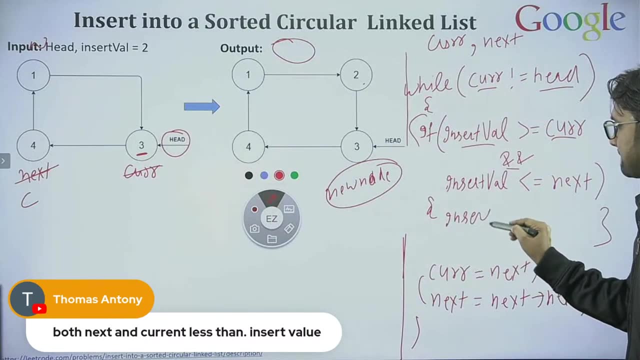 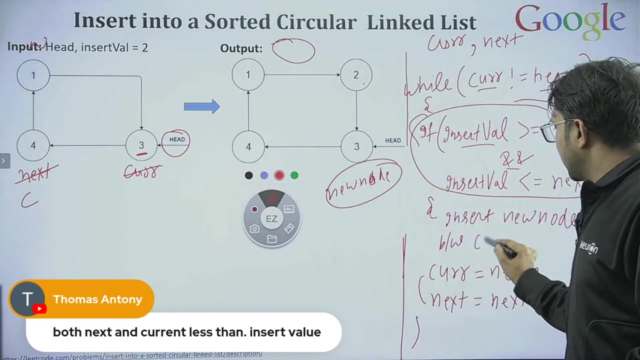 new node. here is the new node, new node, new node. so this new node we can insert just simply. I can write: okay, insert new node, insert new node. that's it. so if this condition satisfy, we can insert new node in between current, in between in between current and current and next. that's it. so if this 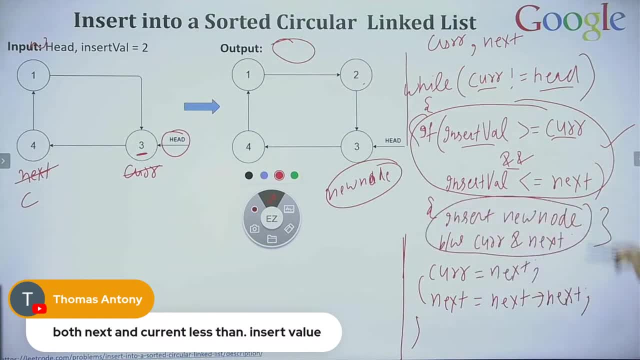 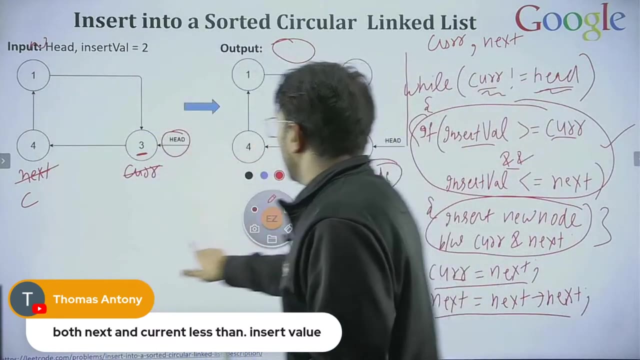 condition satisfied, we will insert the node between current and next. otherwise we will keep incrementing current and next we will keep incrementing them until, unless our current is current is not equal to head, we will going through inside the loop. we are going inside the loop, but we 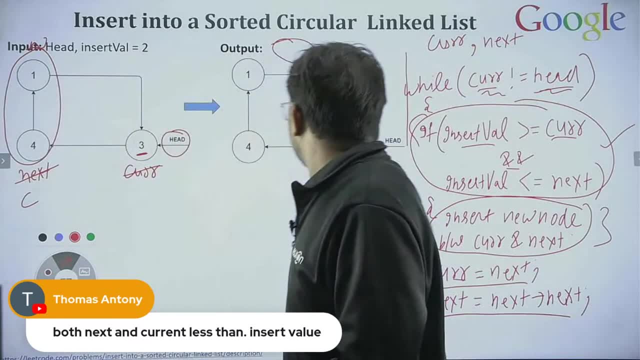 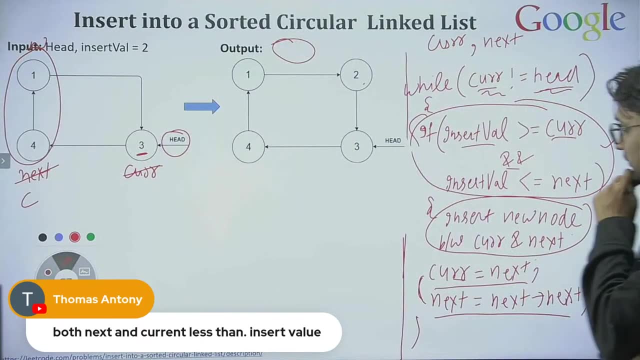 do not handle this condition, but we do not handle this condition over here. for that, okay, can I say this thing? and let me add one more thing over here: what? what I can do is what I can do if, after going through this loop, if, after going through this loop, after coming back to the 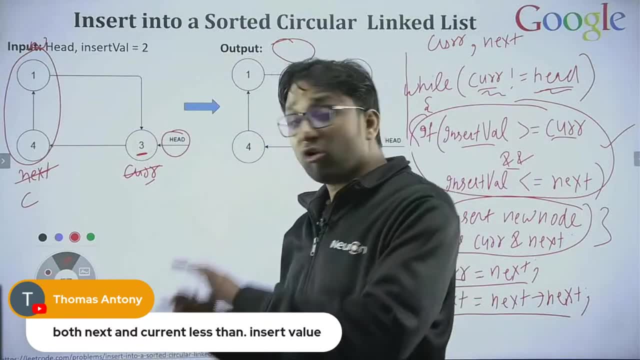 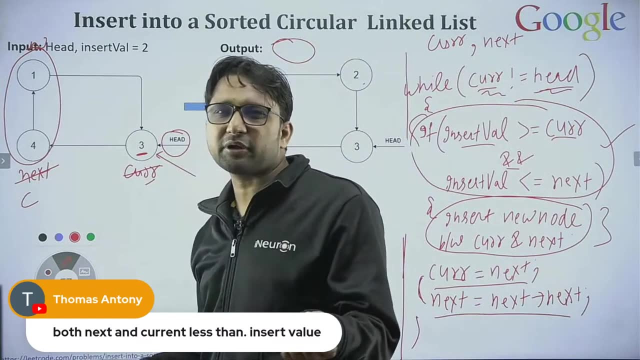 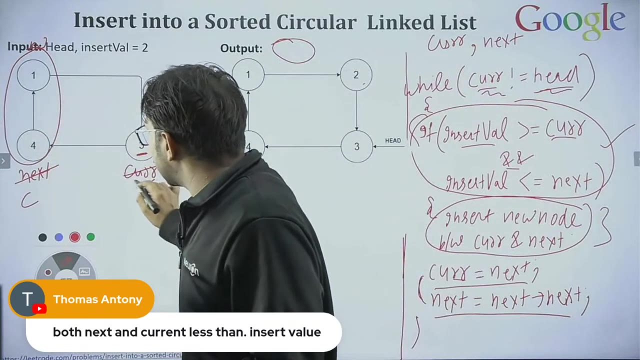 current. after coming back to the current, if I don't find any place- see listen carefully- if I started from here- last thing, actually last important thing here- if I started here, if I started from here- and I am checking again: current and next, current and next current. 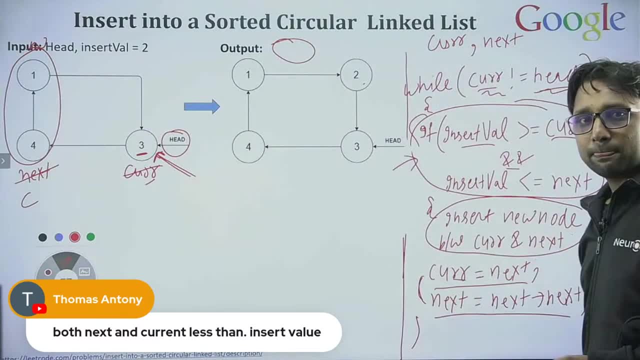 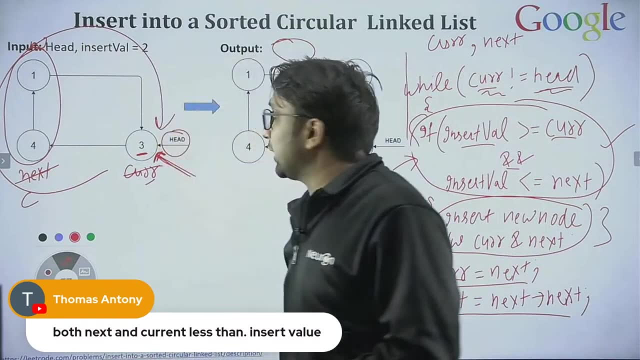 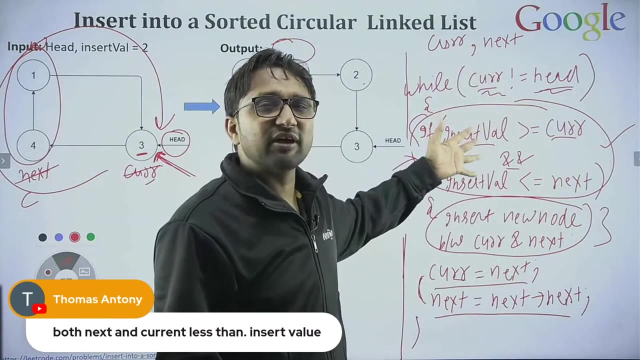 and next, and checking this condition every time you put. you please reply, starting from head, coming back to head again, coming back to head again, but don't find any one, any two nodes. I don't find which is satisfying this condition. which is satisfying this condition. 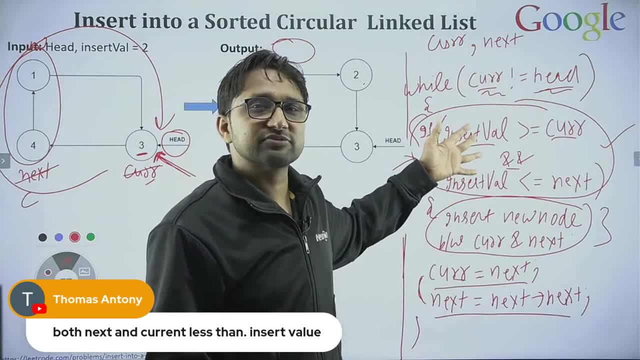 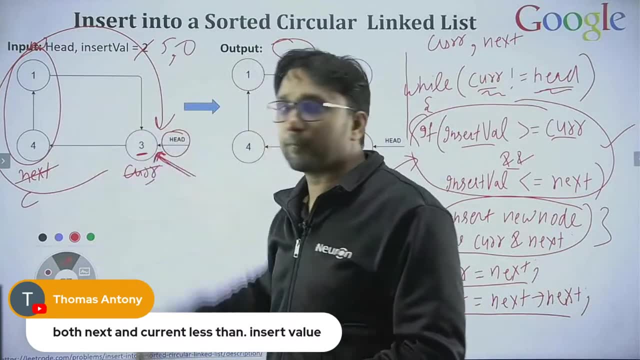 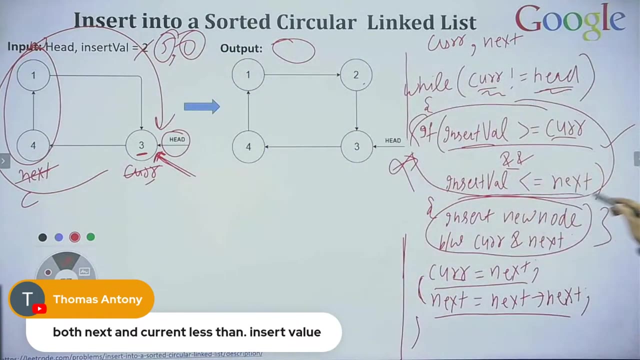 and what that means is where I have to insert this value. If I for any value- let's suppose for five or maybe zero in this particular example- any value, these two value, you know that will not satisfy these two conditions, will know every time they will fail these 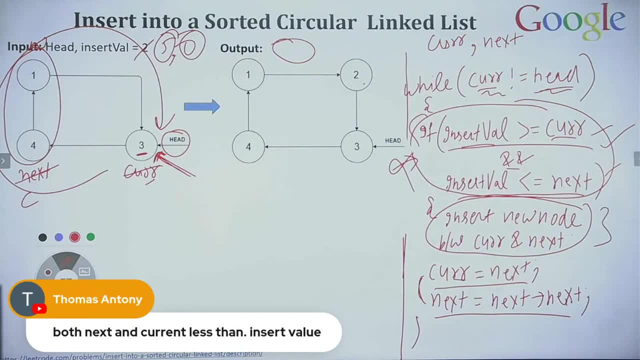 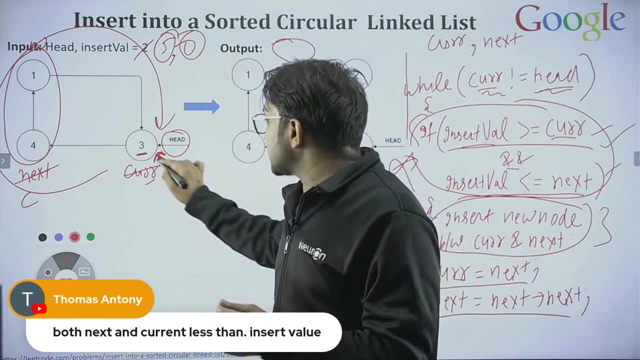 two, either this one or this one, they will fail one condition. So can I say this thing? that Can I say one? can I make one statement? I chop, started from here and going through all the nodes, come back to here, but I don't find. 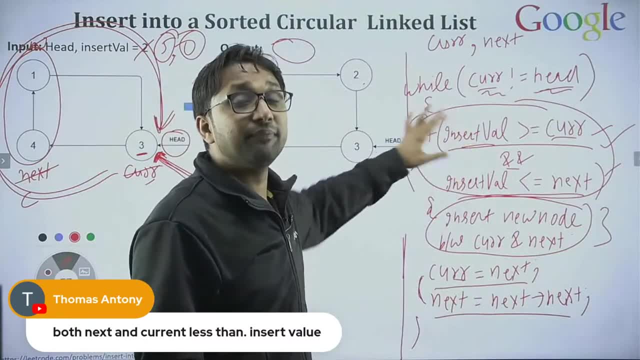 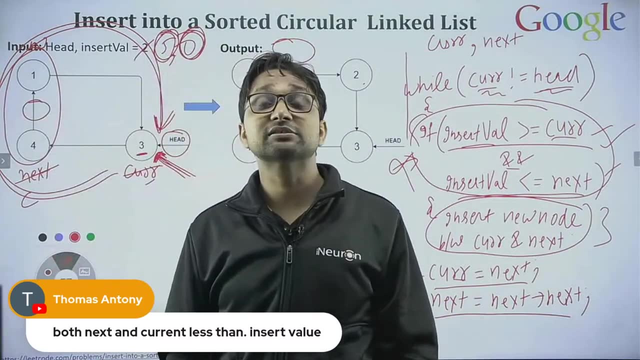 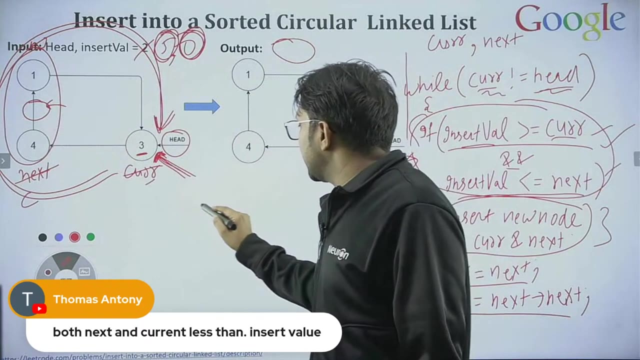 any two nodes which are satisfying these two conditions, then definitely, whatever is the value over here, whatever that will be inserted here, only that will be inserted here only. So, after coming out of the loop, I, we can directly insert between, we can insert we. 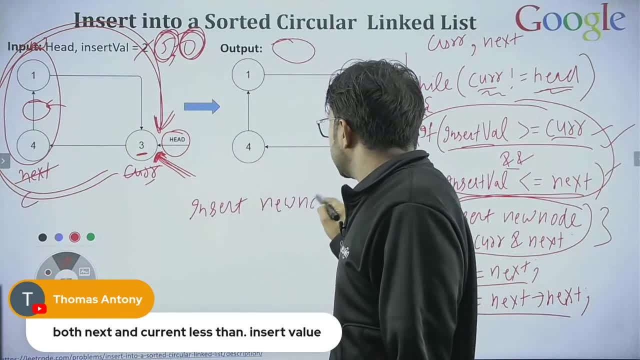 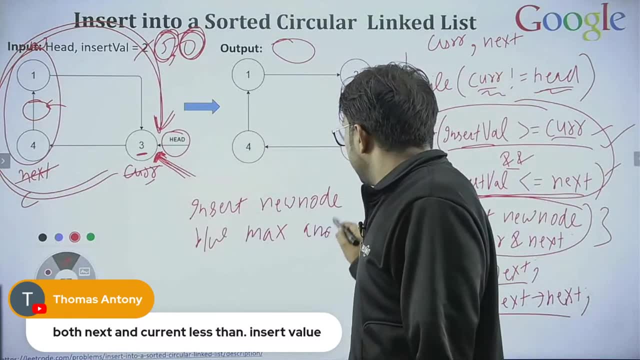 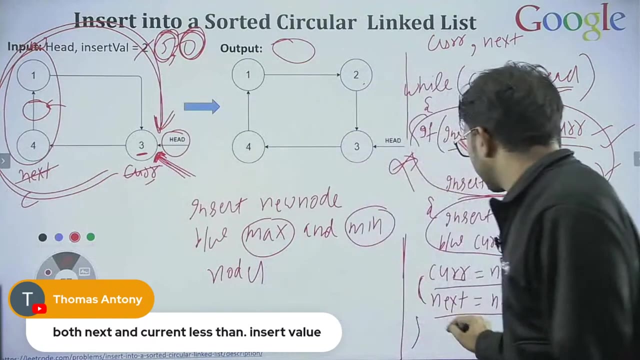 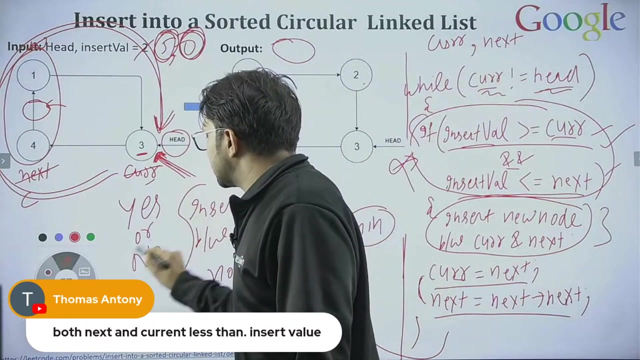 can insert new node. we can insert new node between between max, max and max and minimum value, max and min nodes. After coming out of the loop, can I make this statement? Please write yes or no. Please write yes or no in the chat section. Please write. Please reply. 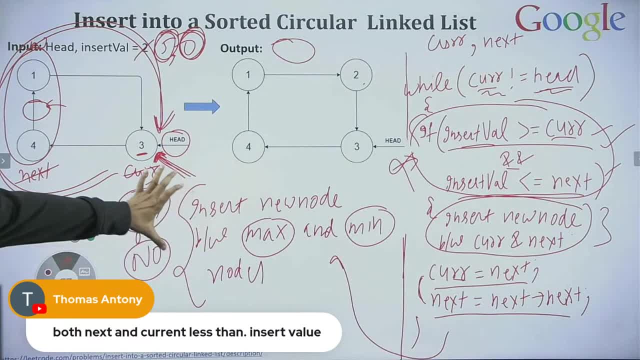 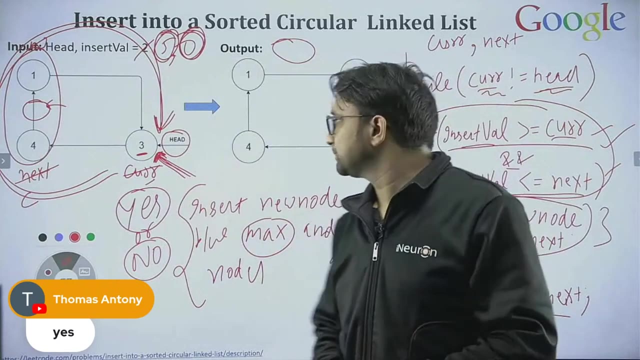 Anybody? please reply this. Are you able to understand what I'm saying? Please reply Okay. Thomas is saying yes. What about other people? Please reply Okay. I'm repeating this thing again. I'm repeating this thing again, Simple. The idea is this: I'm going 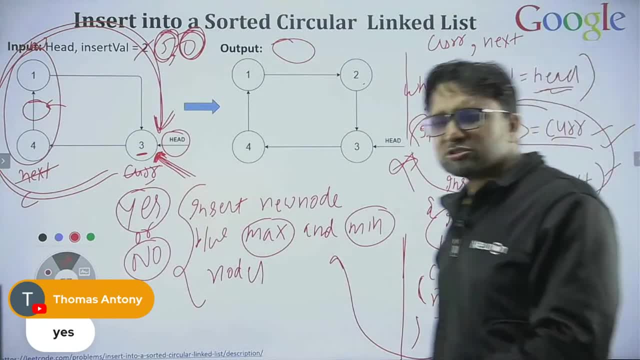 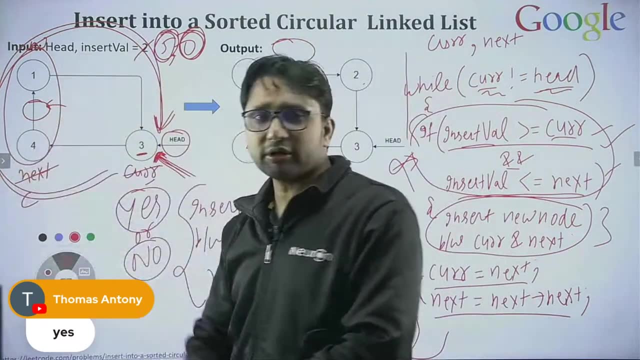 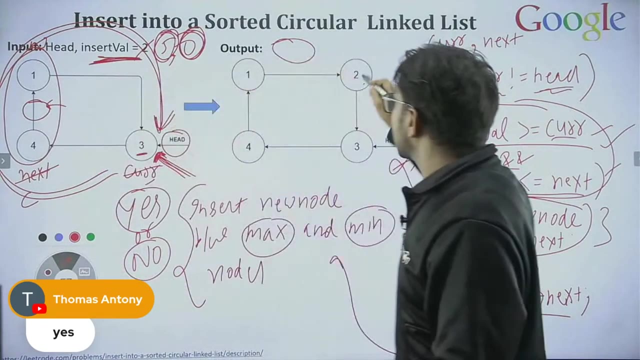 through the complete code. Now, actually the question is like that, starting from the question- let's suppose the question is like that- They provide us the sorted, sorted linked list. They ask us to add a node such that after addition of that node, the linked list remains sorted still. Okay, the linked list. 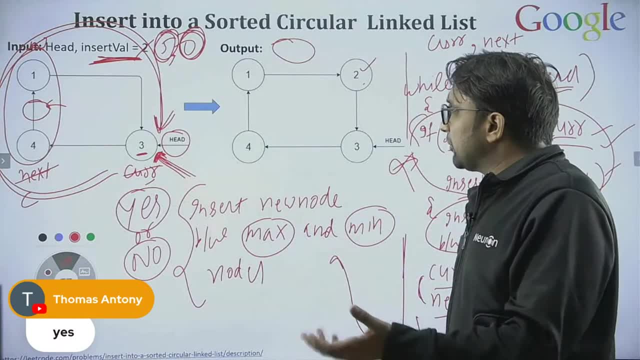 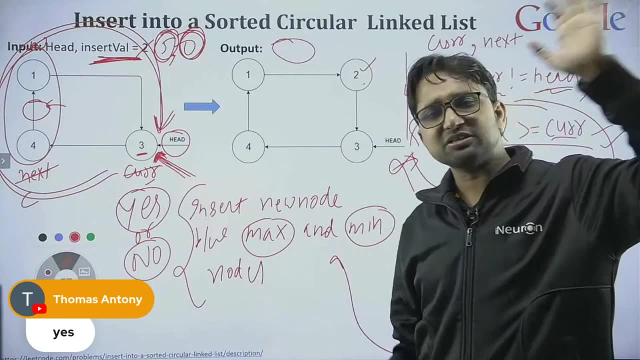 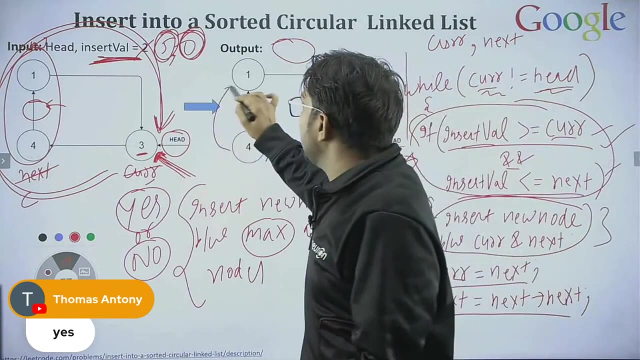 is still sorted only. So what can be the approach? The approach can be: see. this is the linked list. you cannot jump directly to any node. one thing is sure: you cannot jump directly to any node. you need to go node by node only. you need to go node by node. you need to check node. 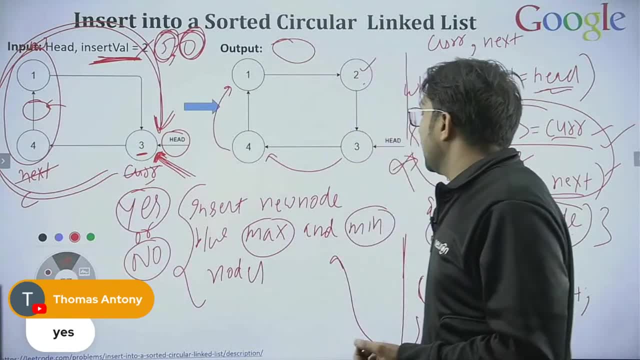 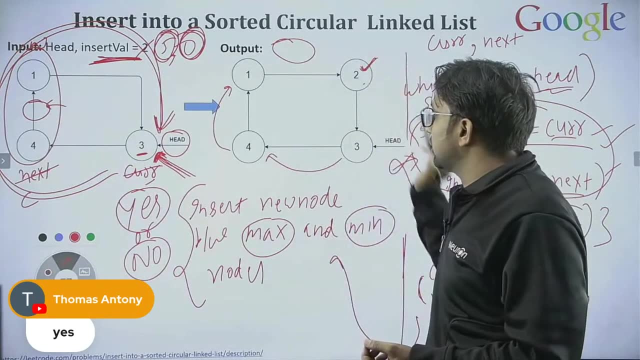 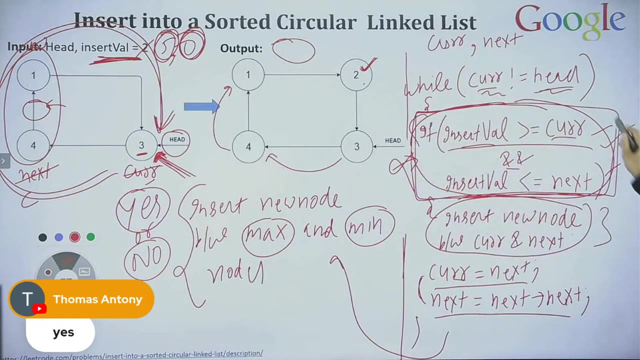 by node on and how you are finding, how you are finding that where you will insert this node, How will find that where to insert this node. So for that you find out that, okay, if this condition will satisfy, if this condition will satisfy, then you can insert the node. 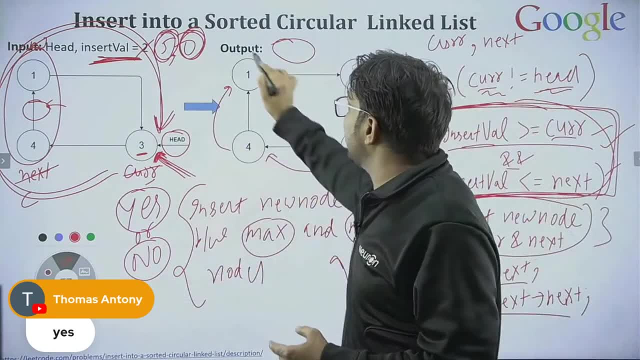 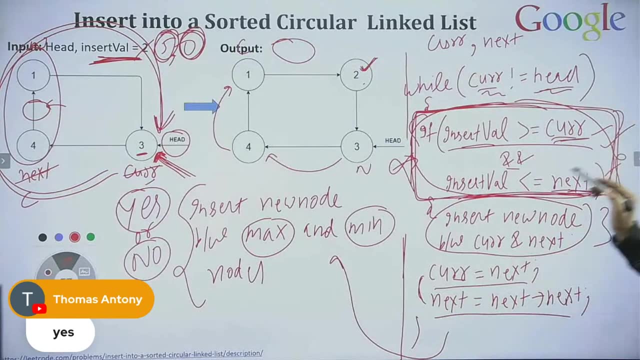 between current and next. You can insert the node between current and next. So next I'm current and next node. if current and next node, current and next node is satisfying this condition, then you can insert. so you are going to check every time, if not finding incrementing current. 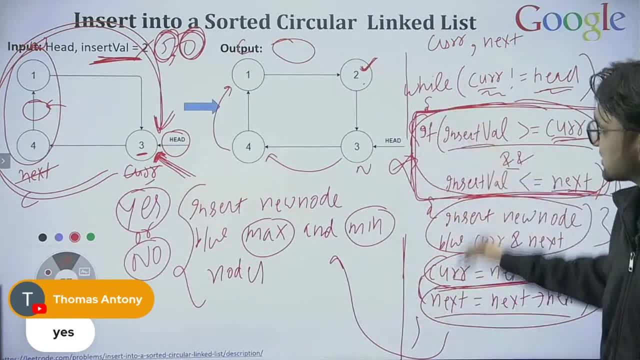 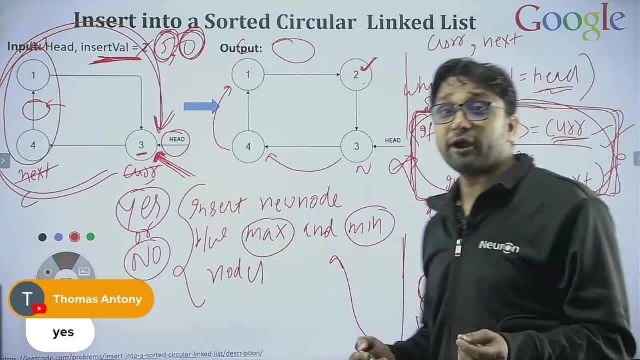 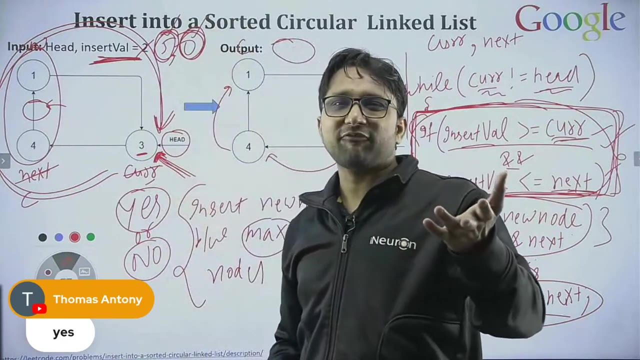 and next every time. okay, you are doing this stuff again and again, again. if you find out, you will insert that, that's it, we're done with that. but if you don't find, if you don't find, then sure that this is sure that, whatever is the node, there is only one place left. there is one condition: that 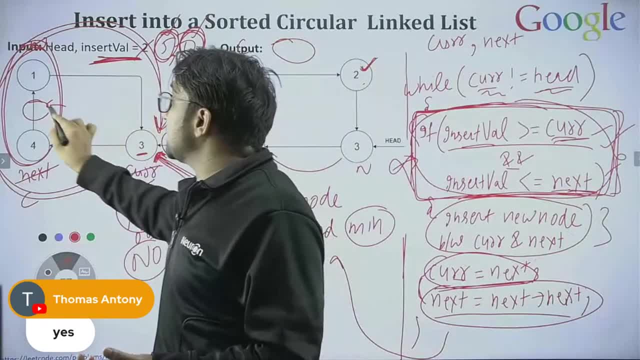 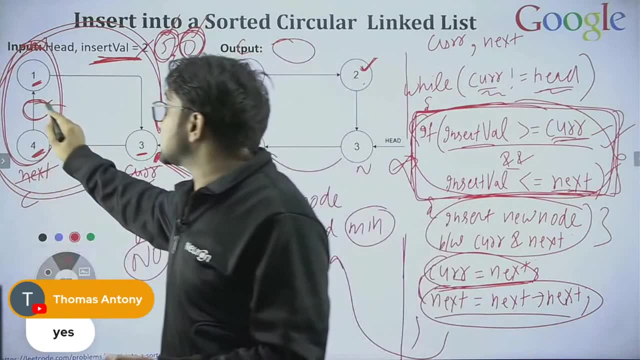 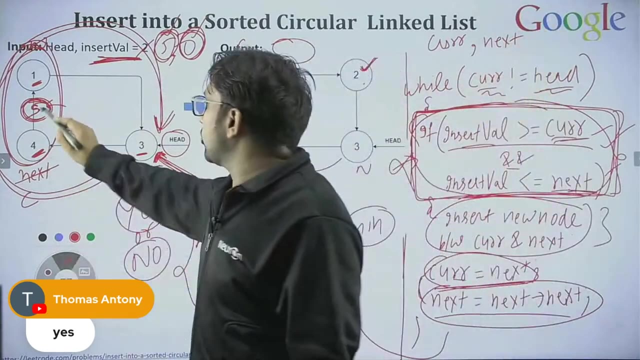 this one exception was left. that node must be inserted between the maximum value in the link list and minimum value. the node must be inserted over here. confirm. confirm. there is no other place. you have checked all other place. this is the only. for this you may write after coming out of the. 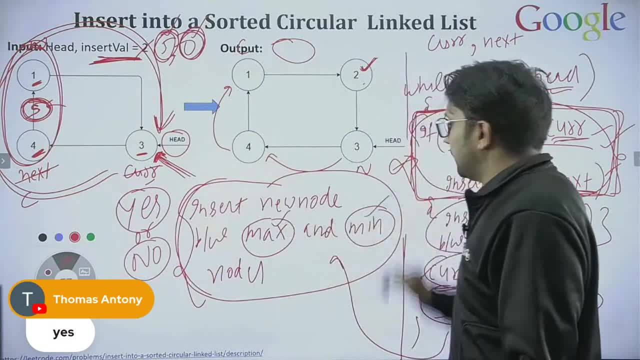 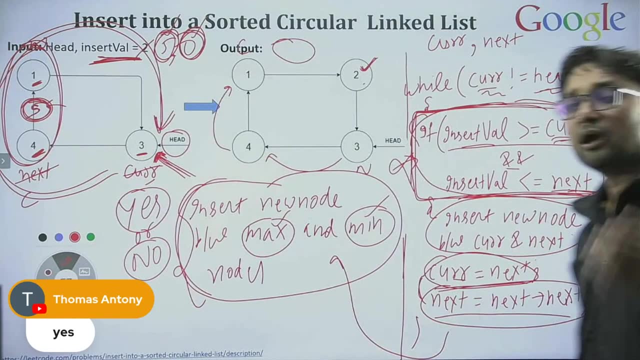 you can directly insert between max and min. you can directly insert between max and min. that's it. that's it. this is all about this. can you tell me how much time this logic will take to execute in worst case? what is the time? complexity, hello gangadhar. can you please tell me, gangadhar? can you please tell me how much? 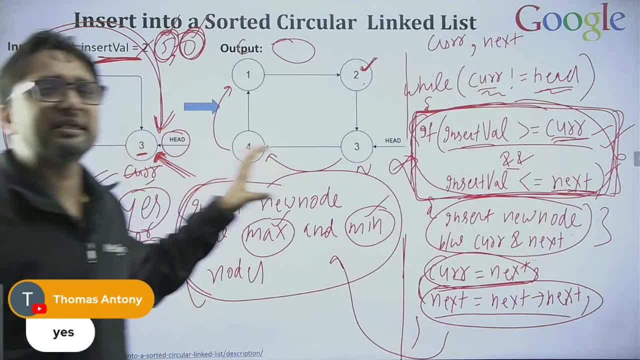 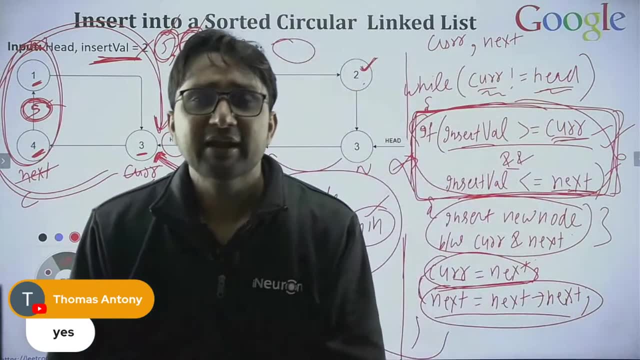 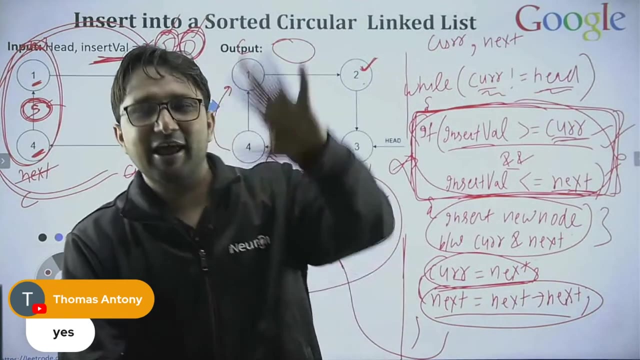 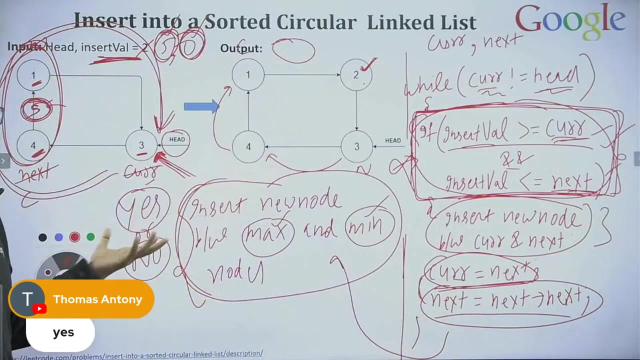 time this will take. can you please, can you people please reply and tell me how much time this will take, this logic will take. please reply whatever is coming to your mind, doesn't matter. the moment you will reply, learning will happen immediately. the learning will happen and that is required. please reply how much time this will take, right or wrong doesn't matter at. 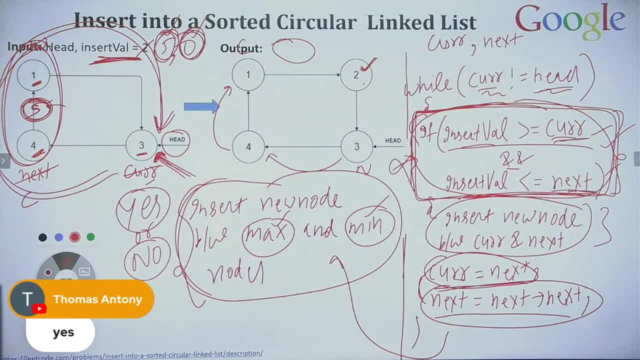 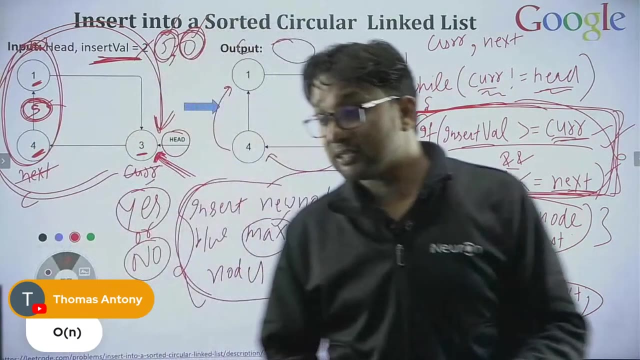 all. right or wrong doesn't matter. please reply how much time this will take to execute this code, this logic. in worst case, how much time this will take. thomas is saying order of n. thomas is saying order, and that is right. this will take order of n time. in worst case, you are starting from the head. 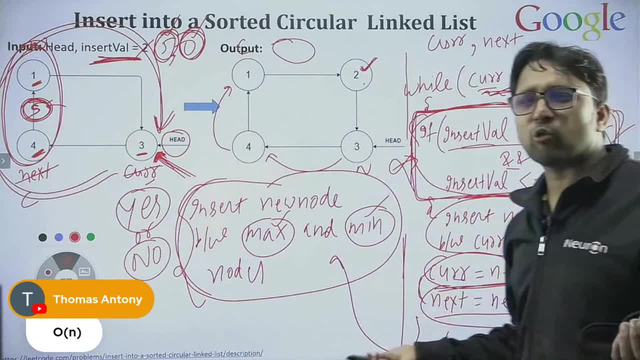 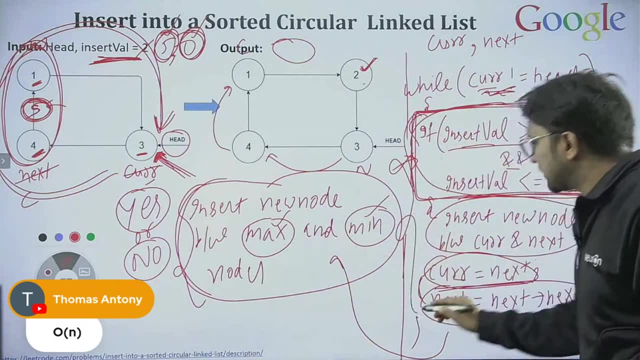 and coming back to the head, simply checking the loop, finding that complexity means finding how many time the loop is executing doesn't. doesn't matter how many statements i have written over here- 1, 2, 3, 4, 5, 6 statement. i have written even 600 statement, i will write. 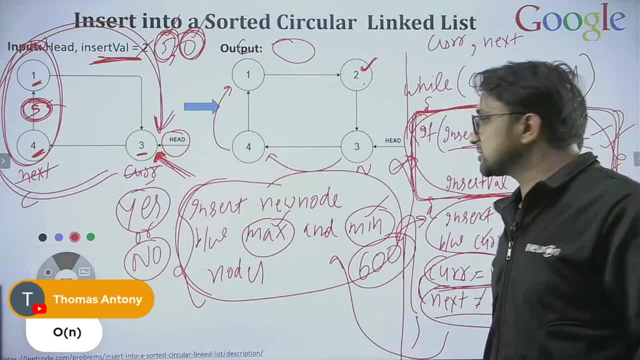 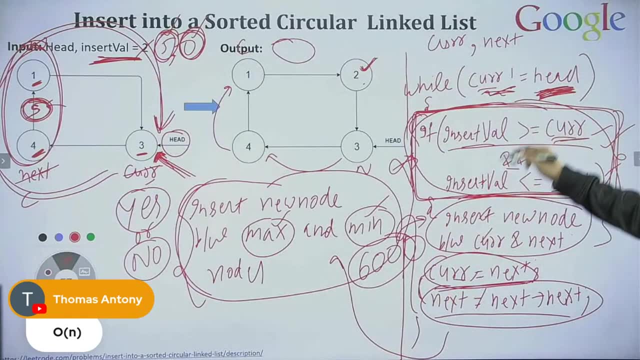 in this loop. loop doesn't matter at all. still the complexity will be: order of n 6000 statement. even i write doesn't matter at all until unless there is some other loop inside the loop. writing single statement doesn't matter, that is still constant. so this loop is coming back to the head starting. 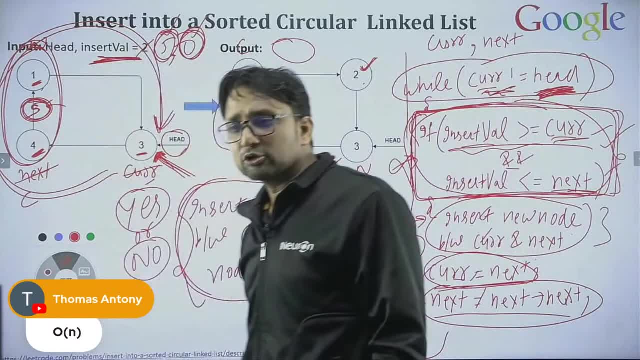 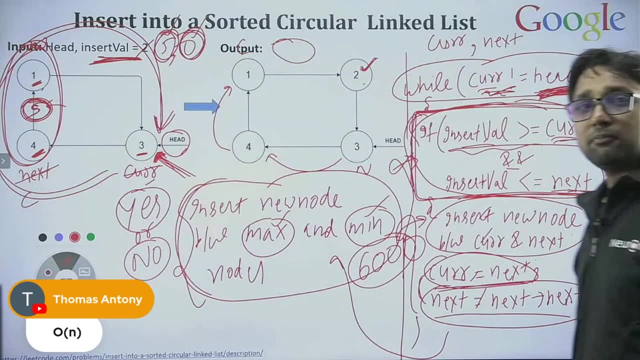 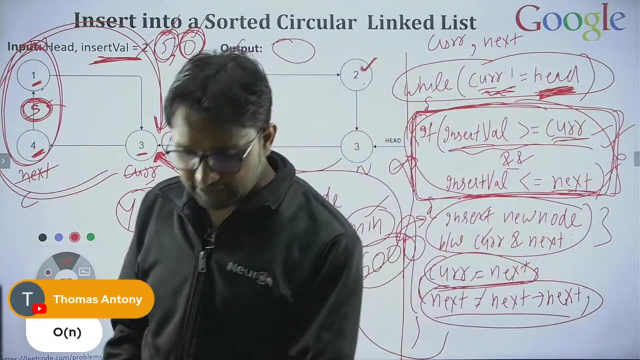 from the head. coming back to the head, number of nodes are n, so this will take n time. yes, this logic will take n time. that's it. any any uh doubt here? you can ask me. any doubt here, you can ask me otherwise. okay, let's try to code it. let's try to code this problem. let me erase this board. 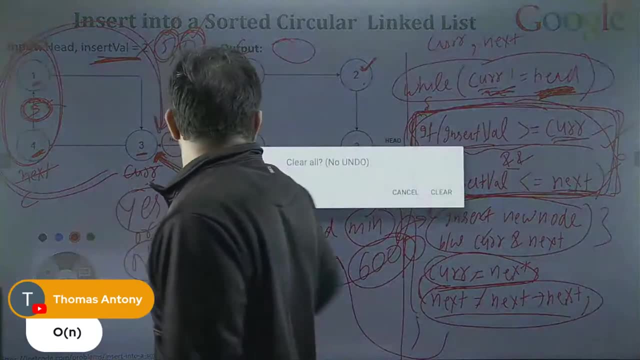 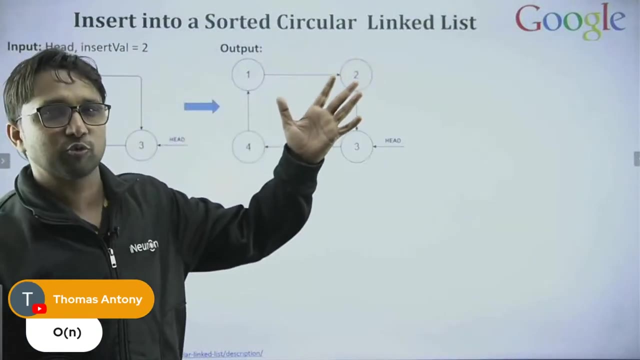 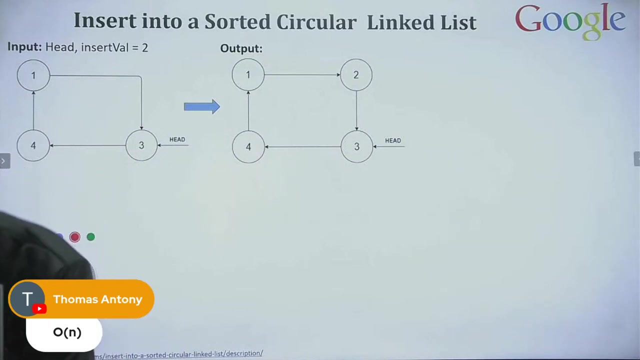 let me erase it. any doubt, please write in the comment section. your doubt will not help only you, but other people also who will watch it later on. they will definitely get benefited from it. from the doubt you have asked, please ask the doubt it's. it's a good idea to do some charity also. 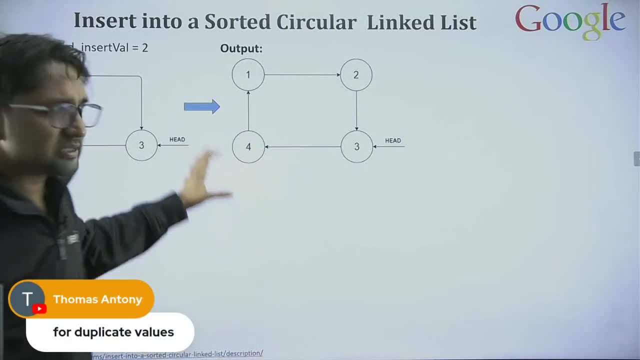 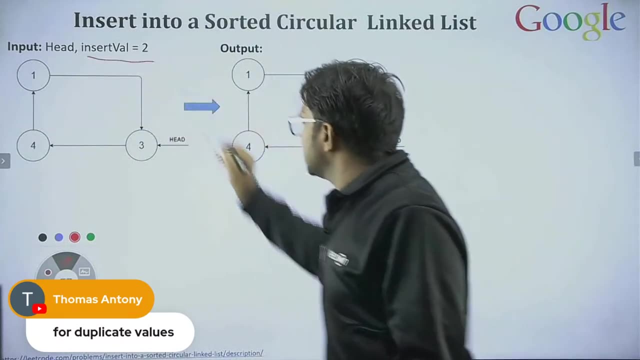 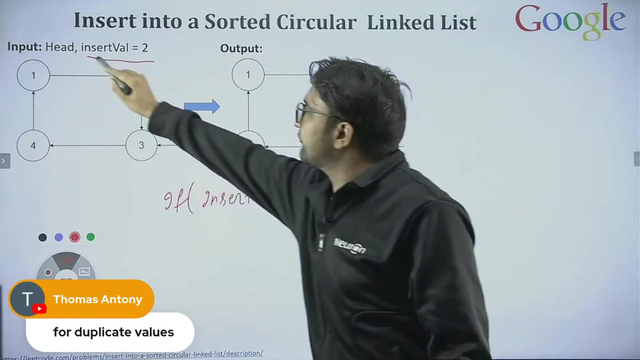 for duplicate value also. thomas, this is working fine. see, you have written great. let me write the condition back so you want to find out. this is the condition: if insert insert- well, see, if insert, well, duplicate value. that is a nice question. is this working for duplicate value? so? 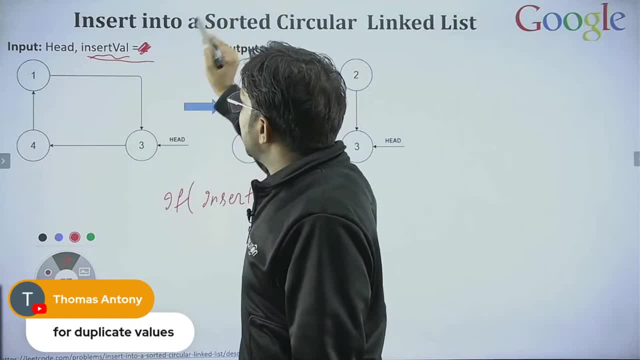 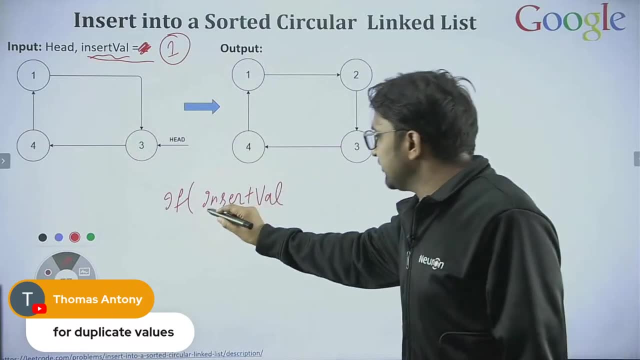 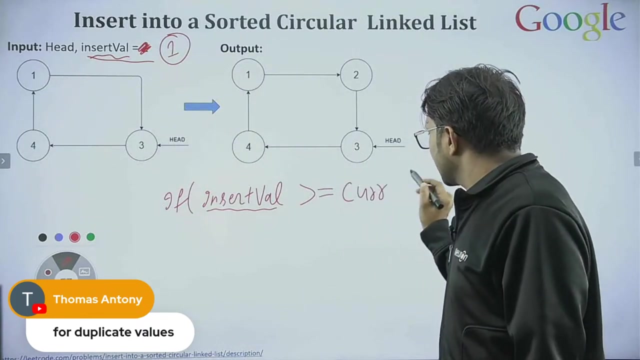 let's suppose i want to insert node 2 here. maybe i want to insert one over here. okay, i want to insert one over here, so let's check. let me write my condition if we insert. the condition was like this: if this value is greater than equal to the current value, the current value and. 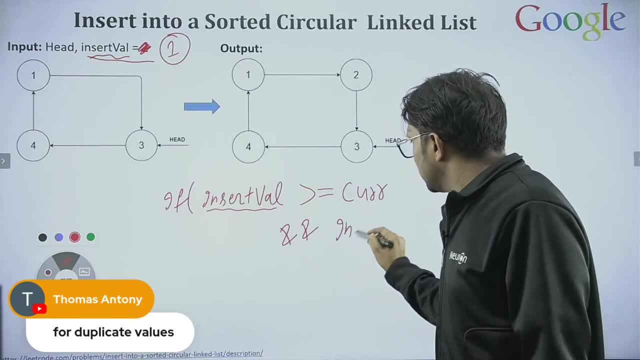 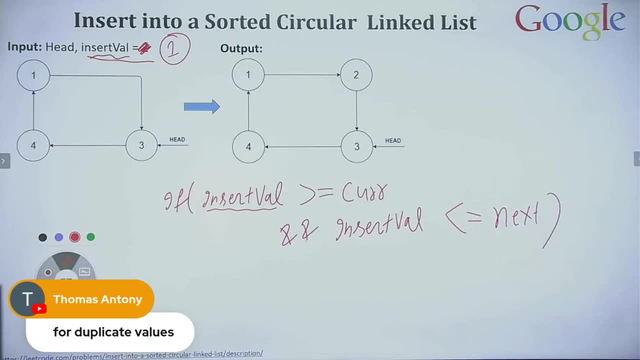 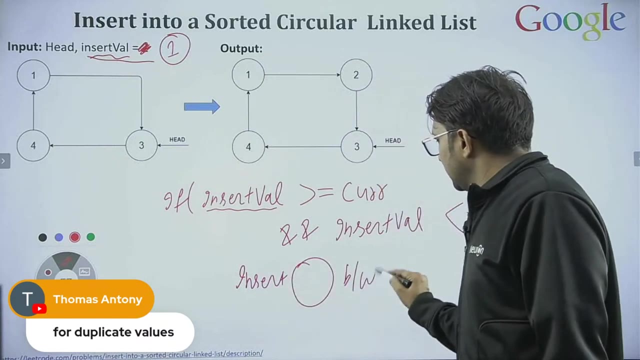 this value insert. well, is less than equal to next value, is that that is less than equal to next value, that is less than equal to next value, and so on. so what we can do here is: let's check, let's look out, then we will insert. then we insert the new node between current and current and next node. that's. 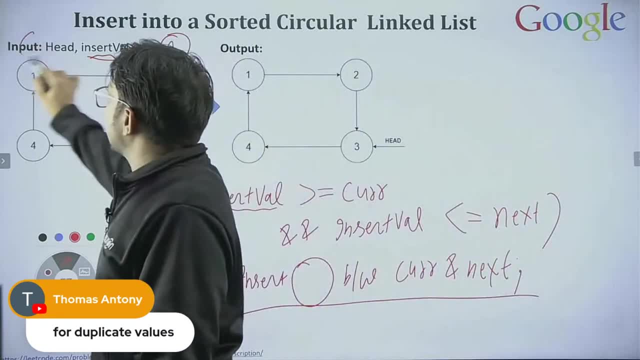 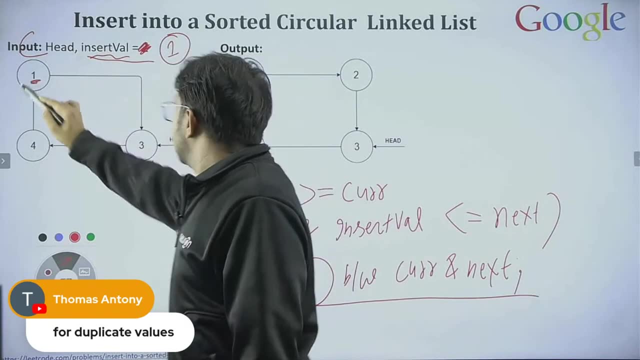 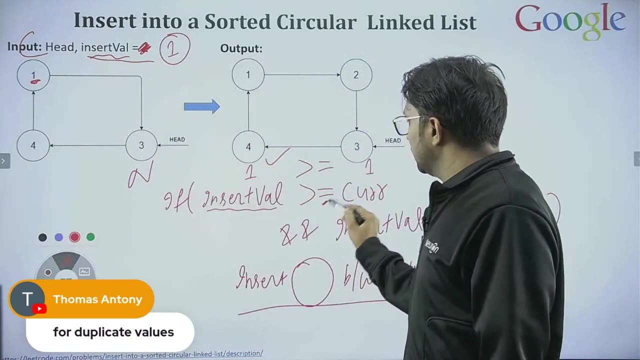 it. that's it. so this is our current node. this is our next node. after moving on, we reach over here, okay, back, and we find out- that is the one let me write. is the this one is less than equal to one? yes, this is equal to fine. and let me check for the next also. next is three. is this less than? 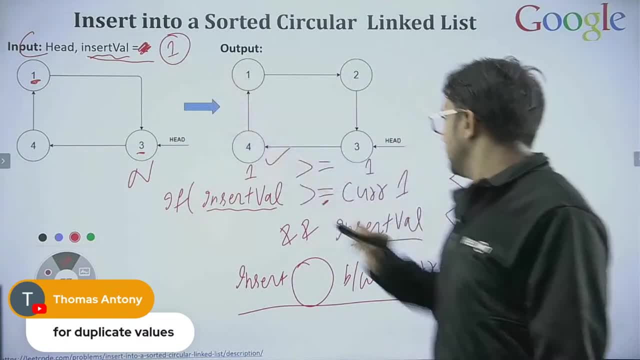 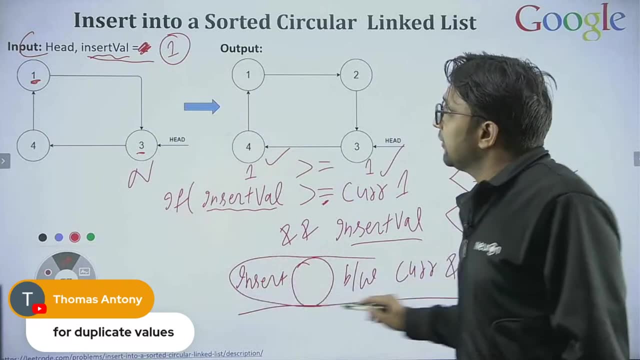 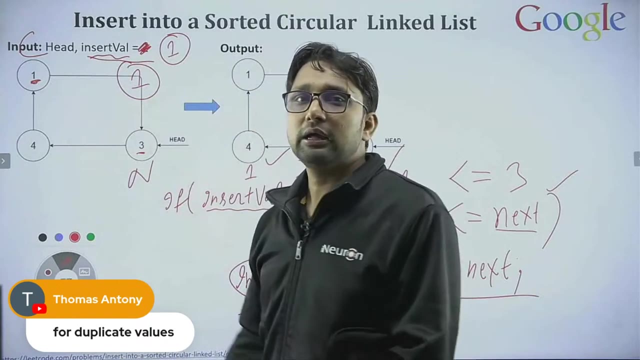 equal to insert values one. insert values one. so is this less than three? yes, both condition are satisfying. both condition are satisfying. yes, we can insert. we can insert one over here and this still fine. it's still fine. this is in non-decreasing order. this is in non-decreasing. 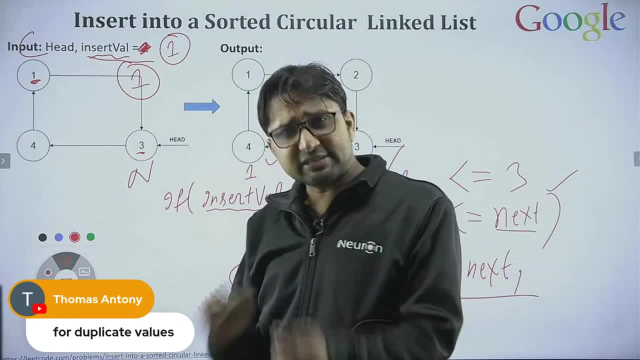 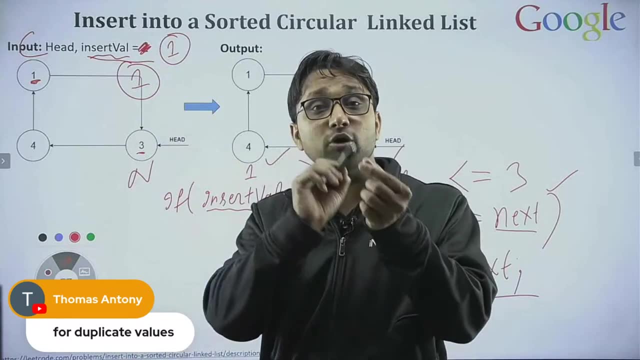 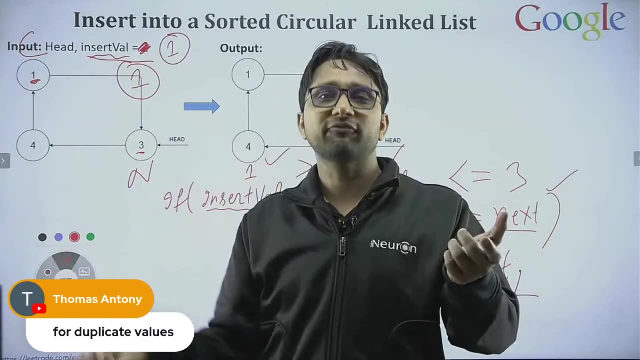 order: one, one, three, three, four. yes, this is in non-decreasing, or you can say increasing with duplicates. what do you mean by non-decreasing? non-decreasing means non-decreasing equal to is what is non-decreasing? non-decreasing means increasing with duplicate values, in which 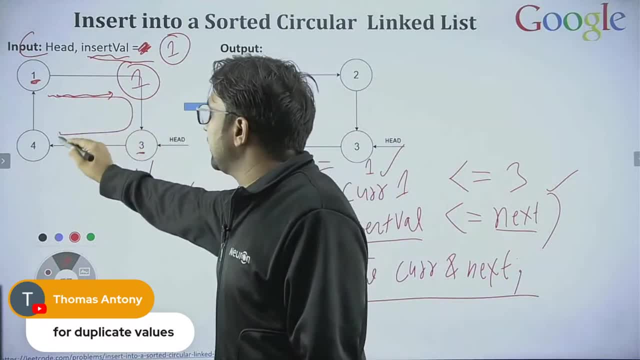 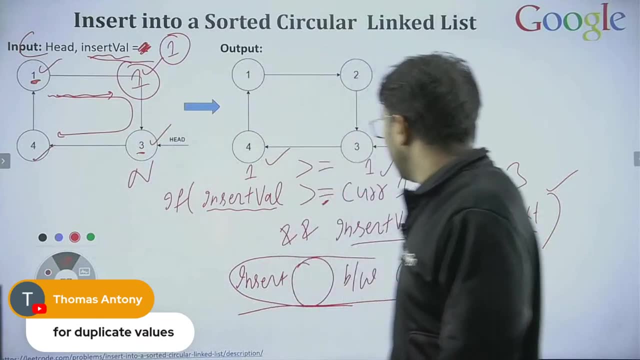 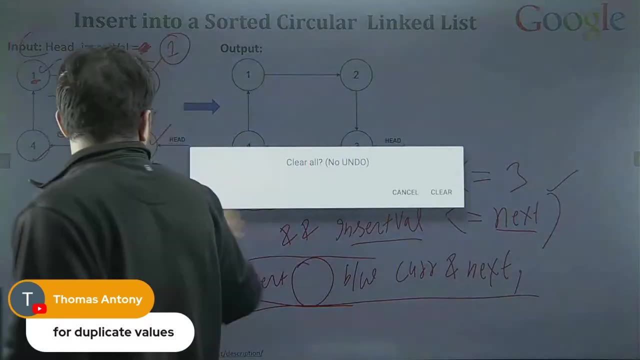 duplicate values are allowed. so this is in increasing order and duplicate values are allowed in this. so, yes, still, our list is sorted. only fine, okay. so yes, this is handling the duplicate values. this is handling the duplicate values. let me do this thing again. the same thing, i will repeat. 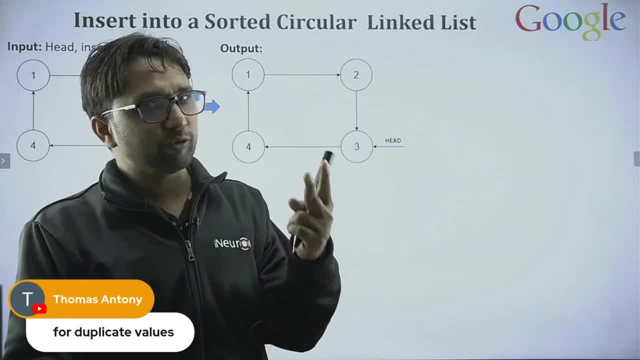 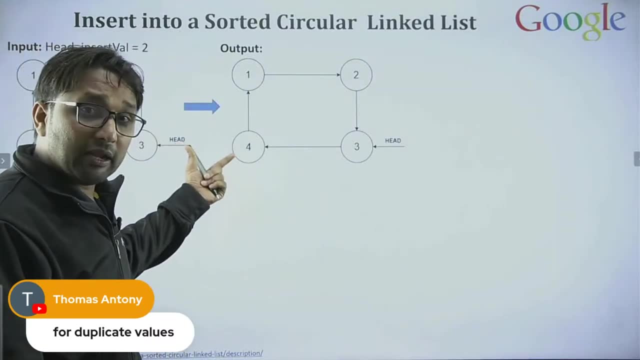 again. if you are not able to understand anything, two things we can do. either you please ask the question in the comment section. second thing, i will explain each and everything again, i will code it and i will do the same thing so you can understand. we have one more chance to understand. 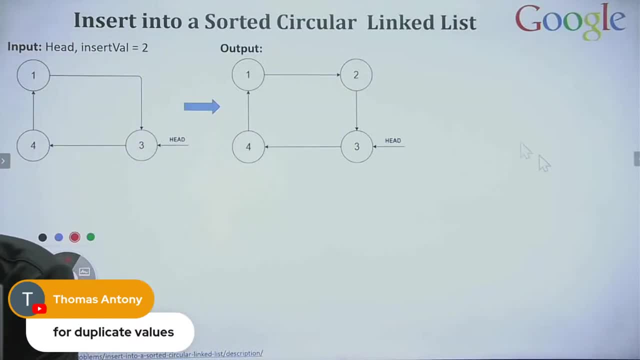 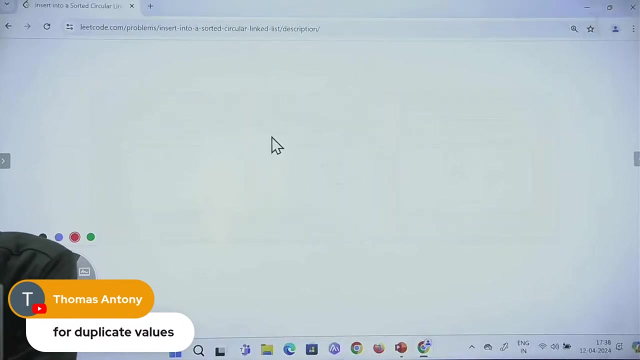 this problem and you people please keep helping me while doing the code. let me share the code with you. hi, bishal, nice to see nice, nice to see you back here. so please help me, bishal, here, to code this problem. please help me over here. i just picked. 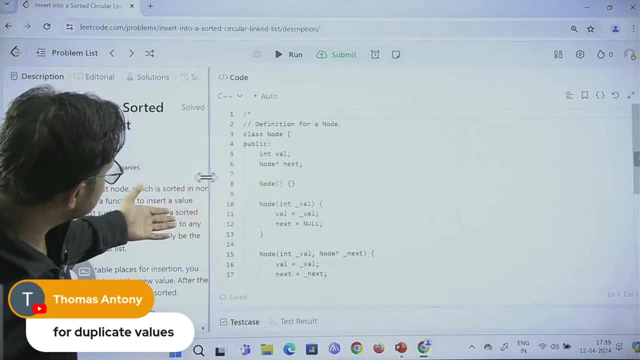 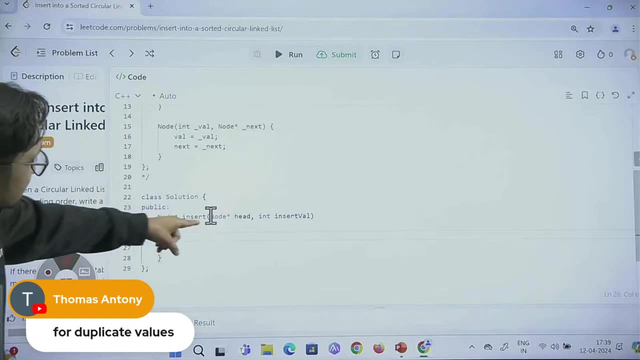 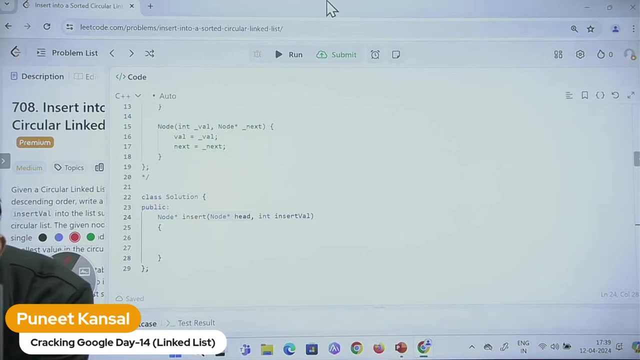 this problem from the lead code. so let me stretch this thing over here and we need to code over here what they provide us. they provide us. let me increase the font also. maybe that will help you people. let me increase the font. yeah, we are going to solution only directly. don't need to worry. 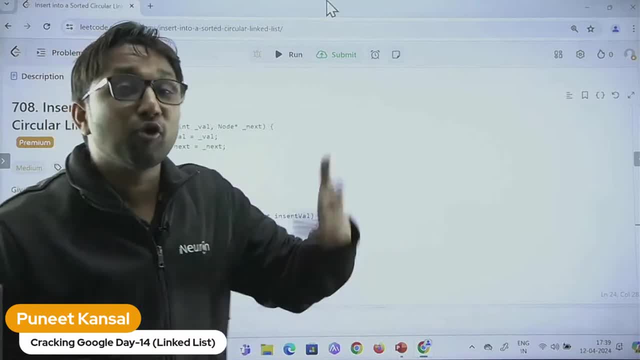 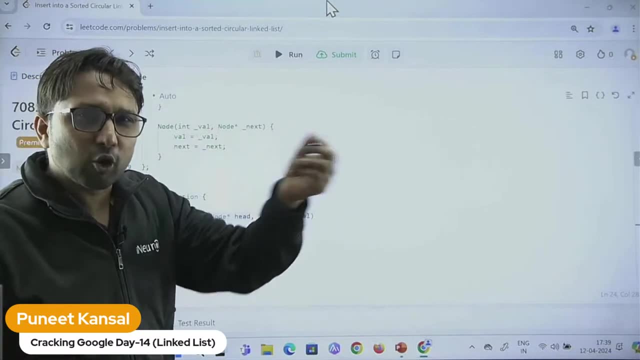 we are starting. it's like. it's like we are starting from zero itself now, right now. don't need to worry if you know the problem. what is the problem? simply, you need to insert a node in a circular linked list and the circular link list is sorted. 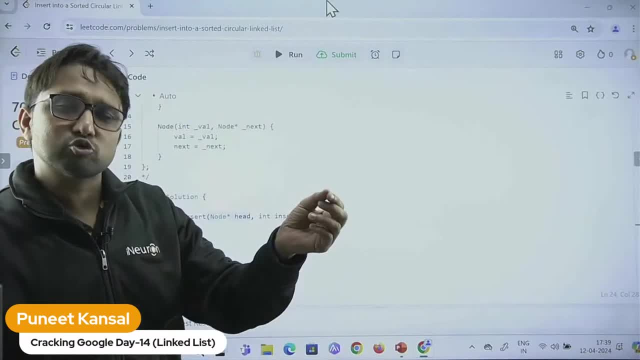 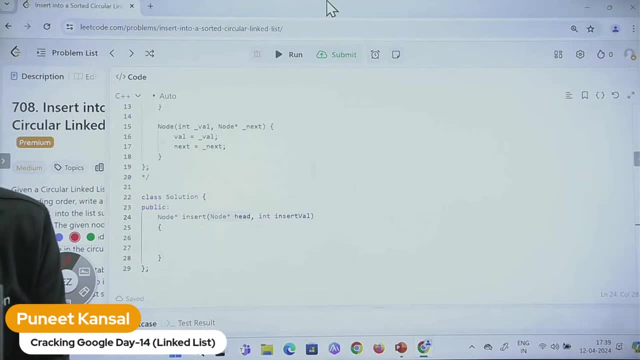 after insertion of new node, the circular link list should be sorted. so this is the. this is the problem and we are going to cod it. i'm increasing the font so that even you are watching in mobile you become able to watch it. watch it little better way, so i hope the font is better now. 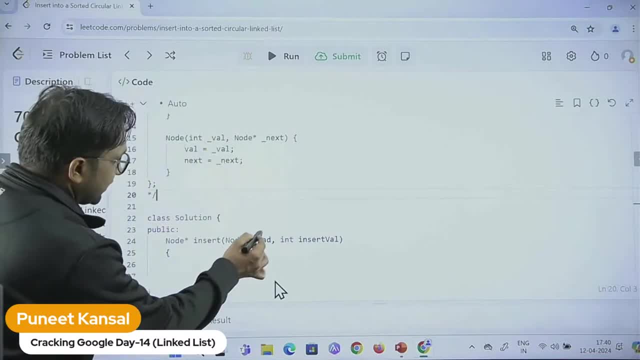 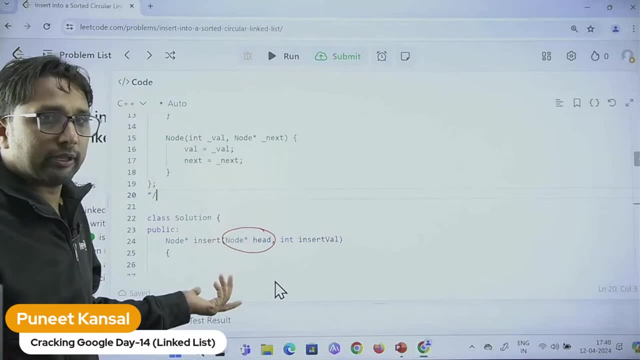 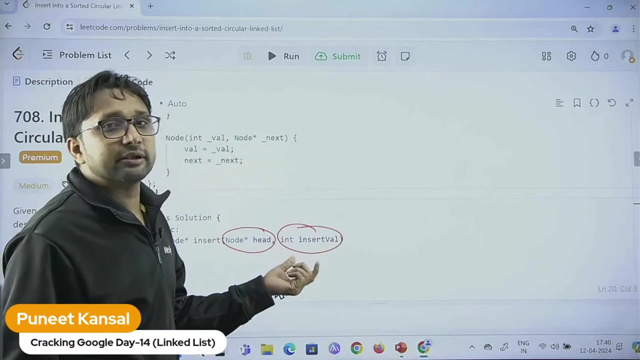 and what they provide to us. here you can see that they provide us the the head node whenever somebody share the link list. actually, they share the head only and they provide the value which we need to insert as a node. Okay, we will insert this. 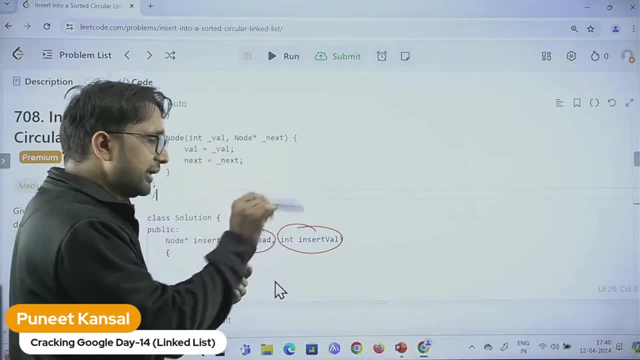 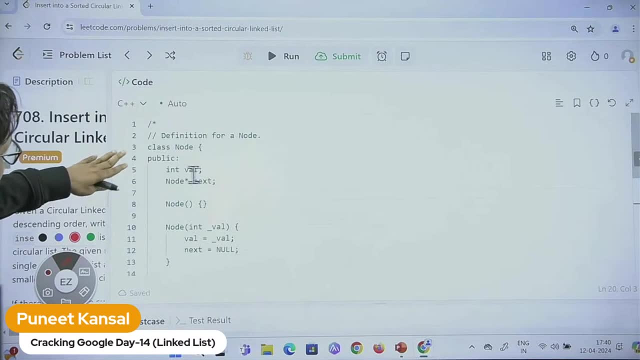 value in a node and we will insert that node in our link list. That's it. So these are the two things are provided. And if we see in the, in this driver code also there is a class node And we can insert, this means it is a structure of a node is a structure. 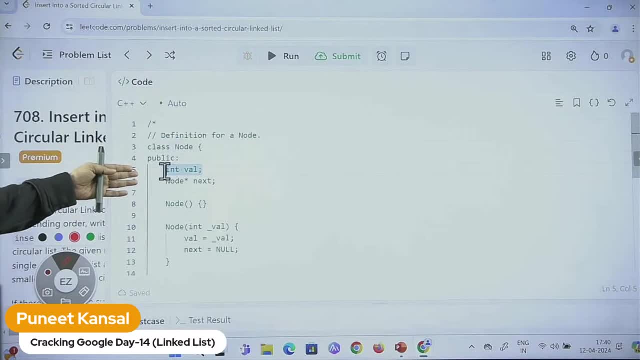 of a node. we can insert a value in the node And there is an address also. there is an address part also in the node where we can insert the address of the next node, address of next node. So I will code, I will provide the code for all the languages: C++, Java and Python. 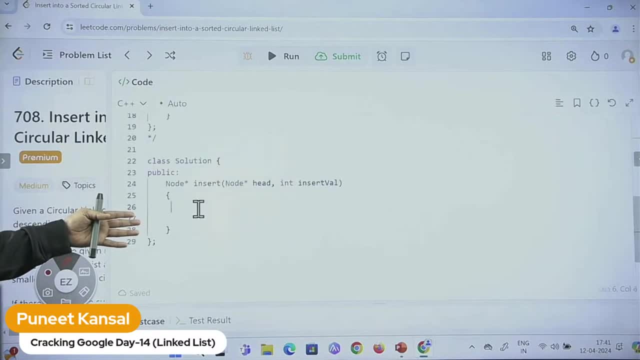 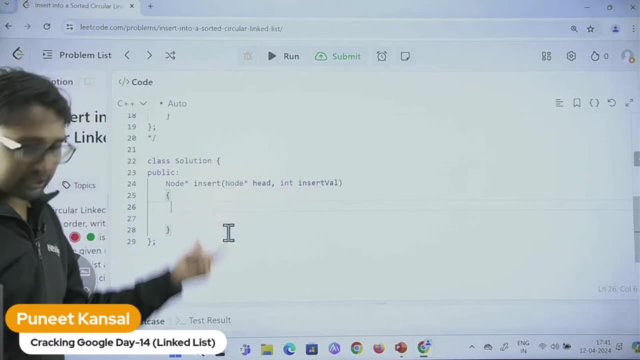 but let me first code it into C++. Fine, So simply, they provide us the head node and you just need to check out the logic, that which is important. So, first of all, let's create a, let's create a new node, Let's create: 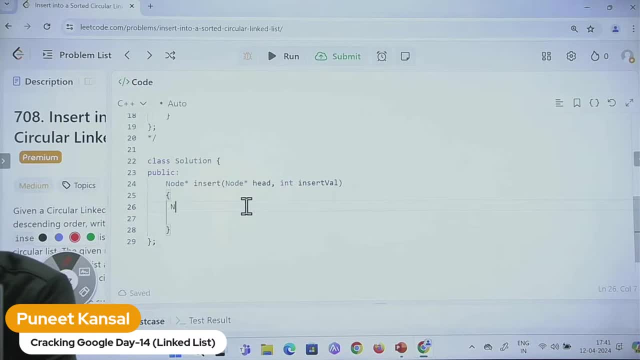 a new node, node. I'm creating a new node, New node. Let me create a new node, So don't need to worry if we are not simple as plus programmer number. You do not have to worry because this is your process with C++ in monod. 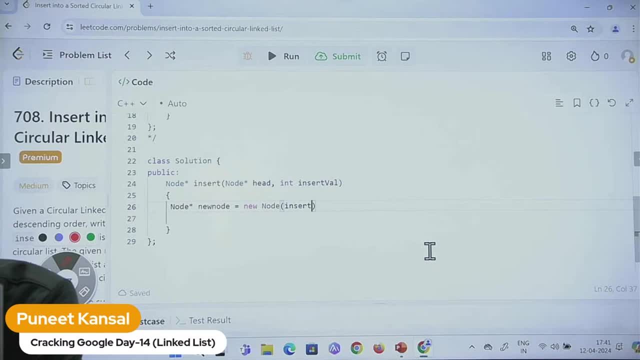 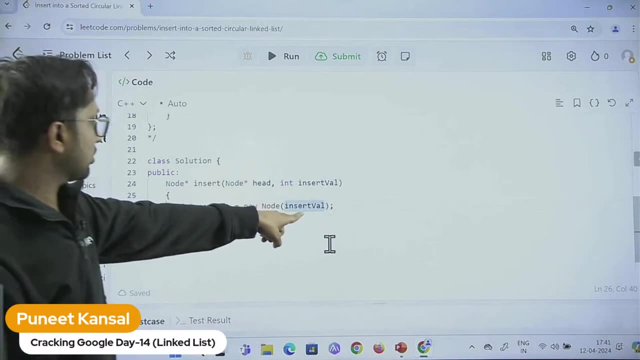 don't need to worry at all. Just we are creating a new node. What I'm doing just creating a new node and inserting this new, inserting the value in that node. created a new node and inserted this value which was provided to us. So this value I inserted in this new. 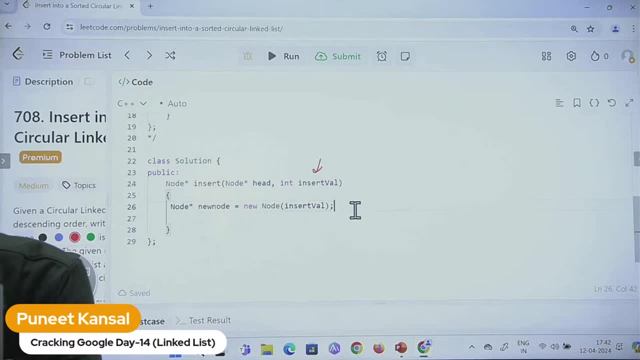 node. That's it. And now we need to find out the place where to insert this new node. That's it. Let's find out this place where we need to insert this new node. First thing I can write is first thing I can write is first thing I can write is if the head is null. 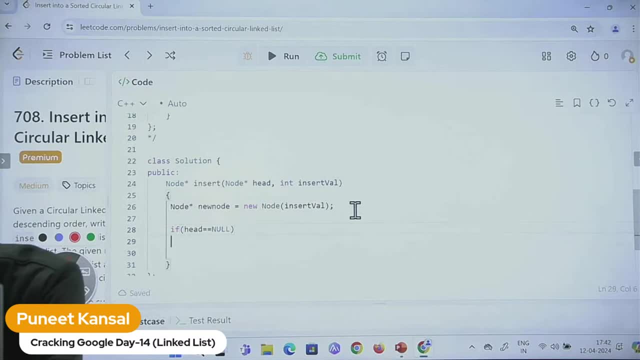 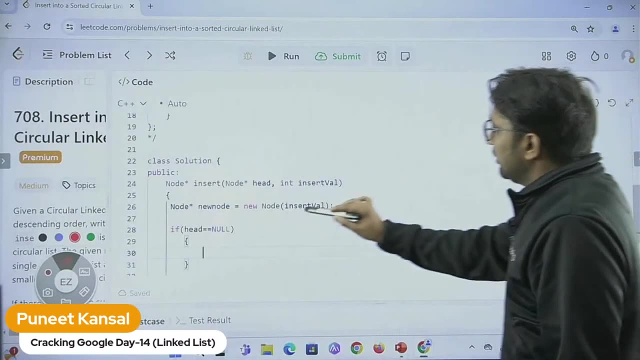 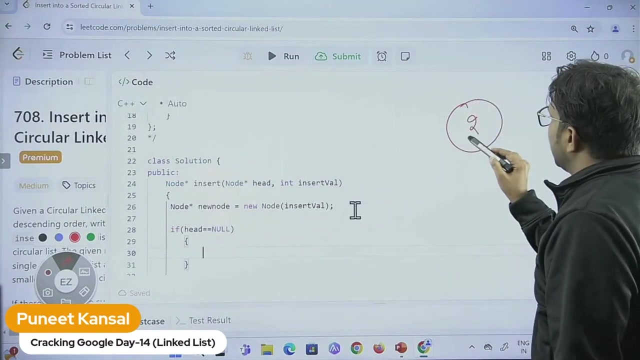 if our linked list is empty. if our linked list is empty, then what will what? what will happen? nothing. if linked list is empty, then we have already created a node with this value, insert value. let's suppose insert value is two, Then what we will do? actually, every node, every node is like this, only we have a value part. 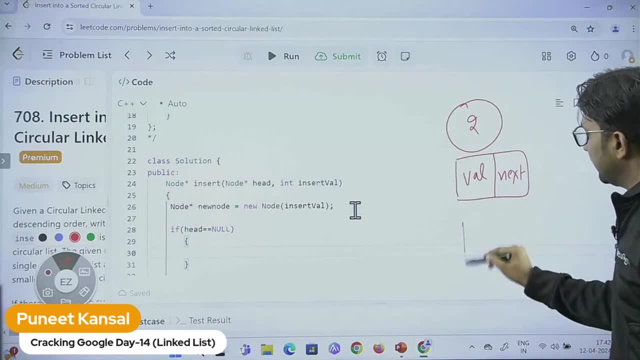 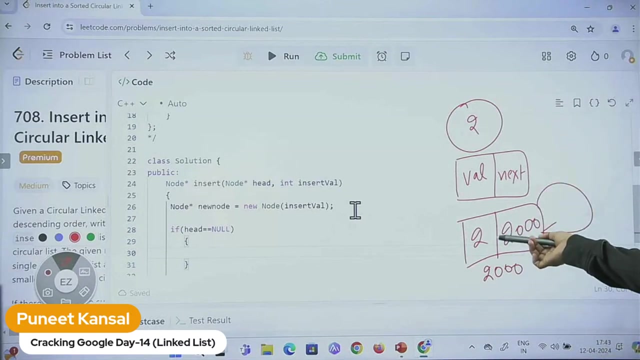 we have our next part, And here the value is two. In the next I will put the address. For example, the address of this node is 2000. I will put 2000 over here so that this become a circular linked list, single node, circular linked list. And this is our head also Head. 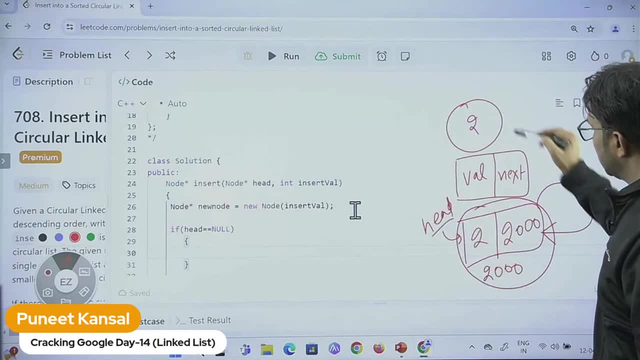 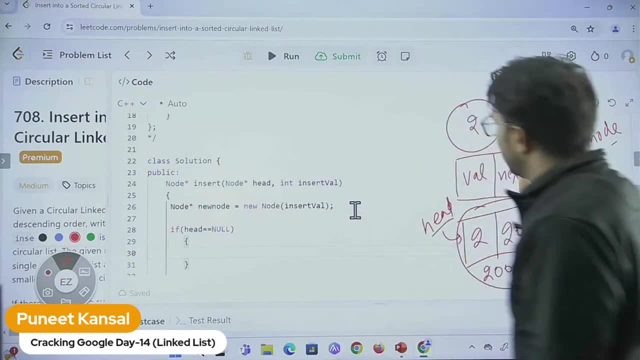 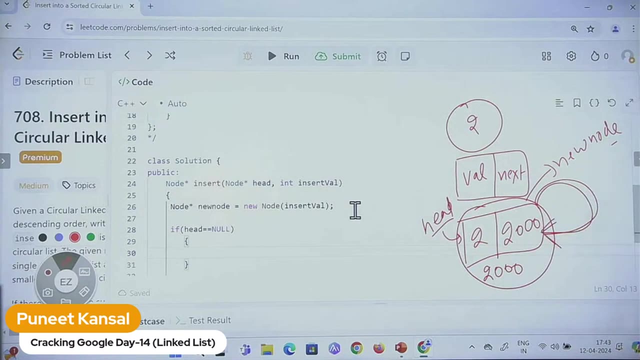 is now 0.2.. This is our new node. This is our new node. This is our new node. So I'm just checking that if the head is null, then this new node should start pointing to itself. should start pointing to itself and we can return this itself, this node itself. So let me write the. 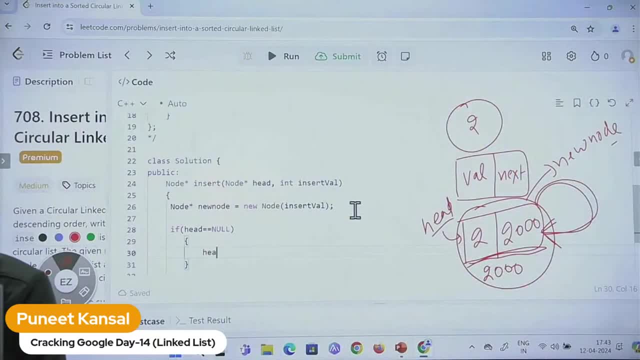 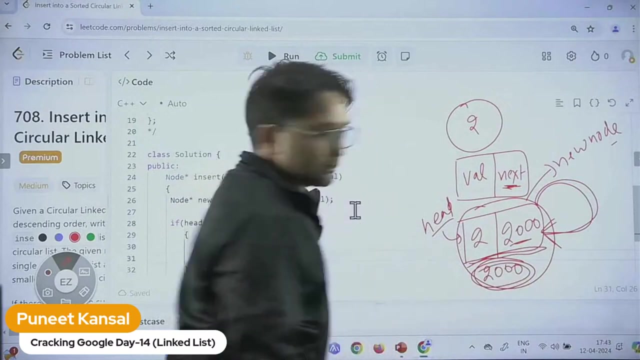 code for that. What I need to do, our head is should become our head, should become this new node. So this node will become our head. And in the new new node, next part in the new node, next part, in the next part of new node, here I will store this address itself. So let me 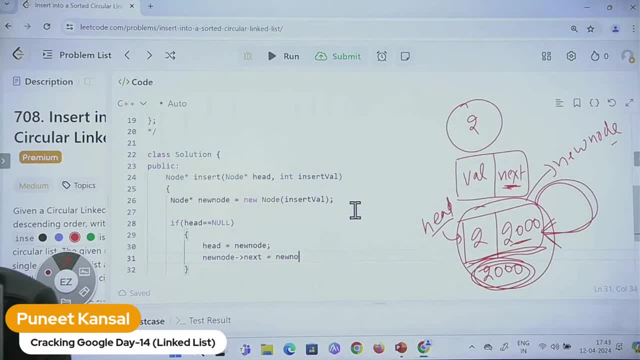 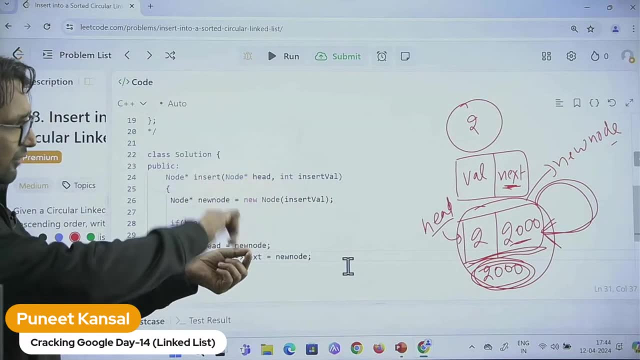 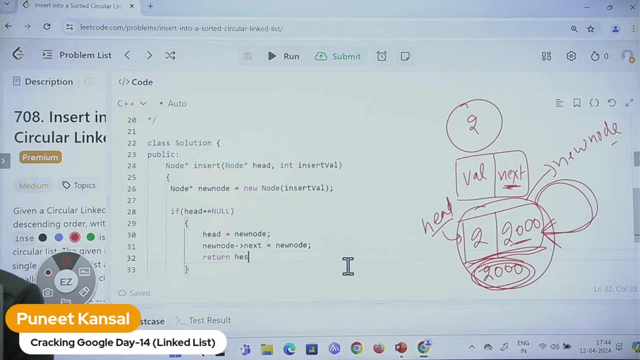 store this address itself over over here. new node, new node itself, new node address, and storing itself in the next of that because single node is there. we need to make it circular, So we make it, that's it, And after doing this, you can return it on the head that said so. this is how we are. 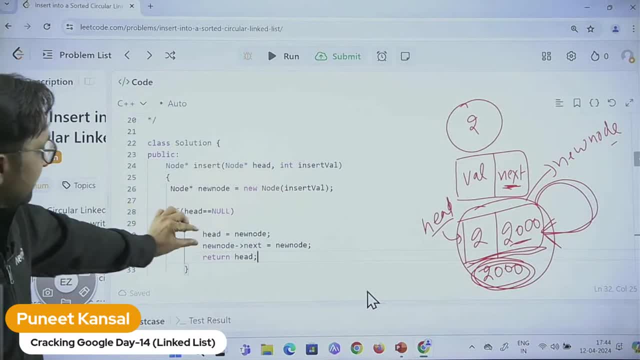 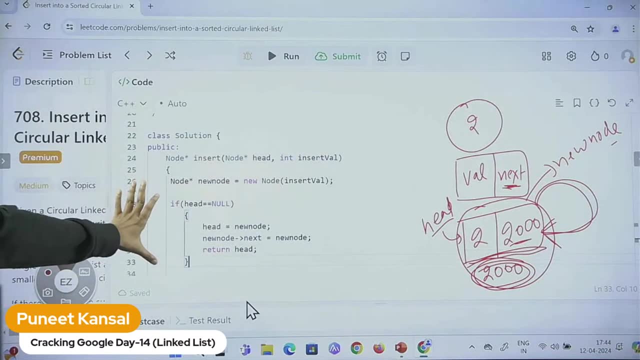 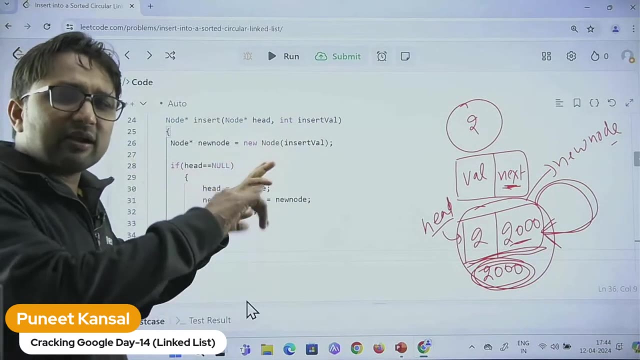 handling the amputee linked list, simply created a new node, make it circular and return it. that's it done. done with the amputee linked list. After that, what we were doing, we were taking a two pointer- one is current, one is next. and going through a loop. We were taking a two pointer- one is current, one is next- and going through a loop. we are not doing this again And after that we should create a new node. a new node, make it circular and return it, And this is what we're used to doing. So this is how we are handling the empty linked list. 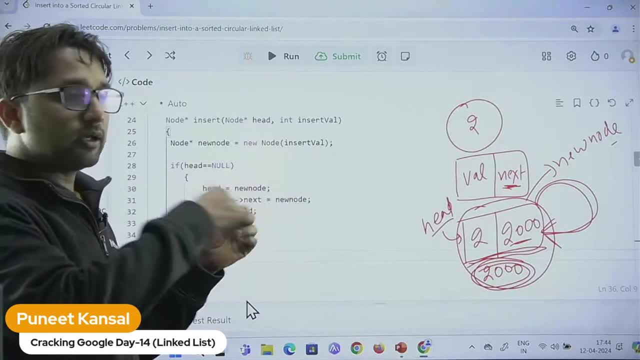 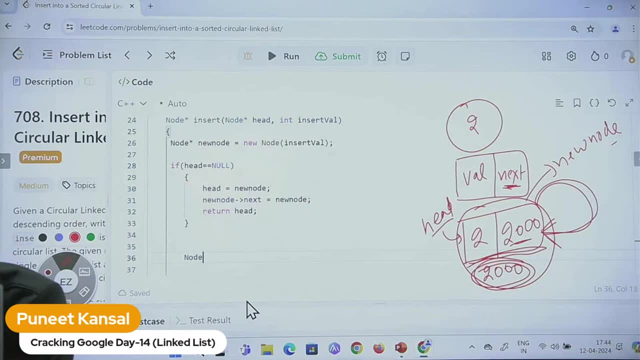 through a loop and checking a condition which we write. so let's write that code itself. so let me write that code. so let me take a two, two pointer over here. one is current and okay, let me point the current to head, and another one is next. so for against to these two, i will check out. 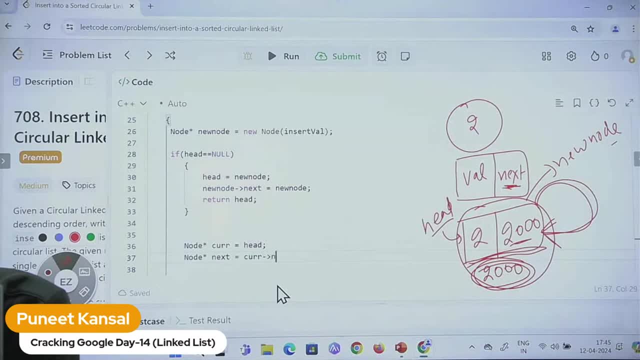 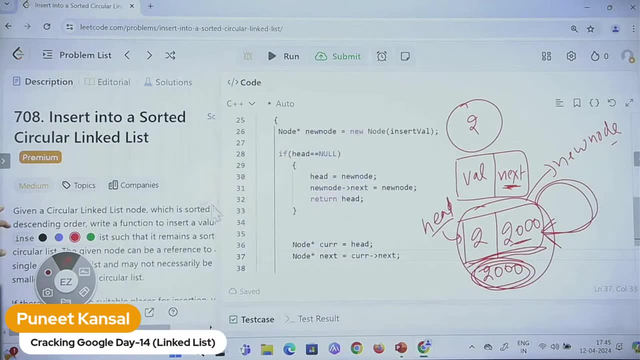 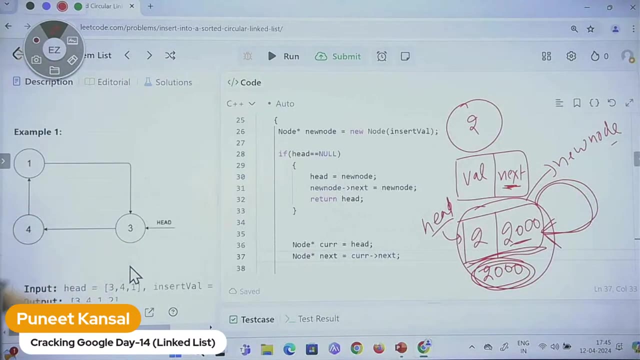 the condition. so current, next, fine, okay. uh, current is pointing to the. let me show you over here. let me show you over here in the here, over here, okay. so now current is pointing here and next we'll point out here. then we will keep doing this thing inside the loop. 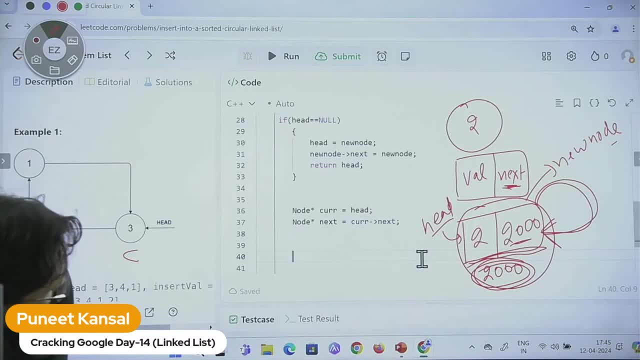 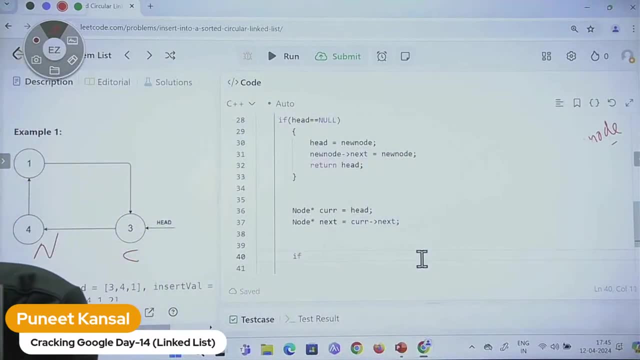 let me write the condition first of all, which we discuss, which we discuss that we erase this part. the condition was: if new node, if new node is, is greater than equal to current node, okay, new node is greater than the current value and new node, new node is less than equal to next value, next value. 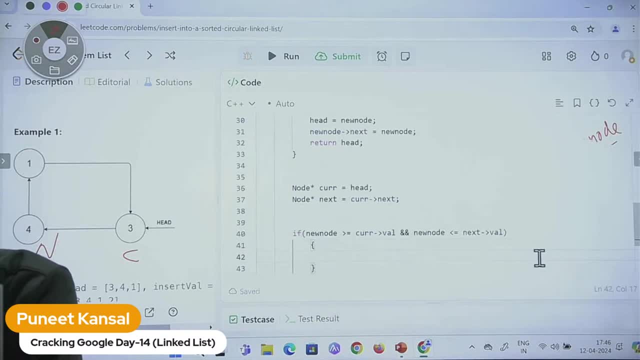 this condition, then what we, what we will do, we will insert the node, we will insert our new node. so let's insert the new node that will be inserted between current and next node. so let me try to insert the node. so for that, okay, current next in current next, i will store the new node, fine, and in new, new node next. new node next. 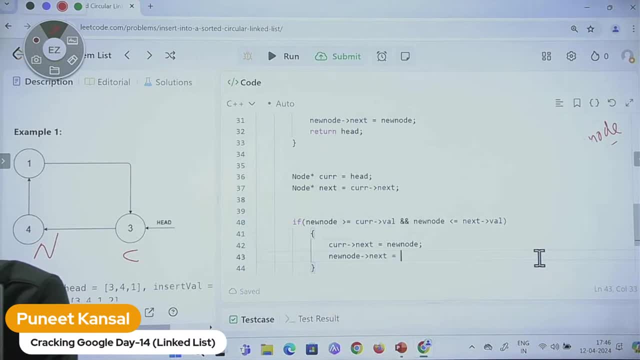 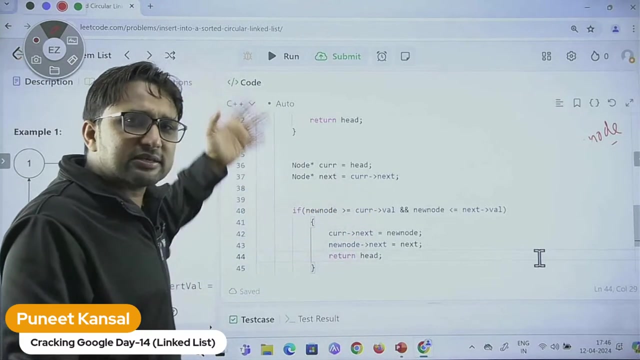 i will insert the next node. i will insert the next node, that's it, and we can return from here. just return, we inserted the node, we inserted the node, we inserted the new node. then just return. the head done, our task is done. but if this is, this condition is not satisfied here, then we will make. 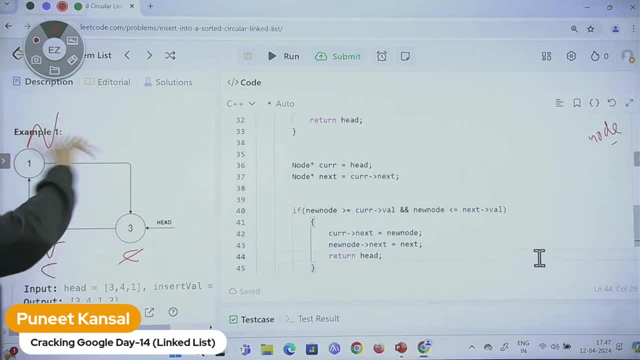 this as a current and this as a next node. we will keep doing this until until- unless current is, we come back to the head node. okay, until current is not equal to head. so we will do this thing again and again. so let me put this inside a loop. 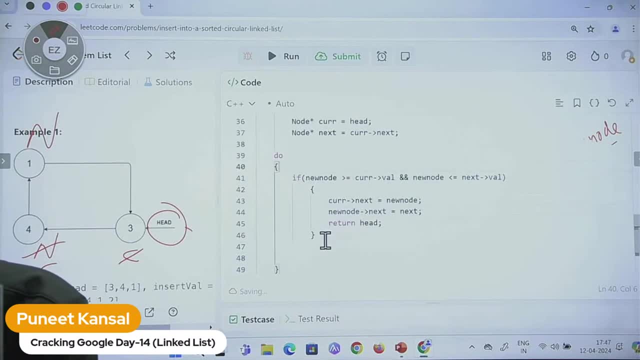 you people, please think over and reply. at the end i will ask you why i am using the do while loop, why i am using the do while loop here, why not? i am using the while loop directly. so this question you need to answer later on. so until current is not, 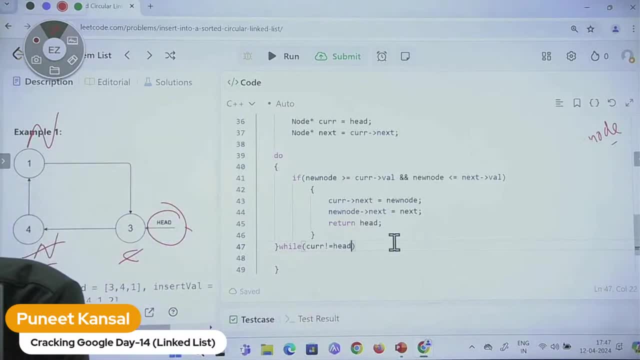 equal to head. fine, so we will keep executing this loop. i put it this condition, inside the loop which we discussed already, let me increment the current value. so in the loop, definitely, we need to increment the current value. so current is equal to next. now, and what will be the next? okay, next. 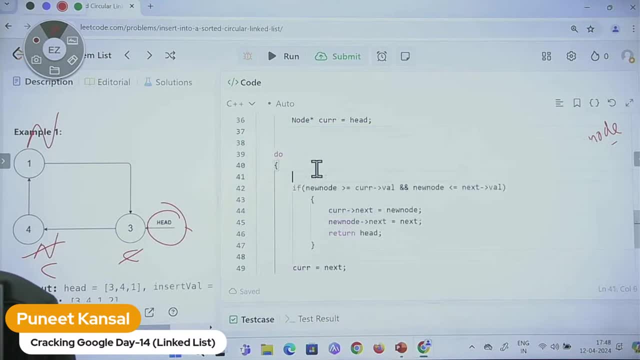 already we have this statement. let me put this inside the loop itself. so because every time we need to update the next also and every time we need to update the current also, so like current will be this, next will be this, then current will be this, next will be this, then again current will be this, next will be this, like: 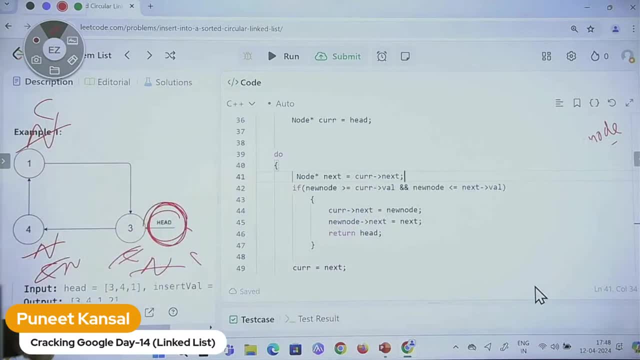 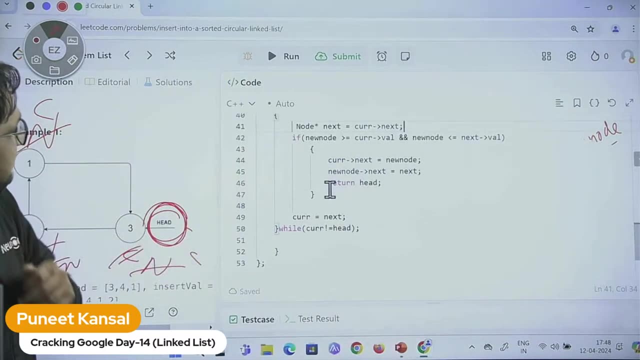 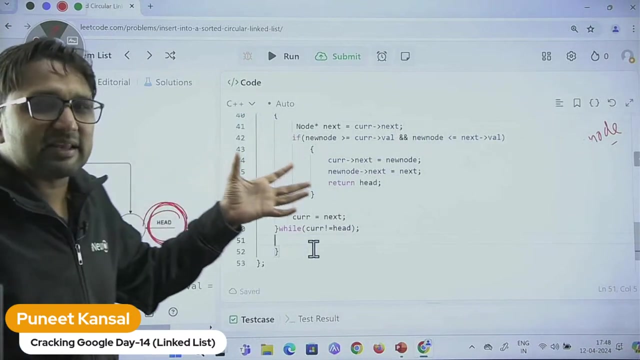 until, unless our current will reach to the head, we will keep doing this thing. until our current will reach to the head, we will keep doing this thing. fine, okay, so this thing is done, and after coming out of the loop, after coming out of the loop, one last condition is left. 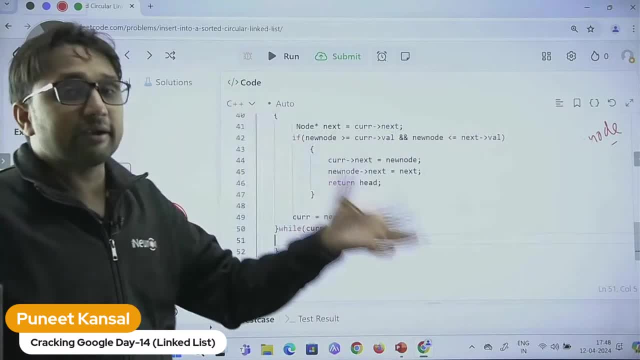 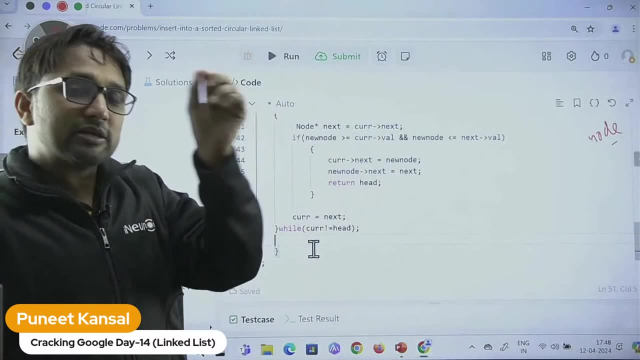 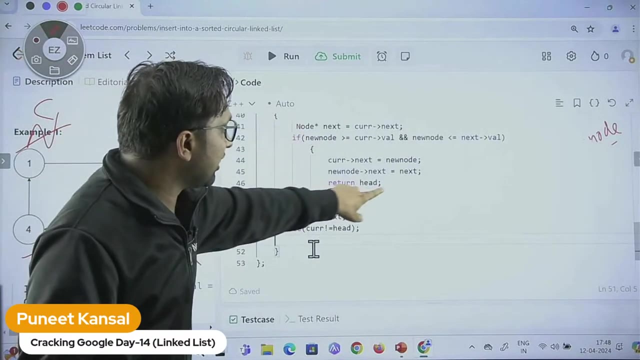 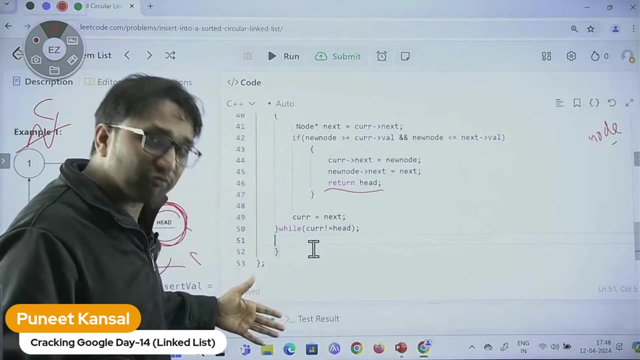 if the value is not get inserted, that means the value will be inserted into the maximum, maximum and minimum element. there is the only place the value will be inserted, even if the value is not inserted in between this loop. if we do not return, we, we do not insert the value and return from the loop then and we are coming out of the loop. 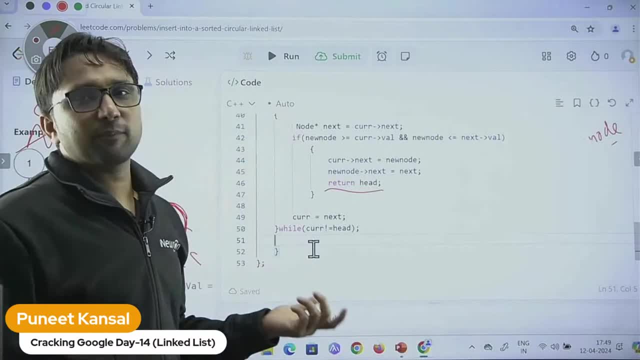 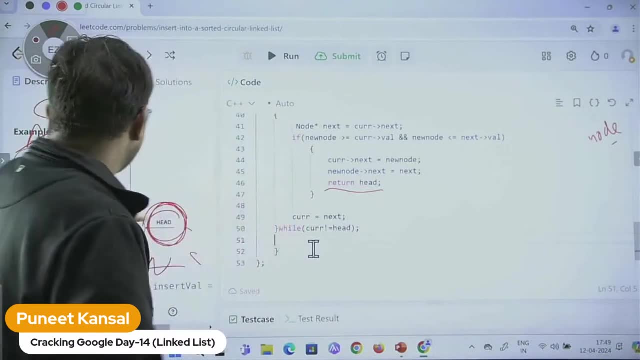 still, our code is executing. so there is only one place left where the node is not inserted and we are coming out of the loop. so there is only one place left where the node is not inserted and that is between max and min value. but we do not know the place. we do not know where is this max and where. 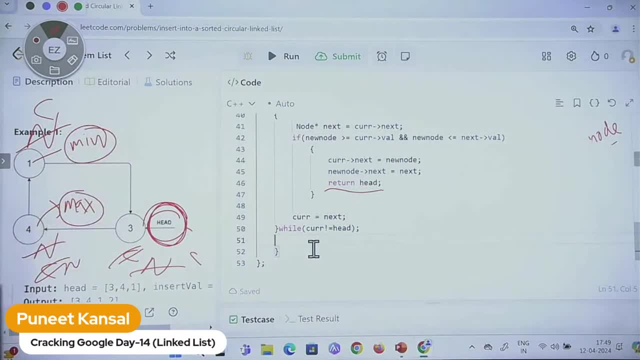 is this min? so to find out this max and min, okay, we, i can insert a code inside the loop itself wherever one value will be greater than the, wherever the current value will be greater than the next value. so i will find out this location, so i will what i am doing. 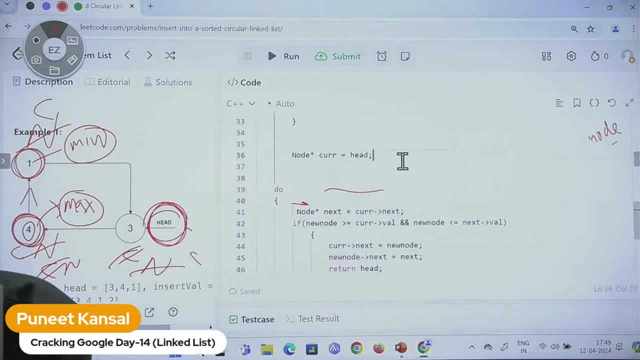 okay, over here let me take two more variable. nod: one is a max- okay, let's suppose max is pointing to head initially, and one is a min- okay, which is pointing to the next element. fine, okay, what i am doing over here is listen carefully. last last thing: i am just trying to find out the location. 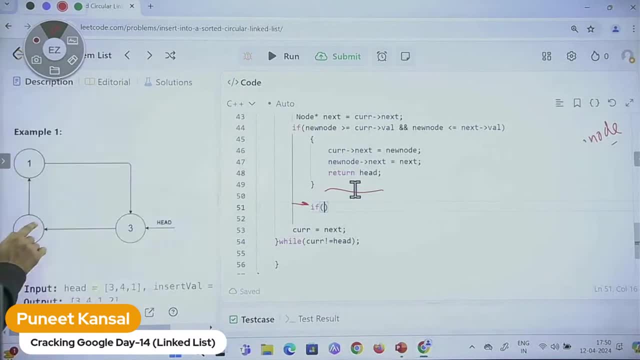 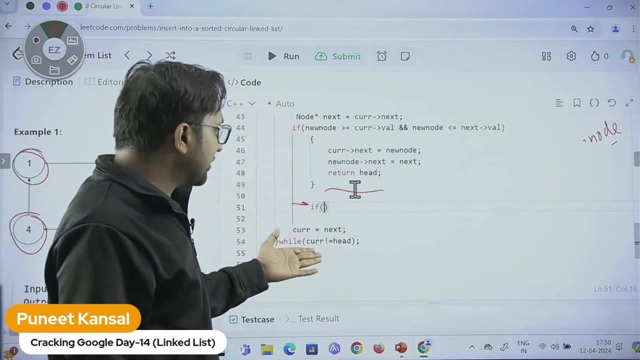 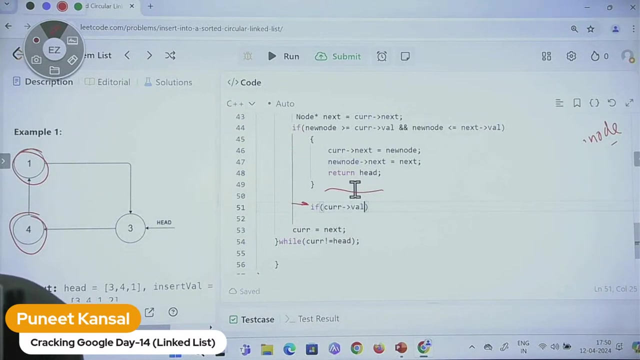 of the maximum element and minimum element. i don't know. i don't know where is the maximum, where is the minimum. so i am taking the benefit of this loop itself and i'm checking if the current, if the current, if the current value is greater than the next value, IPись. 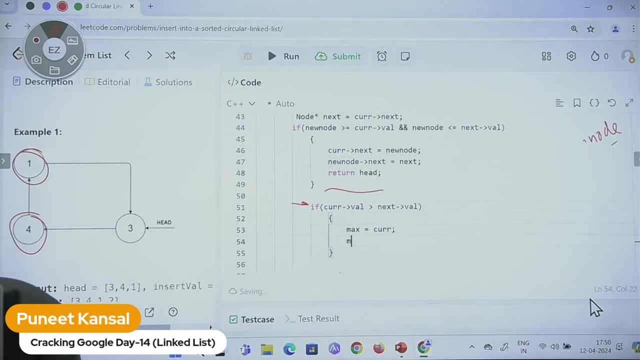 be current and min will be next. do you understand this thing? how many people understand this thing? please reply in the comment section. please reply in the comment section if you understand this statement. pranams: hello, hello. i wish nice from where you belong. i wish from where you belong. 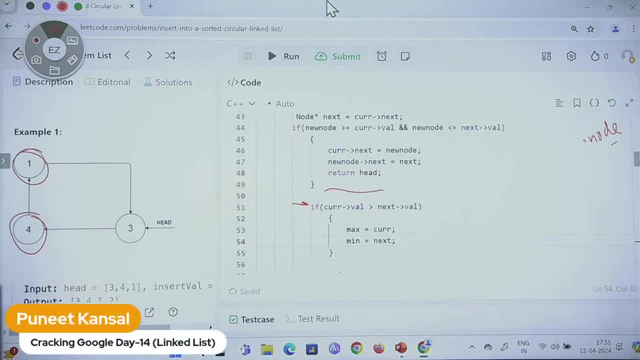 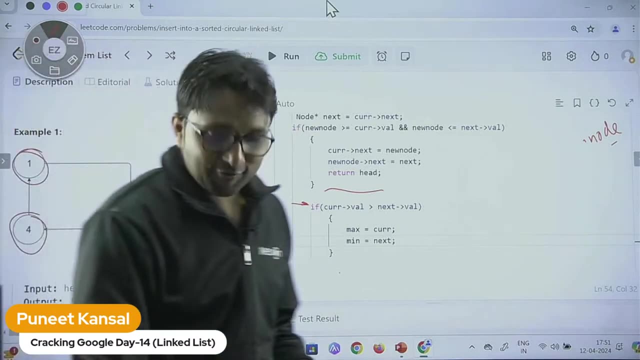 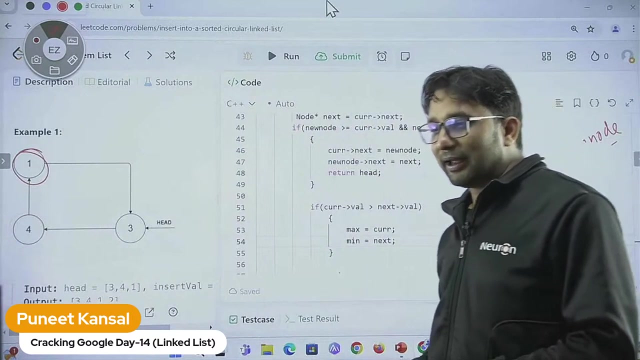 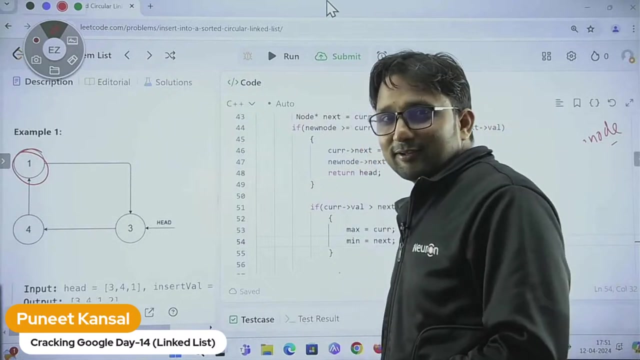 okay, fine, nice to see you back. can you tell me, ayush, this is the question from you only then. okay, you, maybe you are not from the starting of the lecture, so still, okay, if anybody can reply. you are from bihar, fine, so in bihar we don't we say pranam, that is a, is that word we use over there? 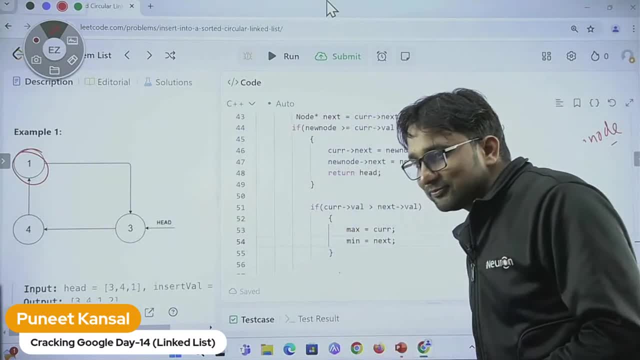 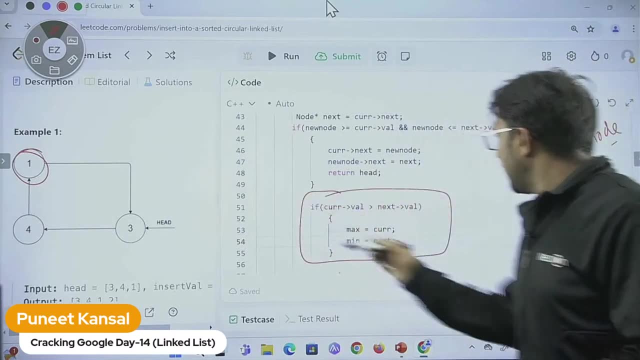 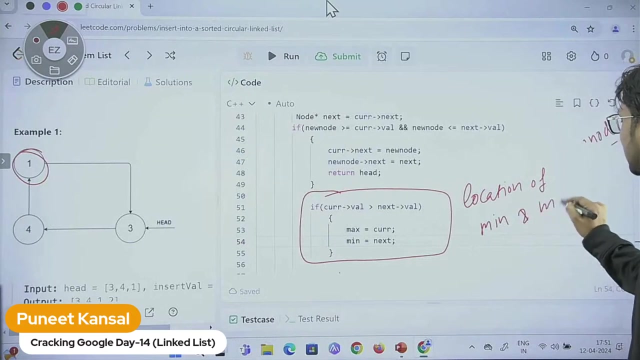 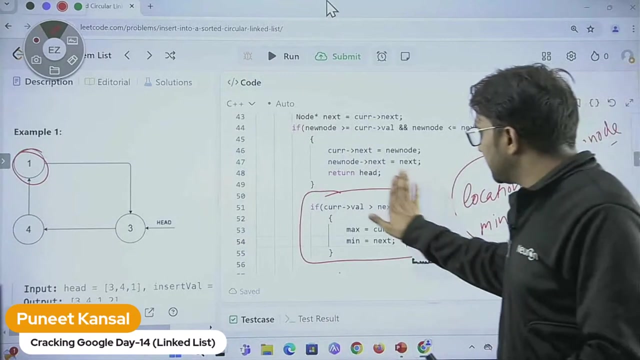 fine, okay here. the question is that what i'm doing over here i'm finding the location of minimum and max nodes. why i'm finding the location of minimum and next node? max node? because after coming out of the loop, after coming out of the loop, after coming out of the loop, 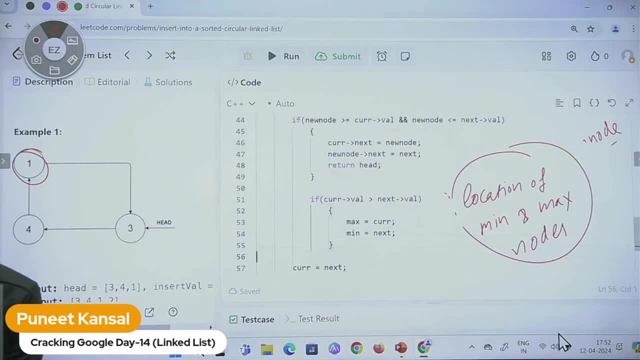 the loop. let me come out of the loop. after coming out of the loop, you can suggest me, you people can suggest me what which is the right time for the lectures. also, if you, if you think that, okay, this is your college time, then might be, we can schedule the lectures. 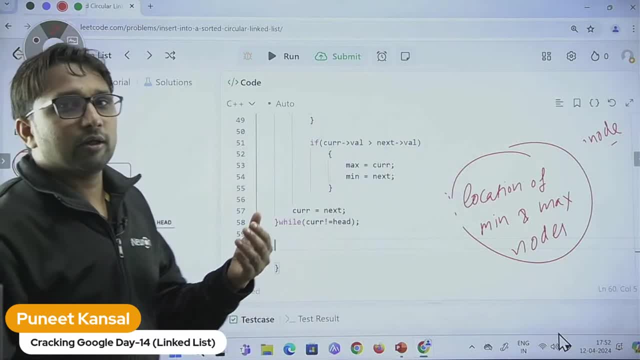 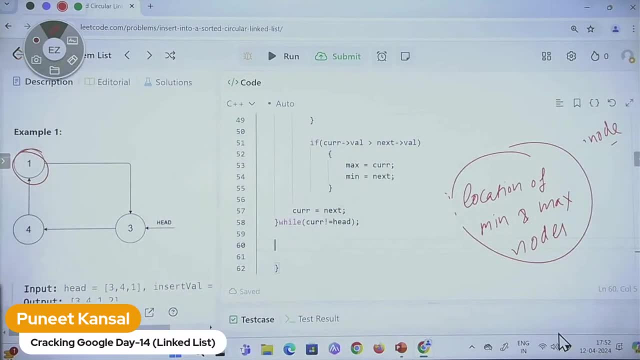 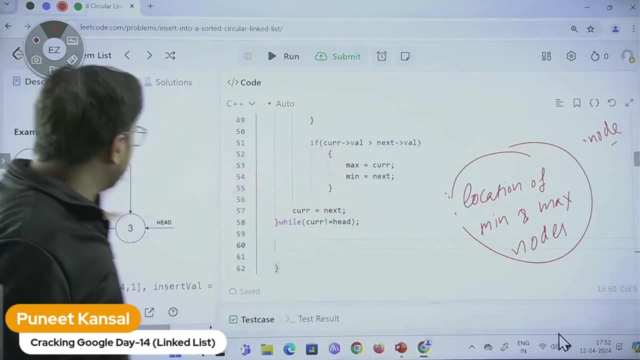 after the college also. so if you think that, okay, uh, the best time can be other other time, so you can suggest me that also. so i will try to schedule the lectures according to your convenience. so, after finding the position of maximum and minimum node, after coming out of the loop, let me insert: 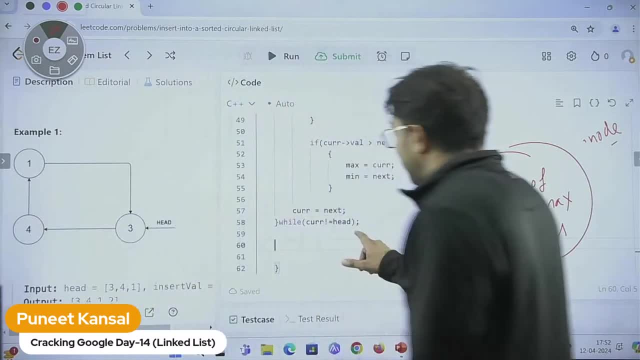 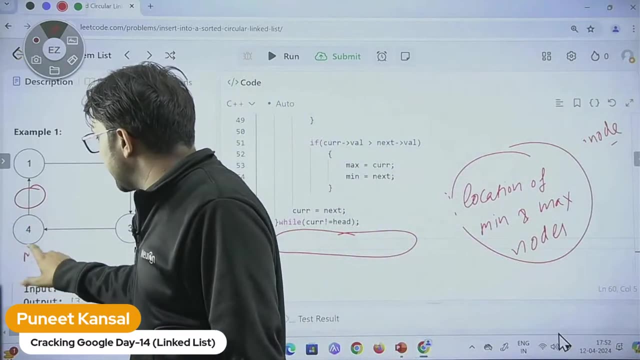 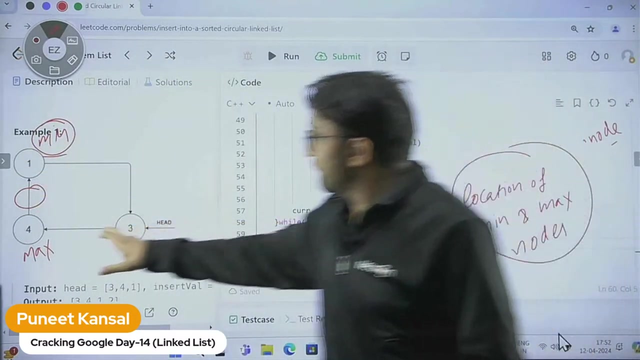 so i'm not writing this code now. can anyone please, anyone, can you? can you write the code? can you insert the node now here? let's suppose this is max and this is min. you know the location now. you know the address of max node. you know the address of min node. 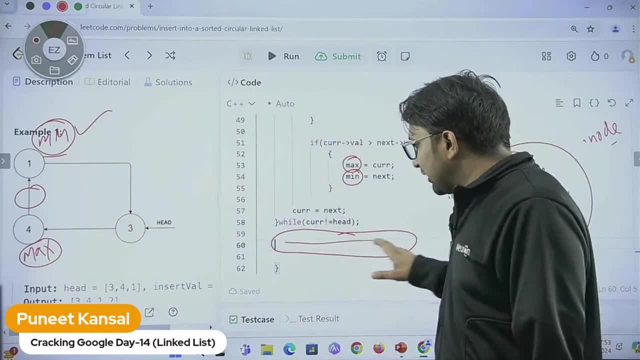 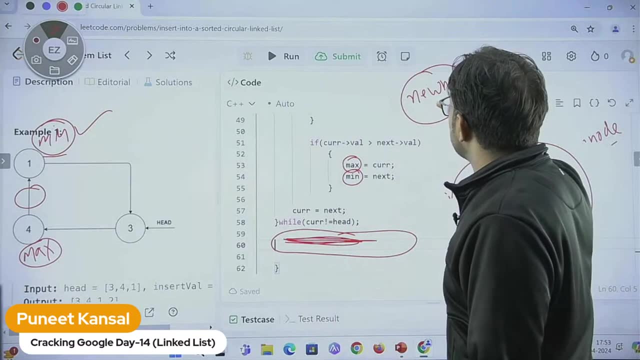 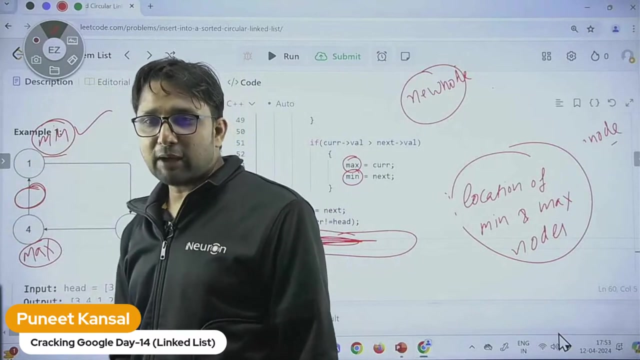 let's see if anybody can reply or not. can you write a code? after coming out of the loop, i want to insert my new node. i want to insert my new node in between here, in between max and min. i'm not writing this code. can you please write for me? anybody, anybody. i'm not. 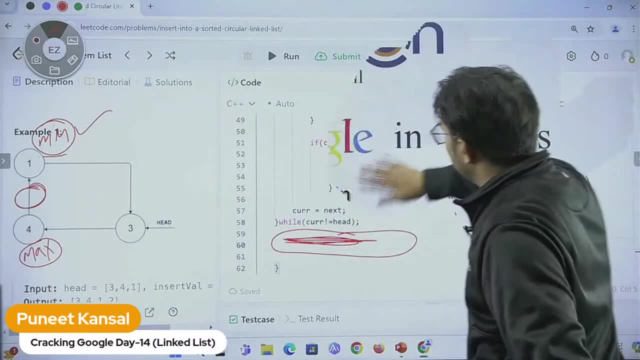 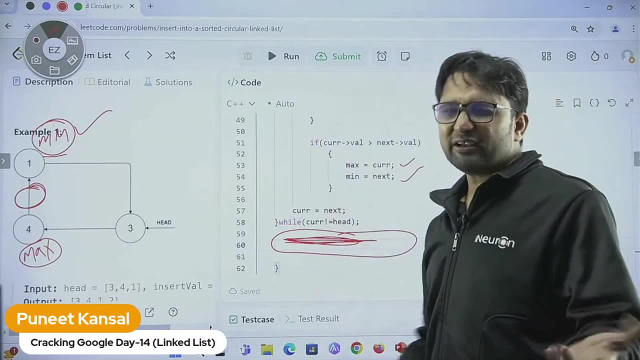 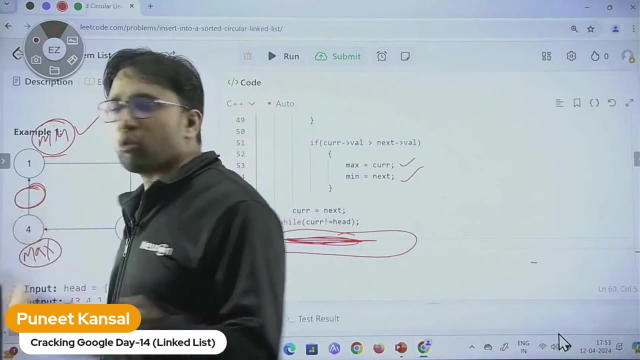 writing. please write. we know the address. we know the address of those two nodes. after coming out of the loop, one thing is confirmed: this is the only location where the element will be inserted now. there is no other, because already we check for all other condition. but after coming out of, 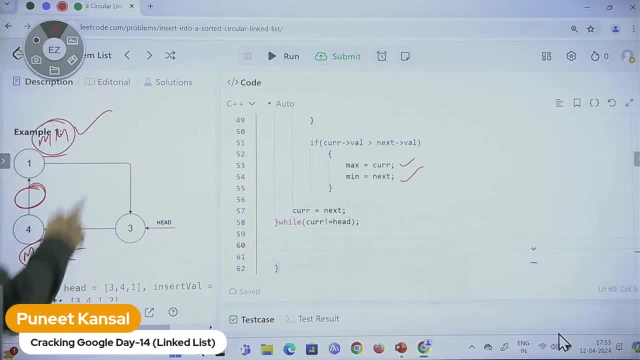 the loop we need to insert between max and min. anybody if can reply you want to insert it in between the nodes after coming out of the loop and then insert in between the nodes as well. please reply. okay, it might be that will. might take a little time. you can reply, i know. but okay, uh okay, i'm going at my end because i don't want to extend the lecture. so max, what i need is max byte 1. death total quantity: enter max to initial number: 13. max is max to initialAPN. cannot use min ip Schweet. 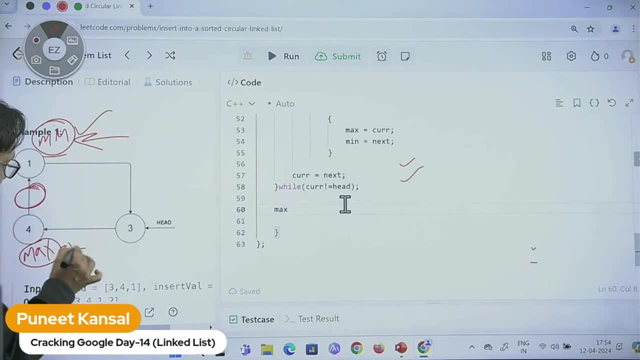 max to initial number 13 to insert. i need to insert at the next. let me write at the next: in the next, next of this node, we will insert new node, new node, fine, in the max next i will insert the new node and in the next of new node i will insert the min. i will insert the min, so new. 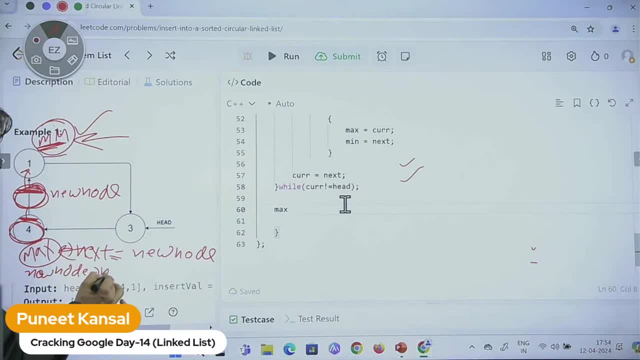 new node, new node. next will be min. that's it. that's it. so let me write the same code over here. and the max. next we will insert the new node and in the next, in the new new node. next new node. next we will insert the min- min node and after that 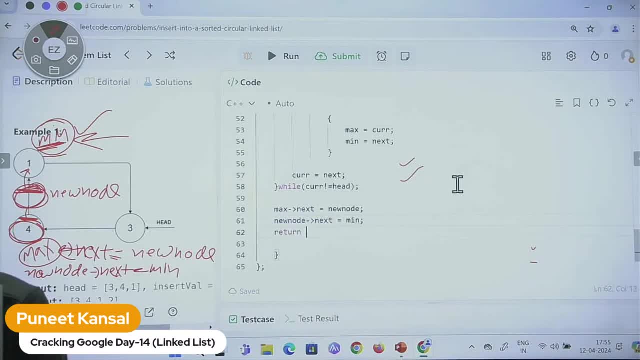 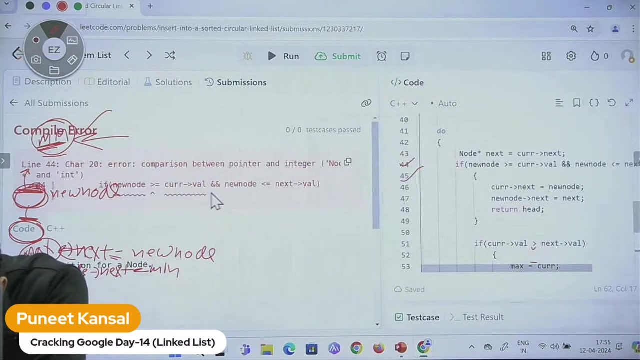 okay, if we are inserting again, we will return our head. we will return our head back. that's it done. done with this, done with this code. let me submit this. there is some error over here. let me check out 44 line, 44 line. i'm going to you people. 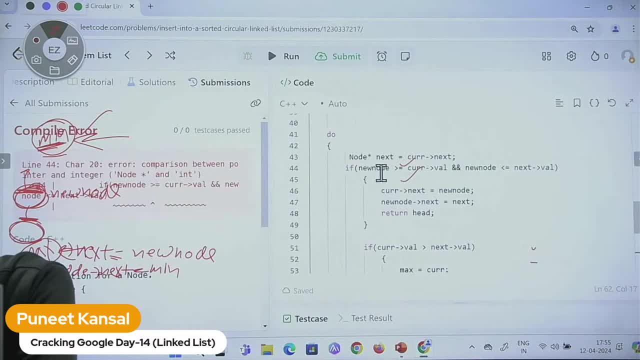 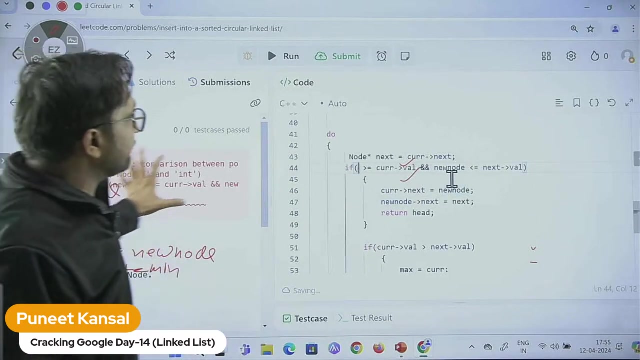 please help me. what is the problem with this? why this is creating the problem. so 44 line, 44 line- new node- new node will not come here: the the value. we are comparing with the value. okay, we are not comparing with the node, we are comparing with the value. so i just write the new node over. 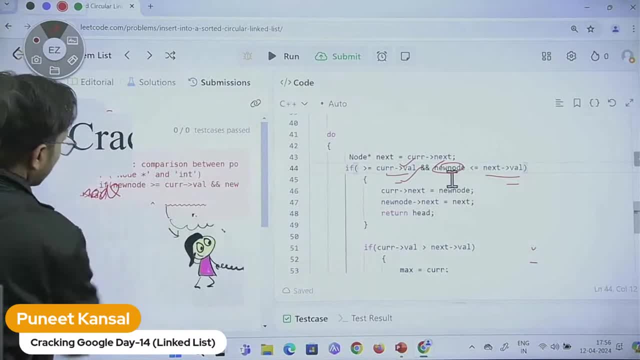 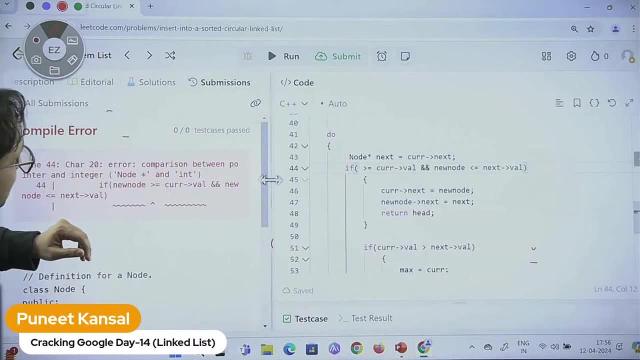 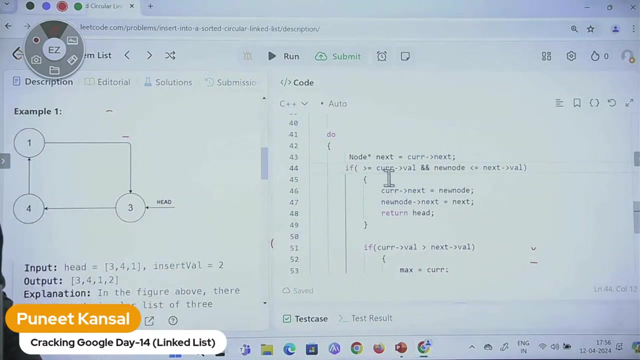 here. no, not new node. we need to write the value. we need to write the value. so the value was: but what was the name of the value? uh, the name of the value is. let me go to the description, that is, insert. well, insert, well, i need to write over here. I'm comparing with the insert value. 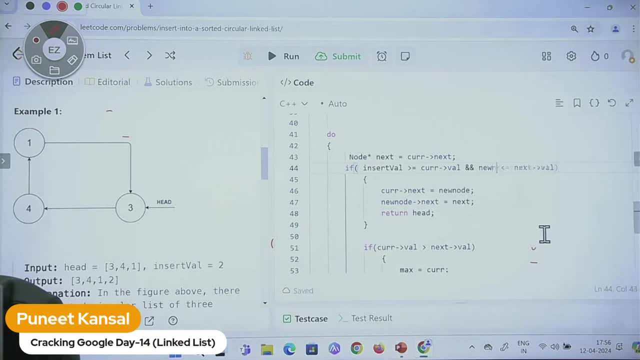 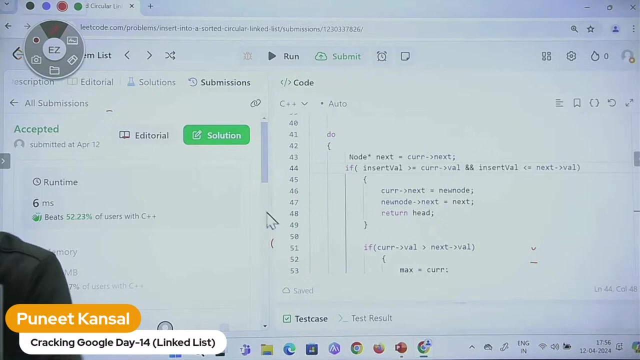 insert- well, not with the node, but its value insert. well, fine, let's submit it again and let's see: yeah, this is working fine, great, great. so, yes, this code is working fine, simply what we do: create it once again. wanted to write return and then something going over. here we are doing. 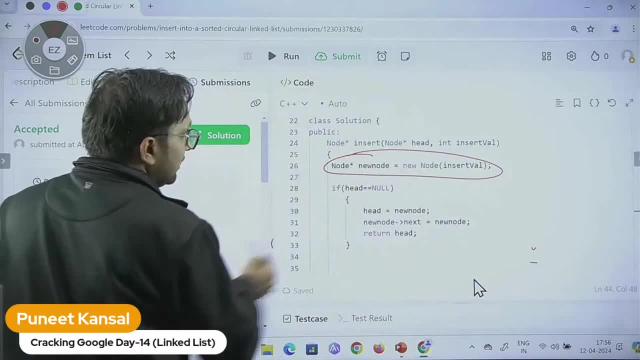 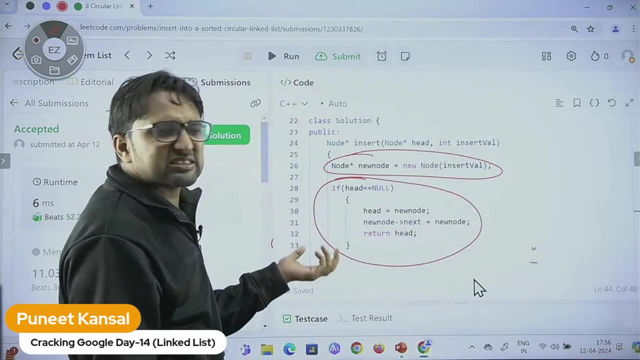 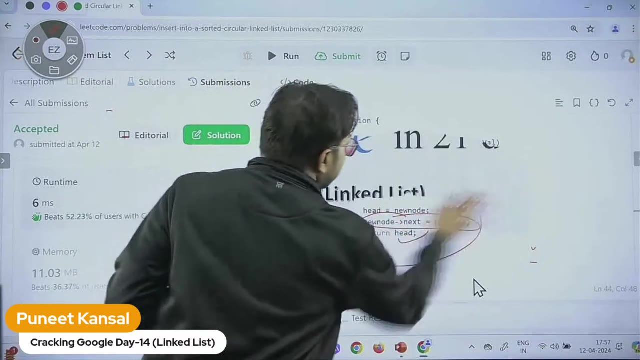 return and we are taking the first color, we are taking the second and we are entering it for governments. i am going to basically build it here. our new node, fine, this is: this code is for the empty link list. if the link list is empty, then just simply make our single node as a circular and return the head. that's it so, till this place. 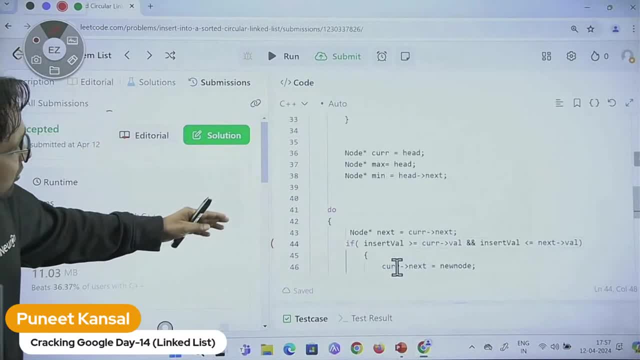 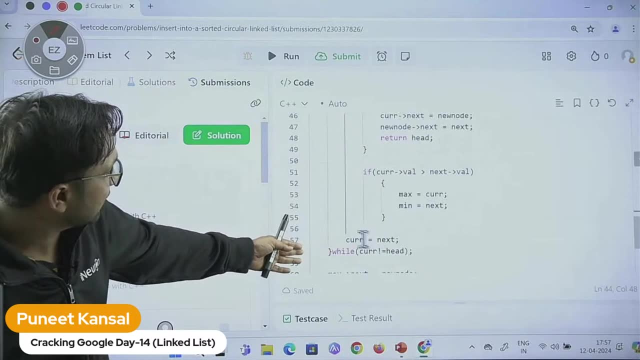 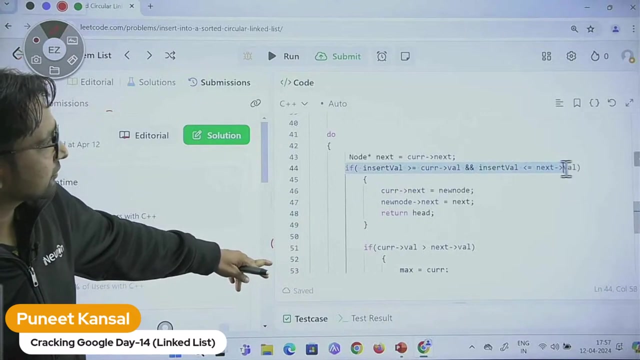 we're done and after that we just take a current and next two pointer, which will keep moving until what? until our current is not become head, and what we are doing? just simply checking this condition. if this condition satisfy, we insert the node between current and next and we return. 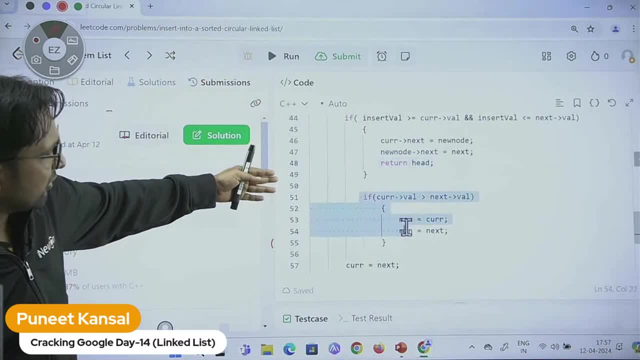 the head, otherwise one more thing we are doing. we find here this cut, this is finding the location of max and minimum element, max and minimum element node and after coming out of the loop we are just starting to find the current and next we return the head, otherwise one more thing we are doing. we 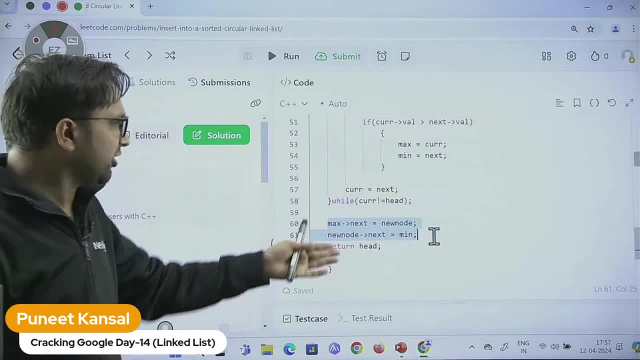 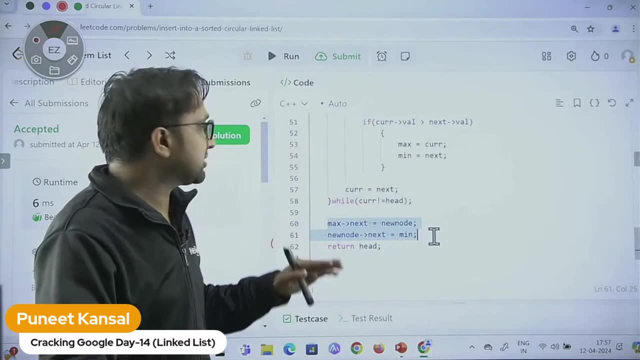 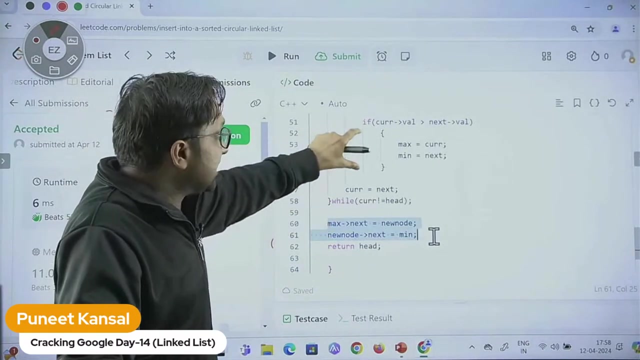 are storing the element between max and minimum, why we are doing this thing. this is the only thing. i believe that in this question, which is uh little, we need to think over. otherwise there is not much in this question. this is the only thing. uh, we are handling this edge case. we are. 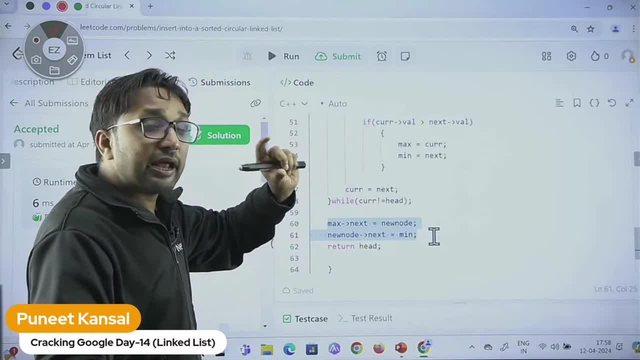 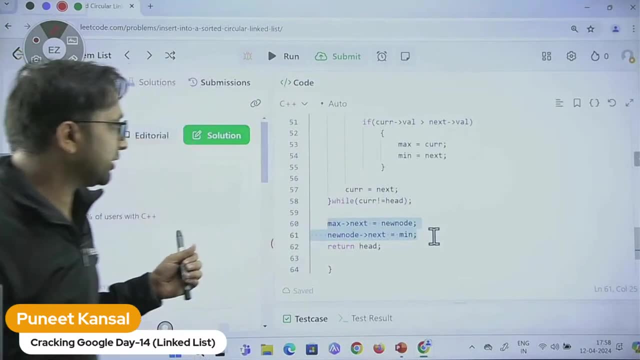 handling this edge case that if the value is lying between maximum and minimum in the linked list, then how you will handle that, that that is the only part actually you can say little difficult over here, otherwise link from linked list point of view this was really very easy. 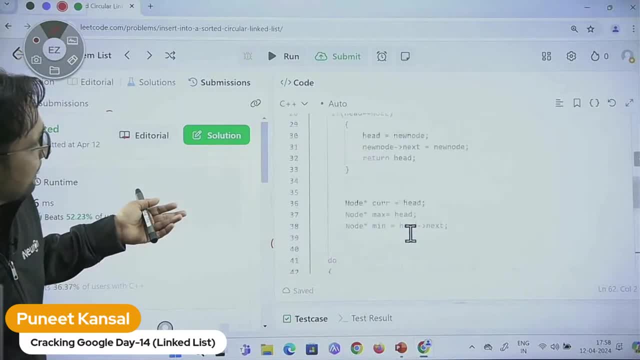 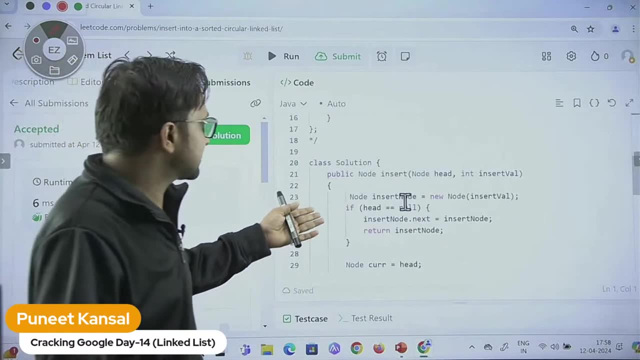 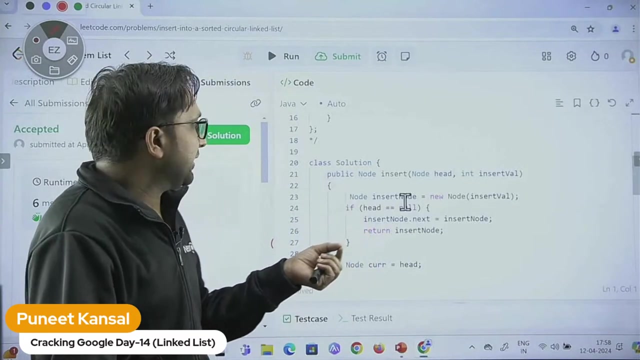 so that's it. after that we return the head and if we check out the code in java, that is the same code itself almost in java and c plus plus in linked list. the main difference is in java we use the dot operator and in linked list we in c plus plus we use the arrow operator to access the value. 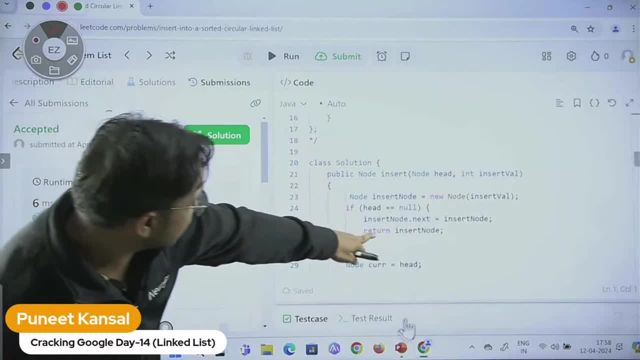 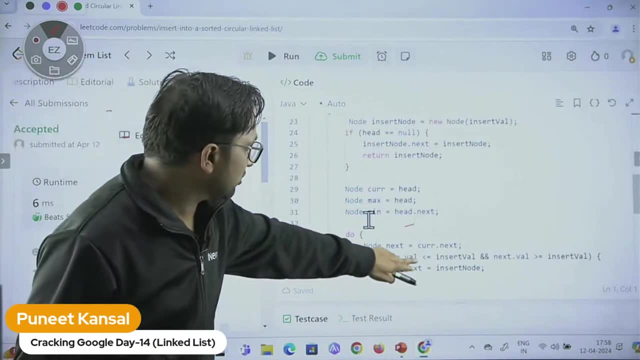 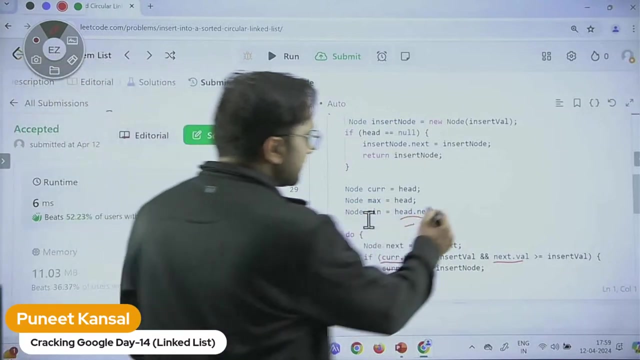 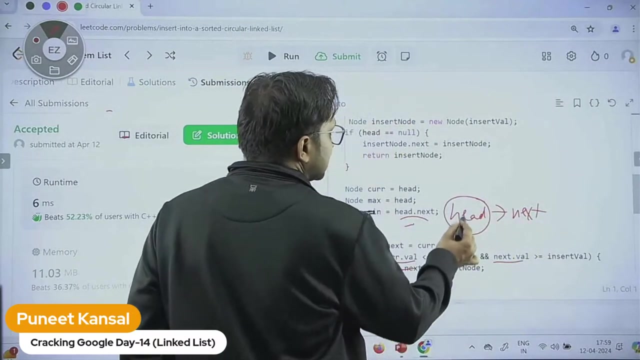 or then next address. so here you can see, every time i'm using dot dot, every time whenever i'm accessing next or or any value, i'm using dot dot. so this is the only difference: dot, head, dot. next in c plus plus, we write head arrow operator next actually in c plus plus. uh, this head is up is a pointer. 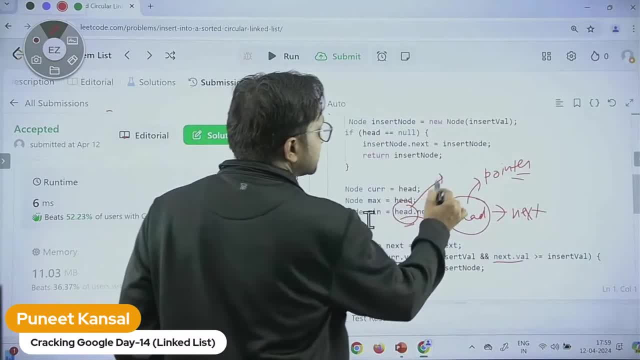 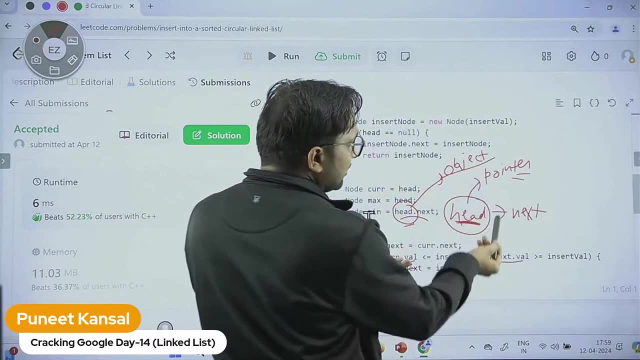 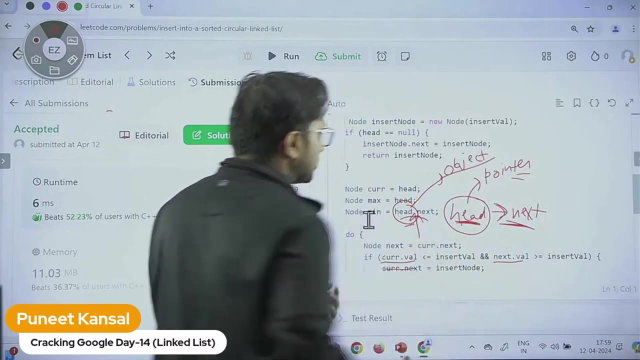 okay, and in java this is a object, this is a object of a class and this is a. this is a pointer and pointer: use the arrow operator to access the element at particular location. object for object, we use the dot operator. so this is that only difference. one more. 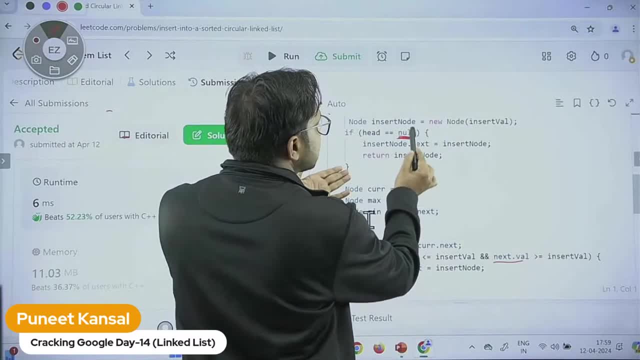 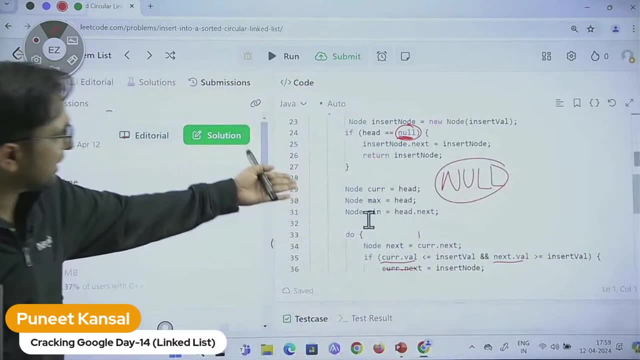 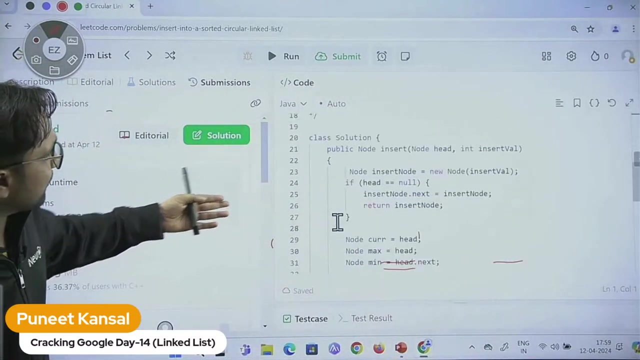 difference is there? okay, little bit. in the java there is a we in the small letter. we write null in c plus plus we write null in capital. that's it. otherwise the code is completely same. you can check out. important part is the logic, what we doing here, what we are doing over here. simple: we created a. 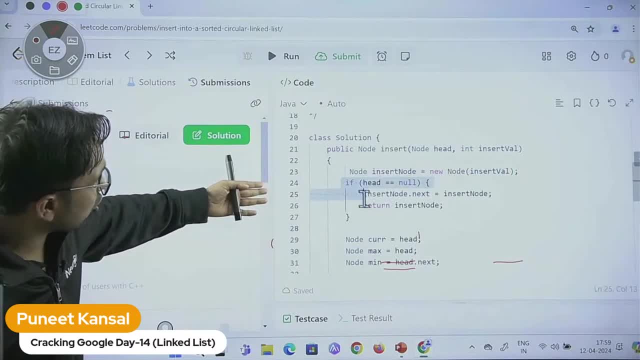 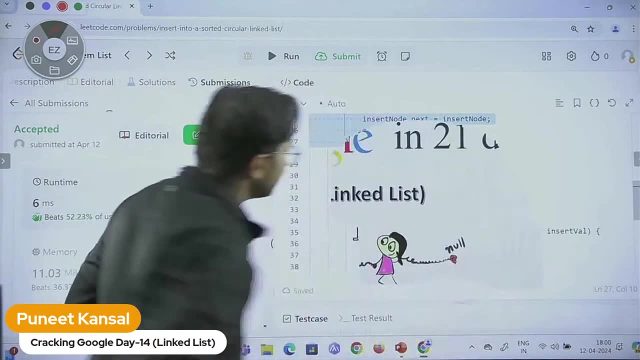 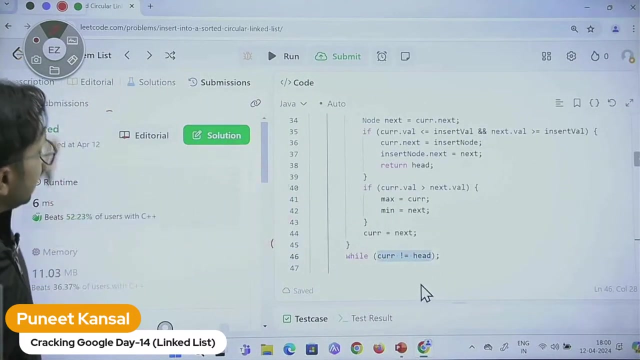 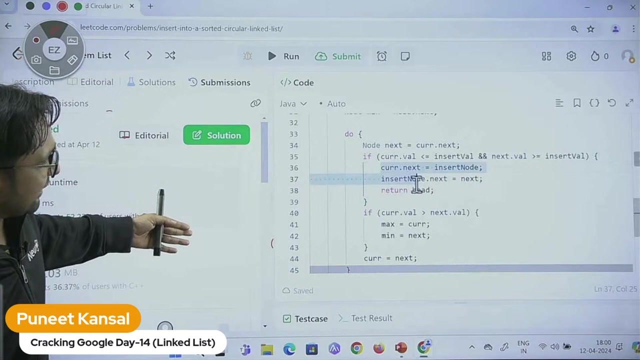 new node. fine, we are inserting a node into empty linked list. fine, after that, after that, we are just going through. we are going through the, we are going through the linked list and if this condition satisfy, then we insert the node and return our result. we are finding the location of min and max. 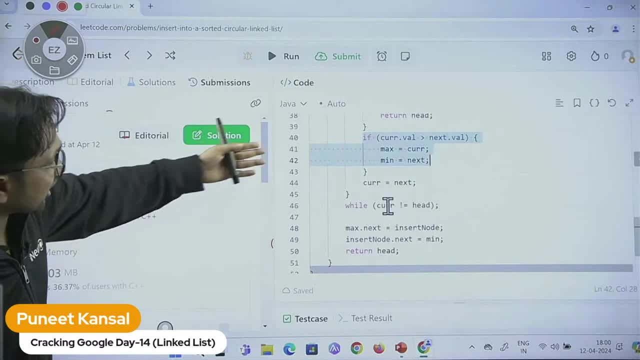 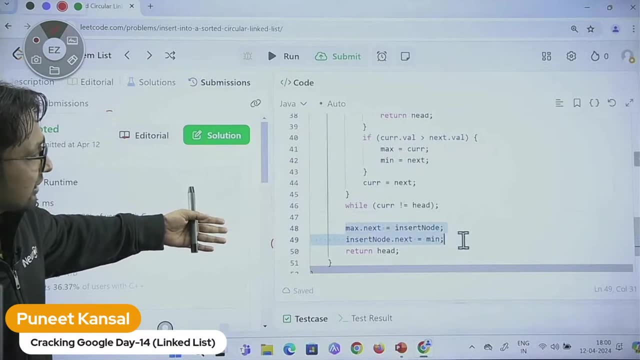 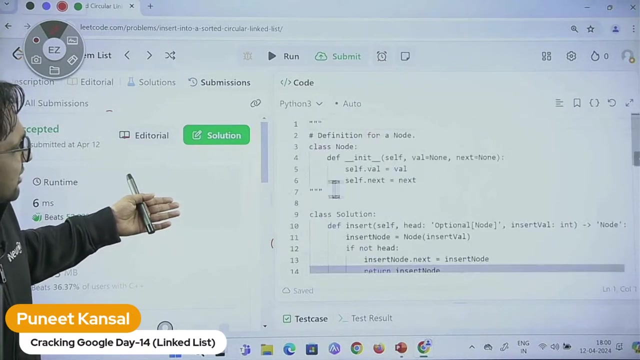 if out, after coming out of this loop, if we are coming out of the out of this loop, then the only location left is between max and min. we insert the new node and return the head. that's it. and we if we check out the java, so python solution, that is same new node is created and this is for. 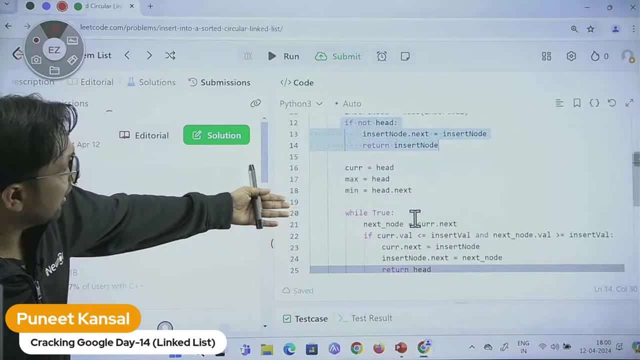 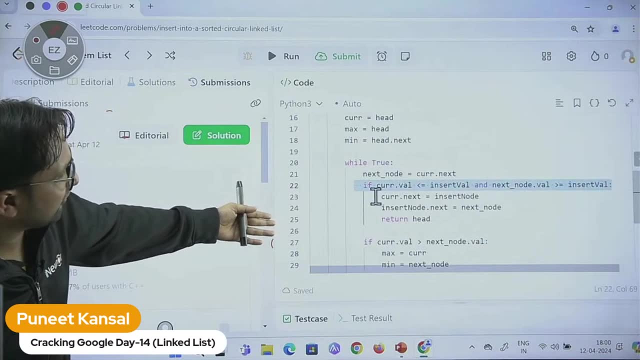 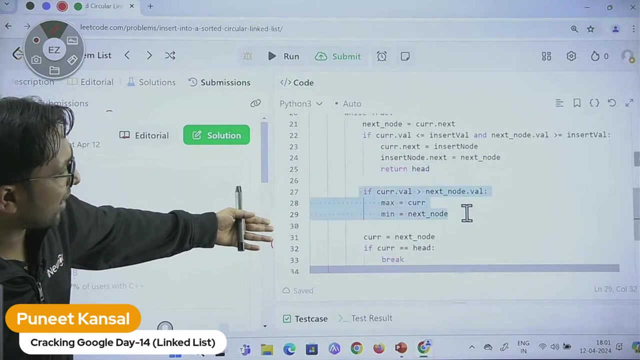 the empty linked list, again the same. and here we are. this until this condition is satisfy, we will. if this condition condition satisfy, we will insert the node and return the head. here we are finding the location of max and minimum node. after coming out out of the loop, we 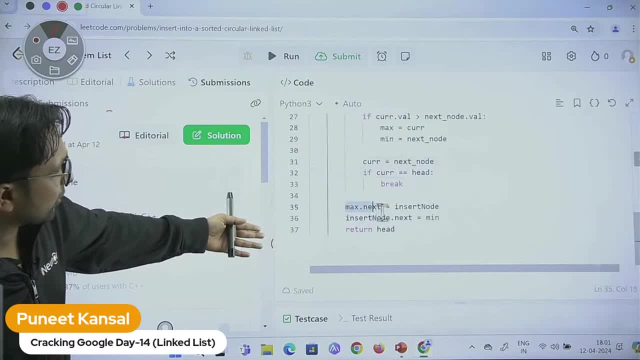 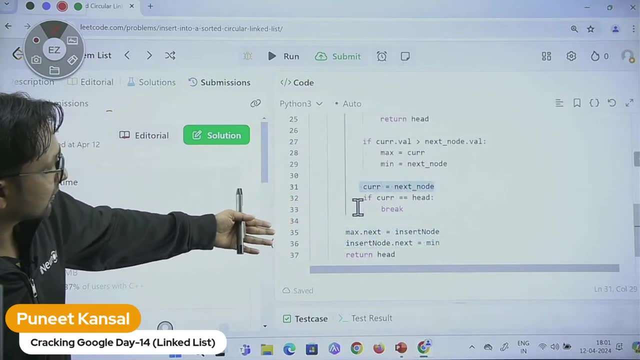 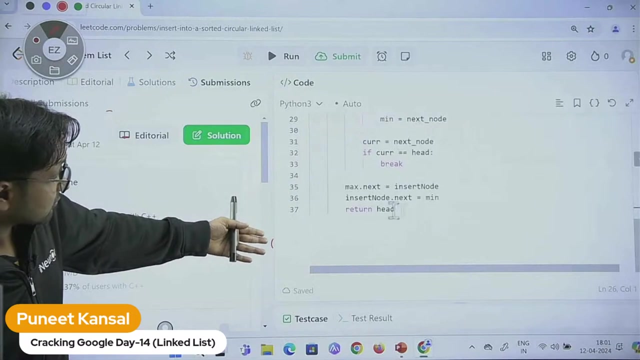 are inserting after coming out of the loop. here we are inserting the, the node between min and max. here we are updating our current, okay, and if, if the current reads to the head, we break. so this loop is going on same thing. everything is same, logic is same, just. 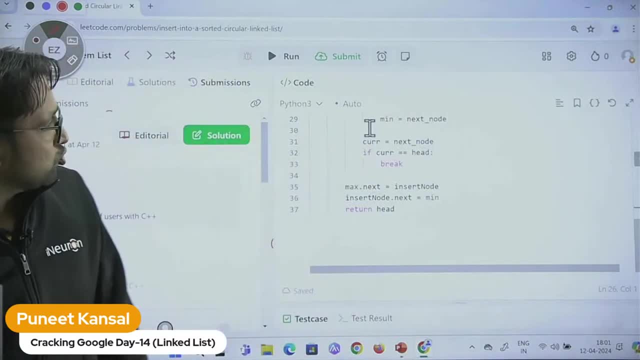 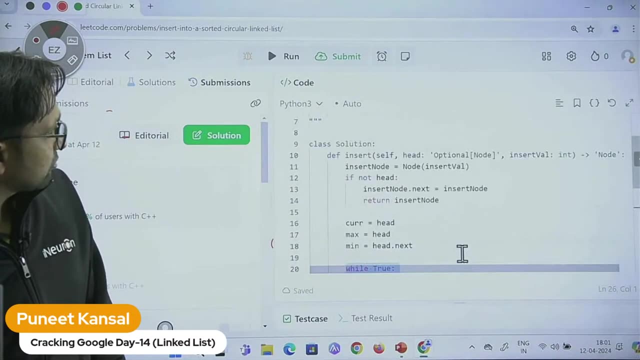 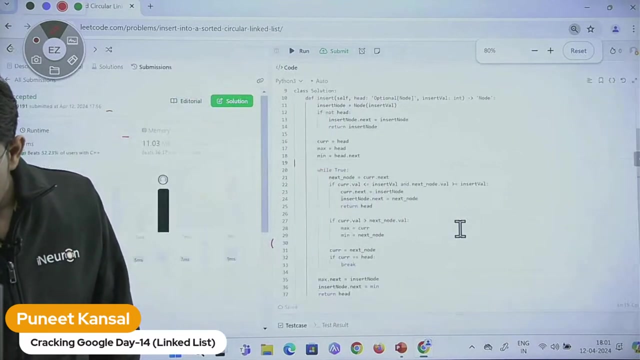 the syntax is different. so whatever language in which you want to see, you can refer that language. fine, okay, let me reduce the size also so that this comes to one single screen. so, yes, this is the complete code for the python now. this comes now in the single screen. 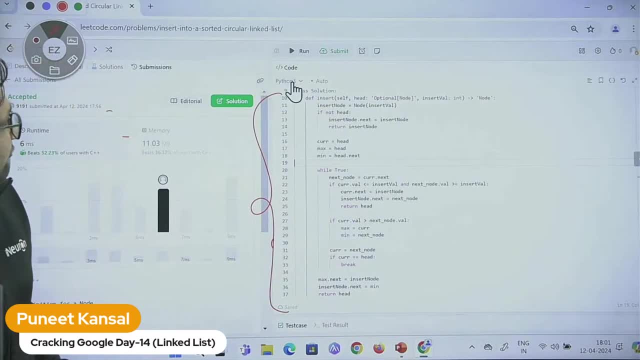 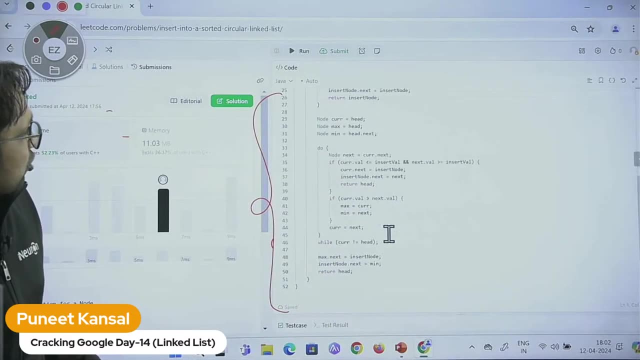 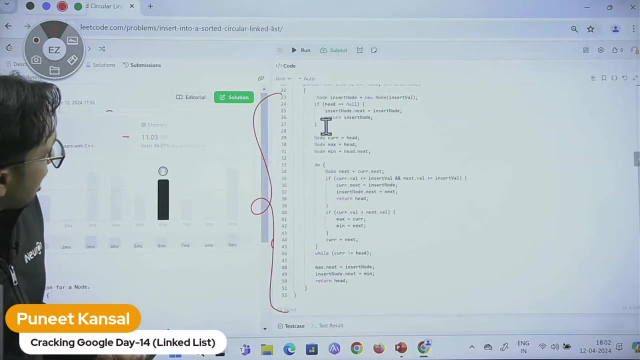 you can check out easily. and if we go to java, let me bring the code into single screen. so here is the code into single screen. now let me reduce little bit more, make it down. yes, this is the complete code to my path to myPoint. I type into: 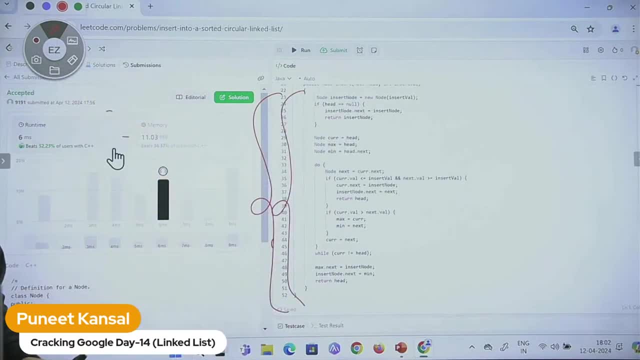 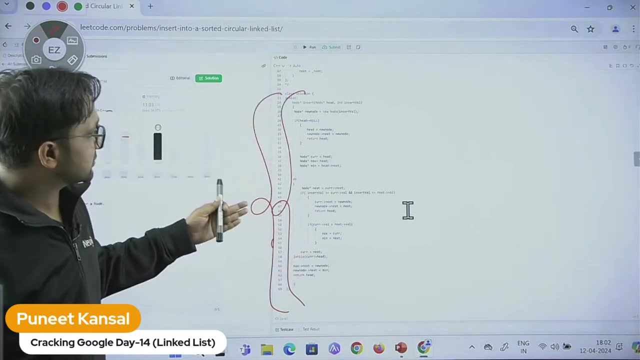 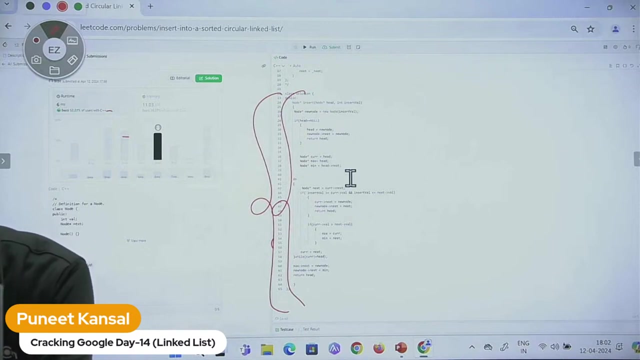 code in java and let me show for the c++ also. so, yes, this is the complete code. let me reduce little bit more. yes, now this is the complete code in c++ in one screen. fine, okay, let me go through your questions now, whatever questions you have, like ayush is asking: sir, is there? 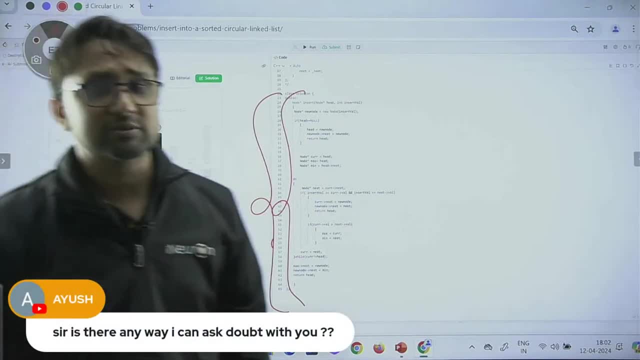 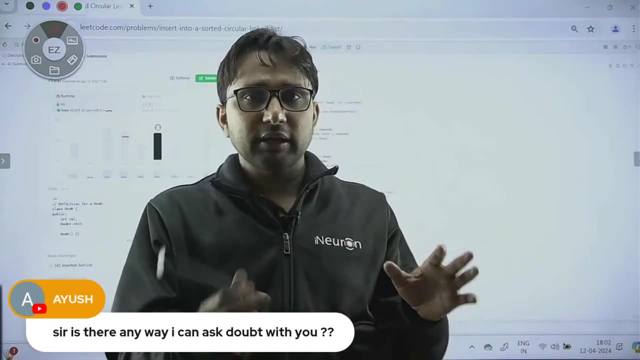 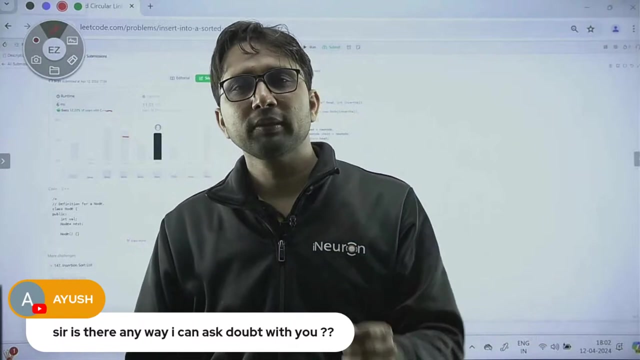 any way, i can ask the doubt with you. yes, ayush, you can ask me the doubt. you can ask me the doubt in the comment section. so go to the. you go to that particular video and write whatever doubt you have related to this lecture. you can ask me over there, even though 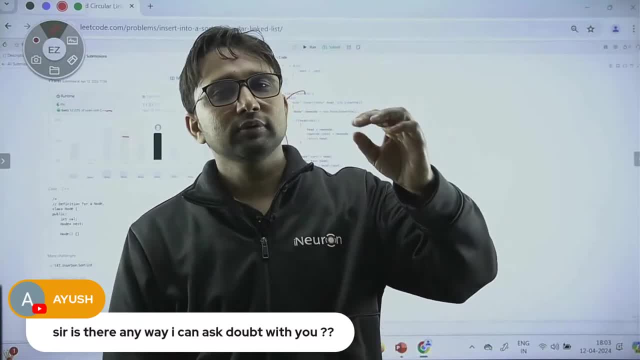 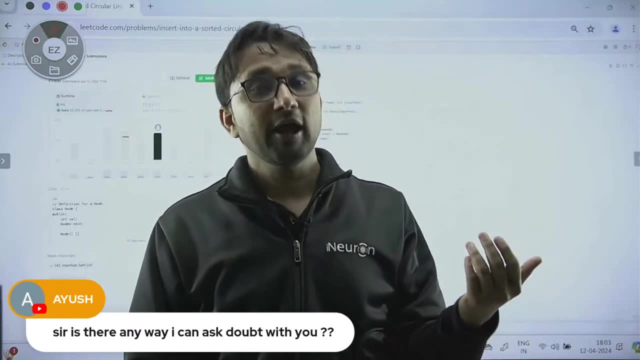 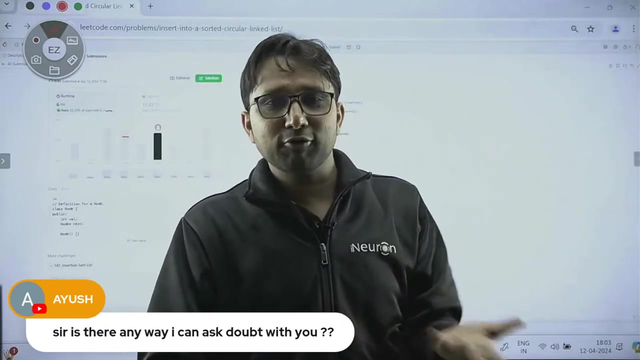 if you have any doubt related to the dsa itself- general doubt also- you can ask in the comment. i will definitely reply over there and if i don't reply you come to the next lecture. you can ask me. sir, i commented in that lecture but you don't reply. i cannot run away means. 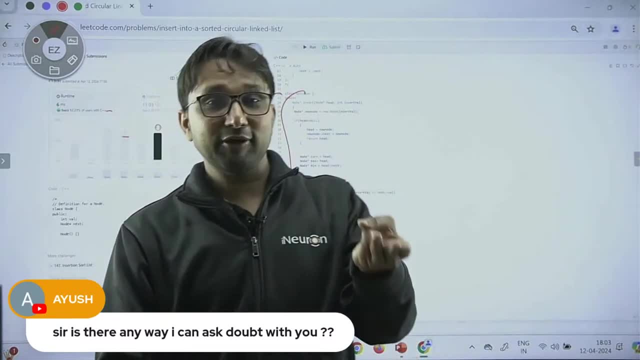 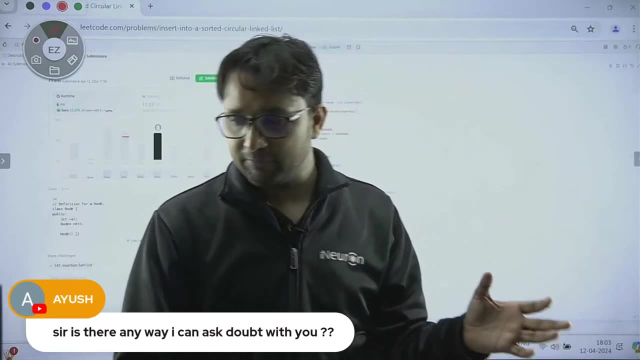 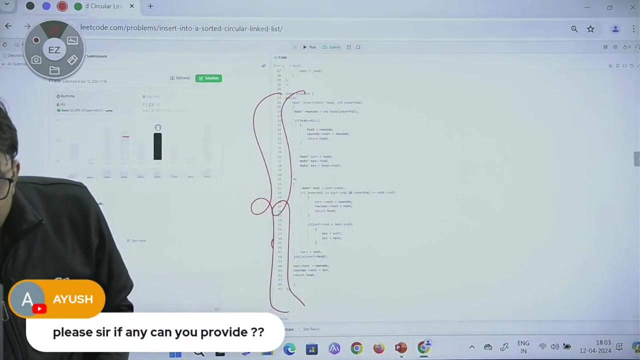 i am coming live. only every three days in a week i am coming live, so i cannot run away. you can write your question in the comment section. okay, i will definitely reply. there is one more thing, sir. please, sir, if you can any, if any can you provide? 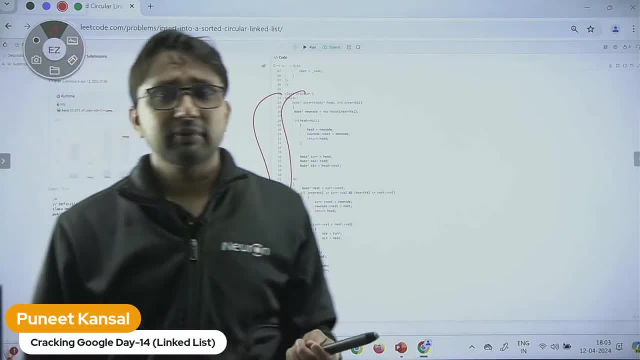 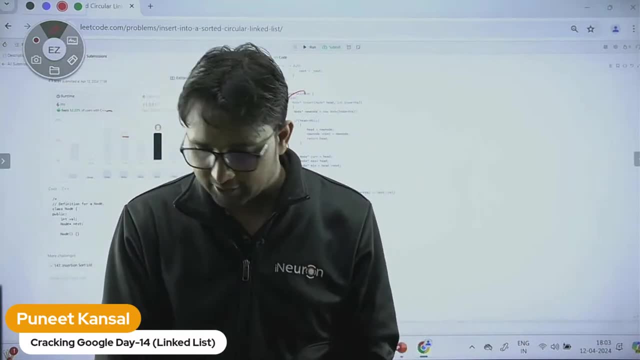 so you can means reply over there. just you can write the com in the comment. whatever is the question coming to your mind related to dsa, you can please reply over there. i will definitely reply in the comment. fine, okay, i hope you get the idea how many people get. 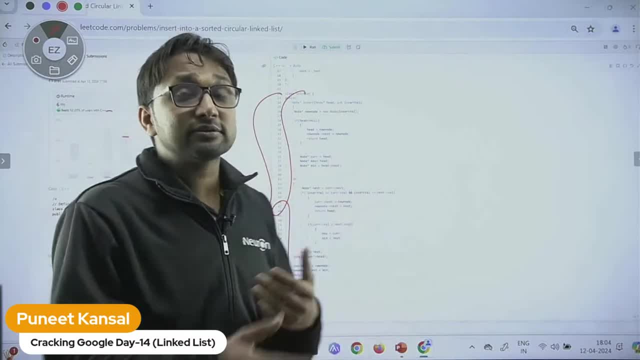 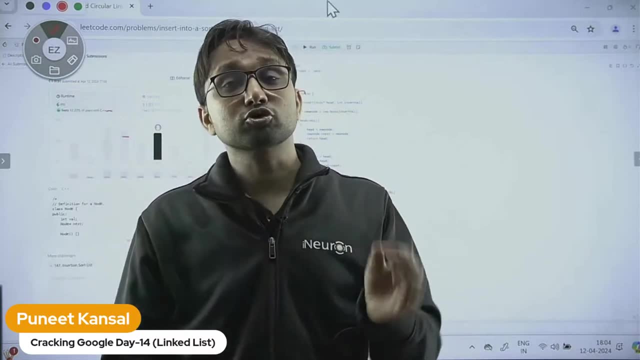 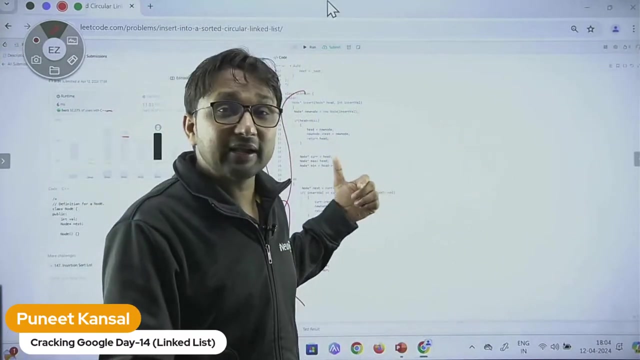 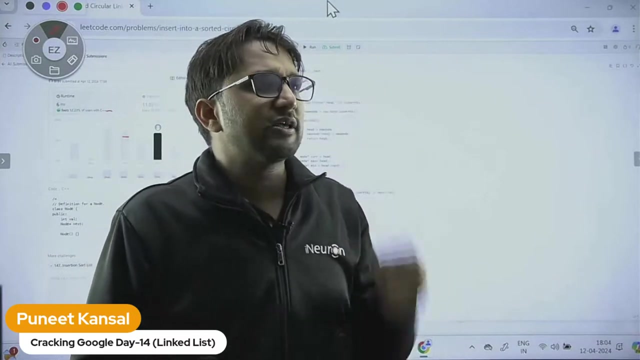 this today's question. so we are covering- see might be today we cover one question, but the complete series. you are covering 21 questions from different, different topics, different, different topics every day. you are solving one quality question. that is really means you are solving google question. that will really definitely that would make make the impact, the only difference. 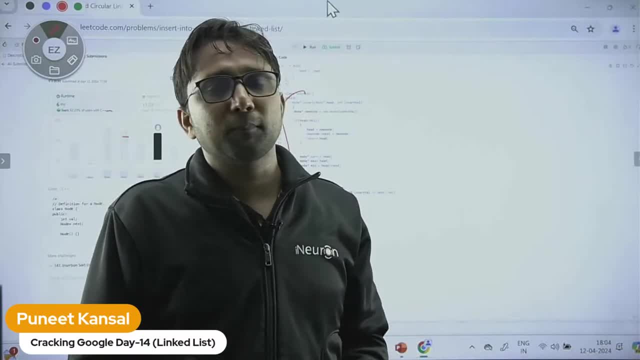 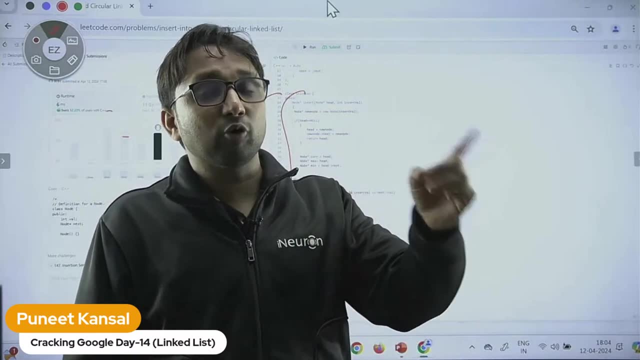 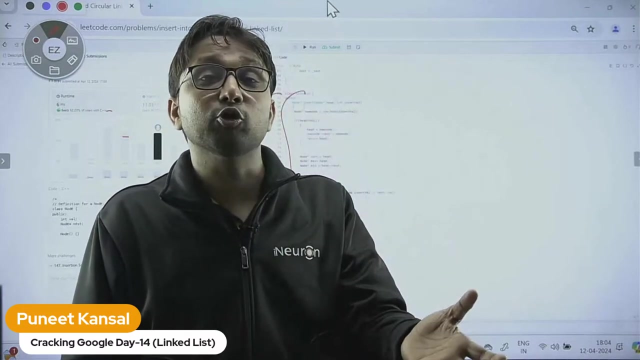 between the people who crack the product based company and who do not crack. what is the difference? if you are thinking that they do not have logical thinking skill, actually you are fool. everybody have logical thinking skill. we are human being. then what is the difference between me and them? 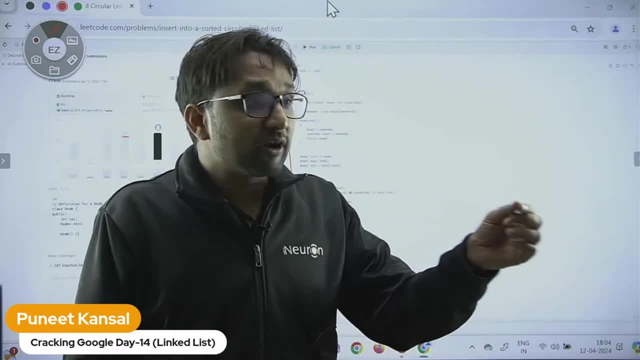 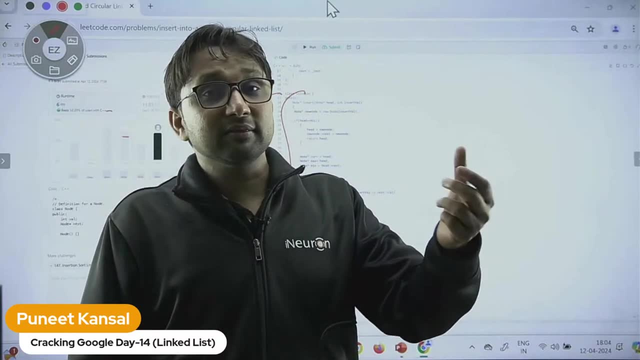 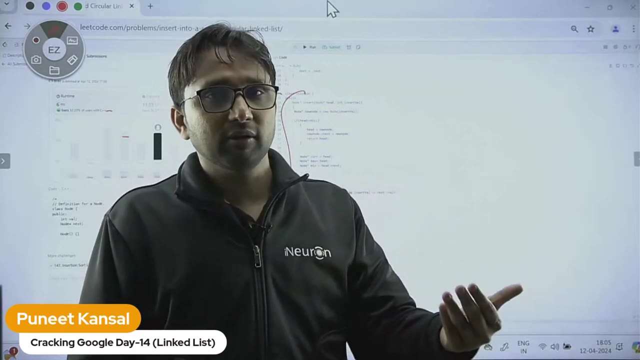 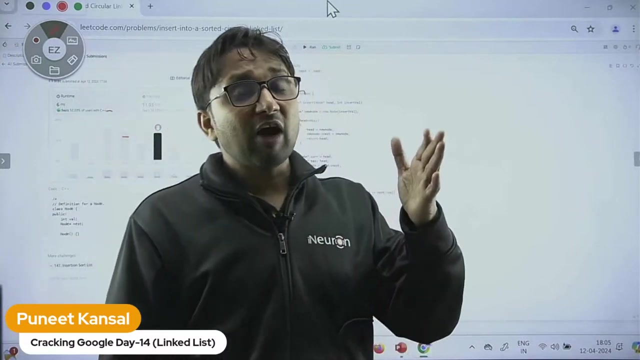 only difference is that who is working consistently, who is daily solving the problem and who is not solving the problem- and this is easy to say for me, but really very hard to follow. to work daily, to work daily. so be consistent and please solve the problems, definitely after. 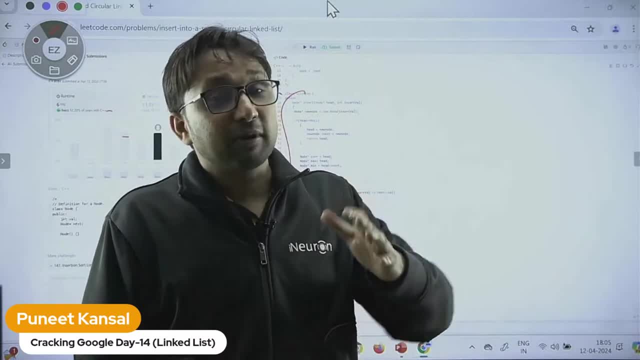 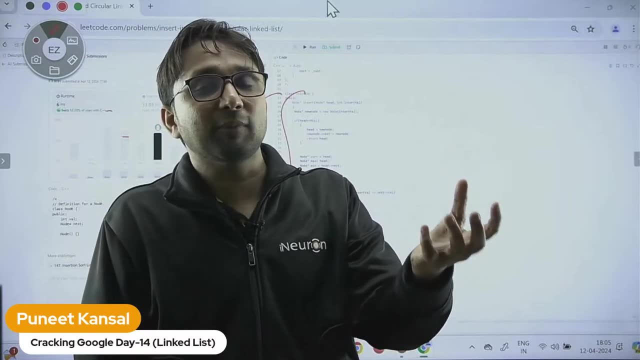 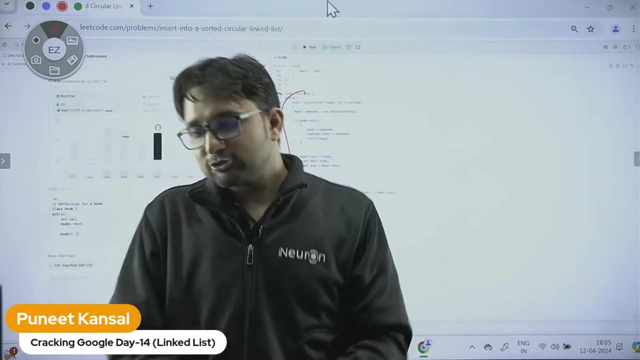 six months you will find out the results. so, but that is a long, long time. i'm sure i know this thing and this is the only difference between the people who are reaching over there who are not reaching. it's not about any other thing. okay, so i hope you find this session helpful. if you find this session helpful, please write in the. 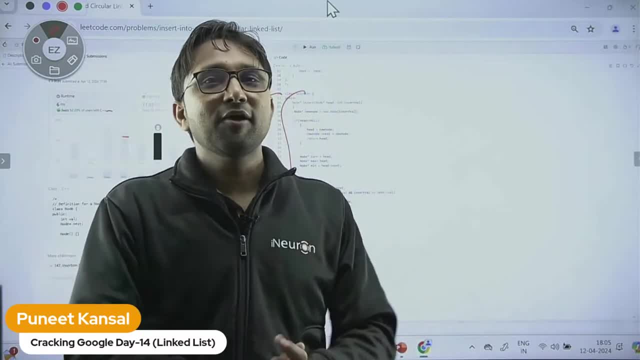 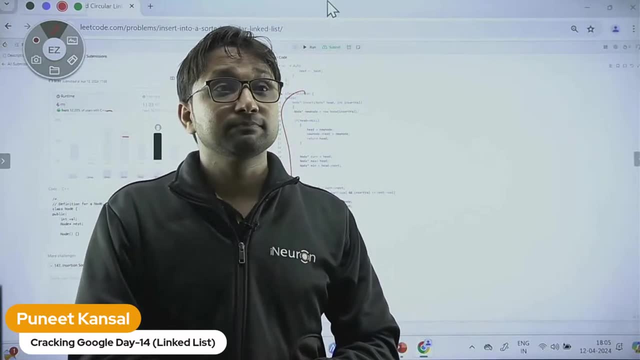 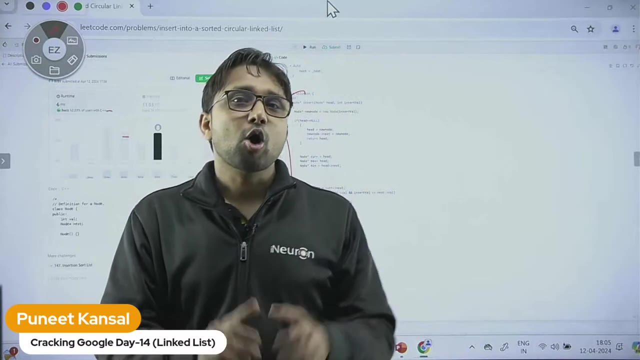 comment section after this session and give a thumbs up, and tomorrow also you can join our new one. another session: i'm coming up with the podcast with the shagun. she is working in amazon. she will share her experience, how she cracked the amazon. so i will see you people over there.